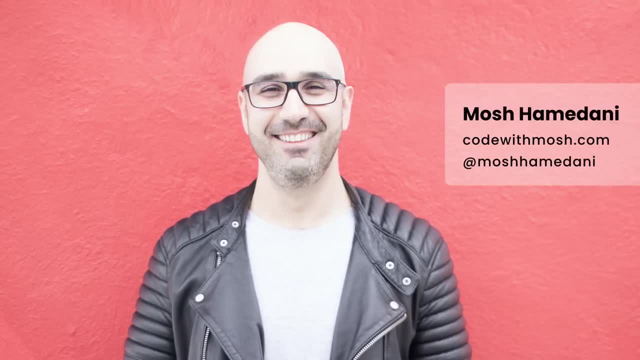 to advanced concepts. I'm Mosh Hamadani and I'm super excited to be your instructor. If you're new here, be sure to subscribe, as I upload new tutorials every week. Now let's jump in and get started. So what is Git and why is it so popular? 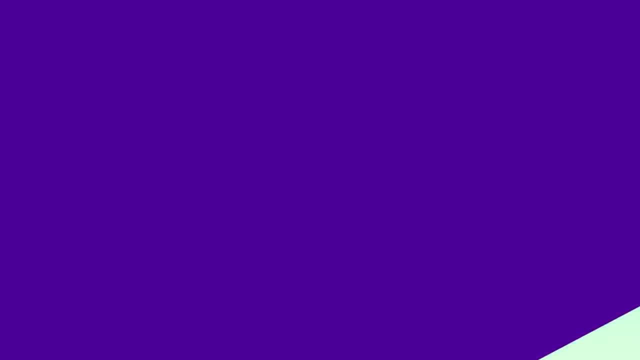 Git is the most popular version control system in the world. A version control system records the changes made to our code over time in a special database called repository. We can look at our project history and see who has made what changes, when and why, And if we screw. 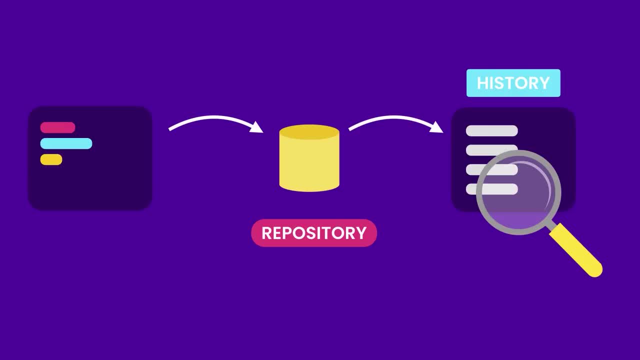 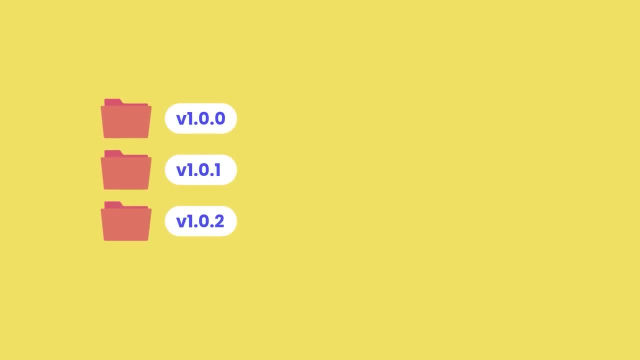 something up, we can easily revert our project back to an earlier state. Without a version control system, we'll have to constantly store copies of the entire project in various folders. This is very slow and doesn't scale at all, especially if multiple people have to work on the same project. We will have to constantly. 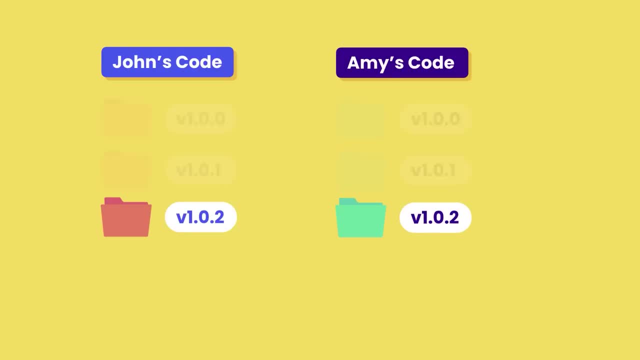 toss around the latest code via email or some other mechanisms and then manually merge the changes. So in a nutshell, with a version control system, we can track our project history and work together. Now version control systems fall into two categories: centralized and distributed. 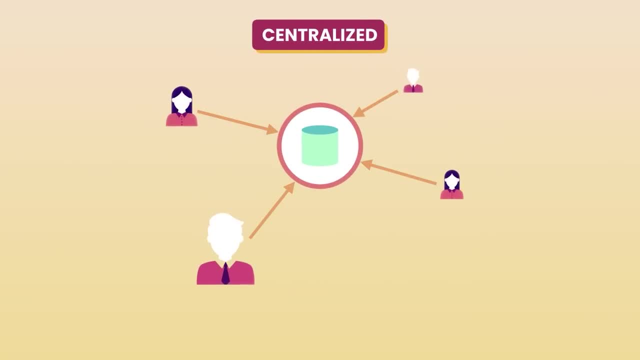 In a centralized system, all team members connect to a central server to get the latest copy of the code and to share their changes with others. Subversion and Microsoft Team Foundation Server are examples of centralized version control systems. The problem with a centralized architecture is the single point of failure If the server goes offline. 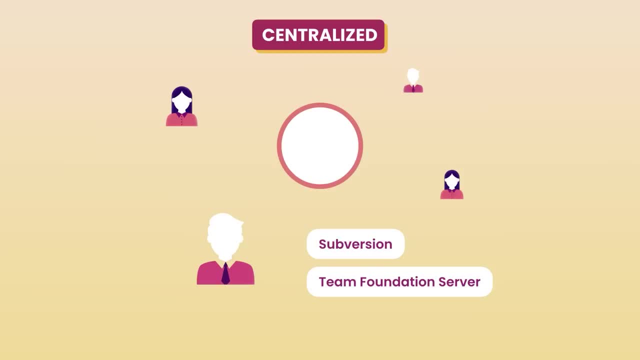 we cannot collaborate or save snapshots of our project, so we have to wait until the server comes back online. In distributed systems we don't have these problems. Every team member has a copy of the project with its history on their machine, So we can save snapshots of our project locally on our machine. If the central server is offline, we can synchronize our work directly with others. 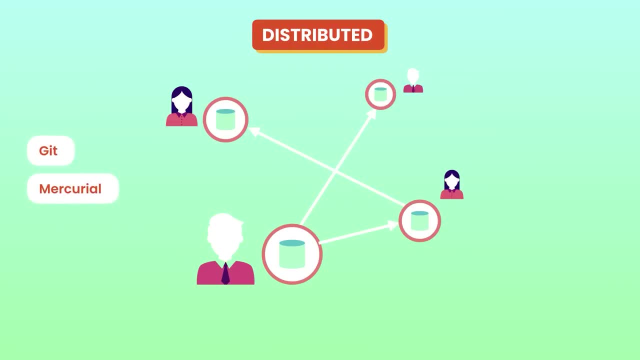 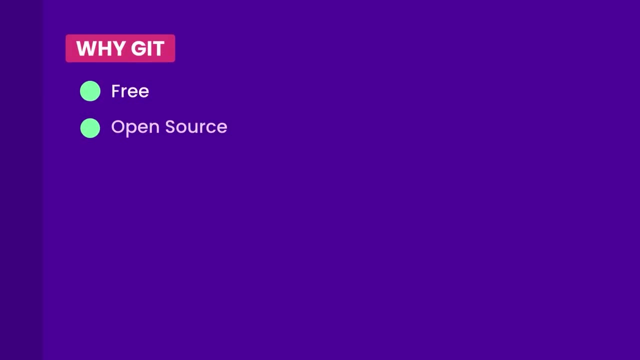 Git and Mercurial are examples of distributed version control systems. Out of all these, Git is the most popular version control system in the world because it's free, open source, super fast and scalable. Operations like branching and merging are slow and painful in other version control systems like Subversion or TFS. 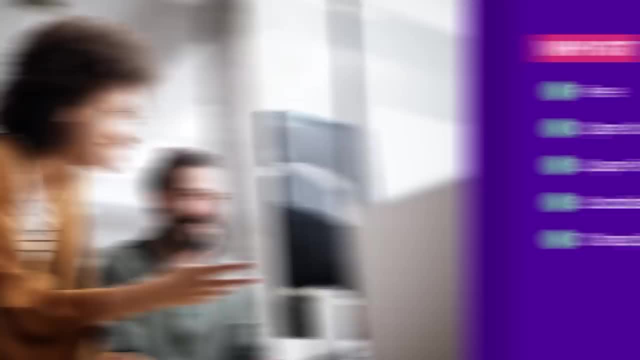 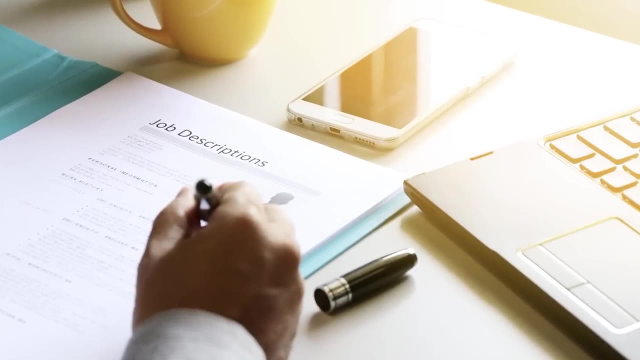 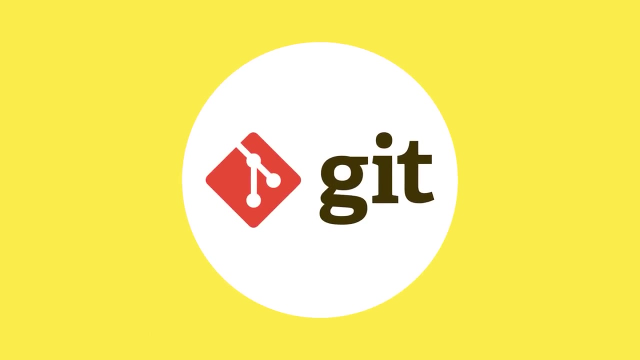 But they're very fast in Git. We'll talk about this later. So Git is almost everywhere. More than 90% of software projects in the world use Git. That's why almost every job description for a software developer mentions Git. So if you're looking for a job as a software developer, Git is one of the skills you must have on your resume. 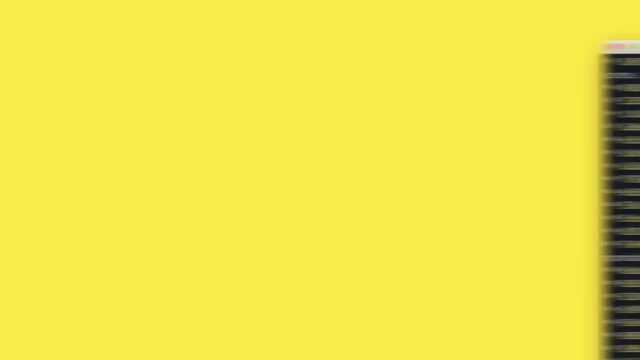 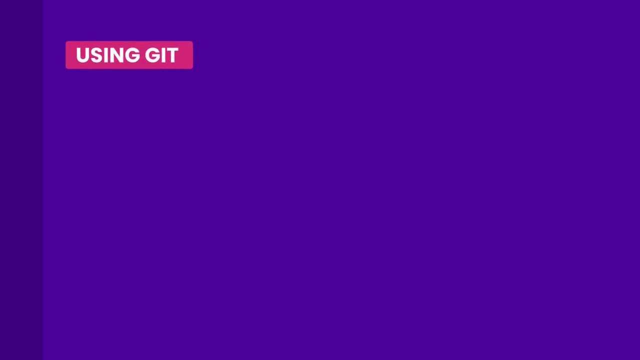 You should know it inside out. you should know how it works and how to use it to track your project history and collect data, And that's exactly what you're going to learn in this course. Let's talk about various ways to use Git. 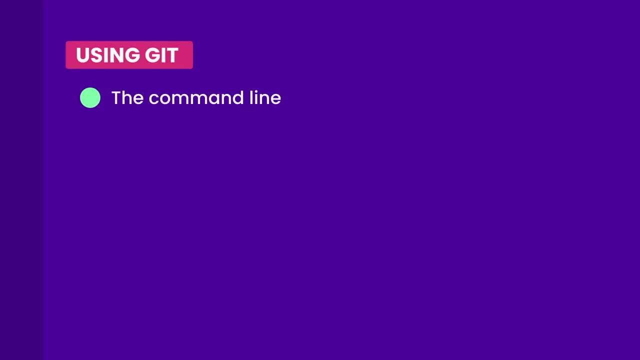 We can use Git on the command line, So we open a terminal or command prompt window to execute Git commands. This is the fastest and sometimes the easiest way to get the job done. That's why a lot of people use the command line. 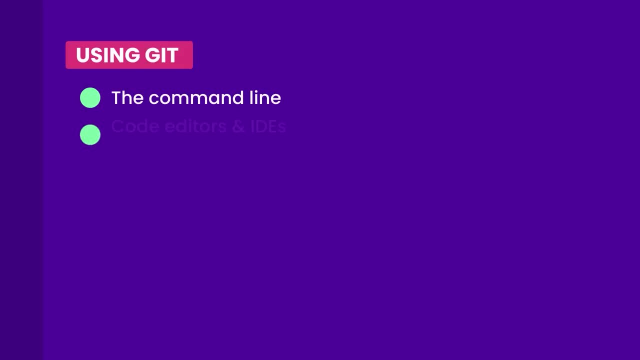 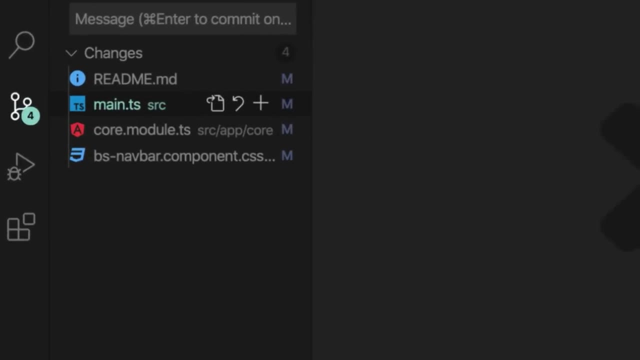 Now, if you don't like the command line, well, you're in luck, Because most modern coding systems don't have a command line. They're just built to support basic Git features. For example, in VS Code, we have this source control panel which gives us the essential Git features. 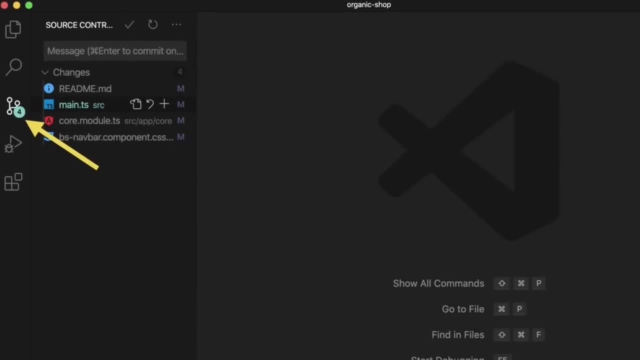 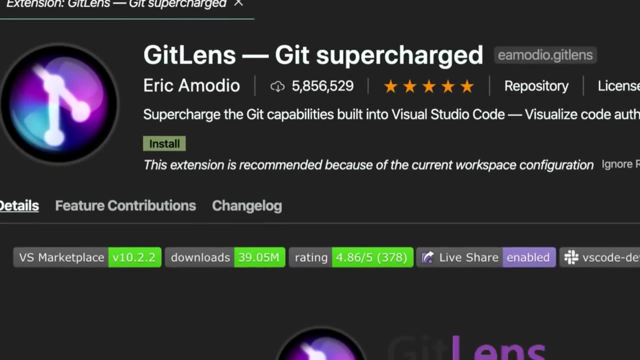 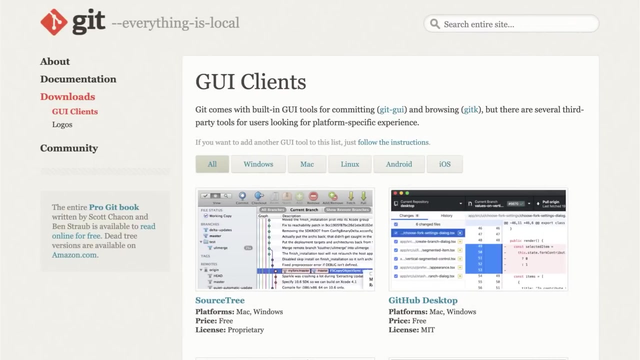 There are also extensions available for bringing additional Git features For VS Code. the most popular extension is Git Lens. It brings a ton of Git features in VS Code. There are also graphical user interfaces specifically made for using Git. Here on the Git website, you can find the complete list of these tools for different platforms. 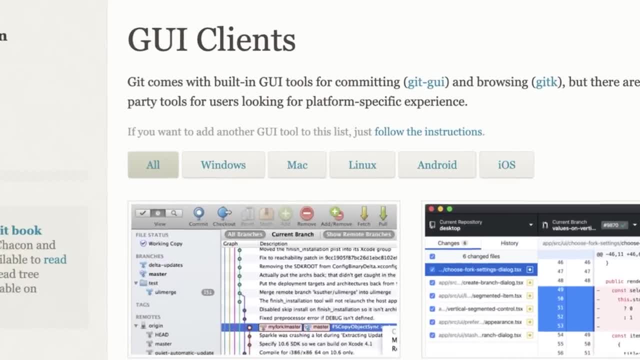 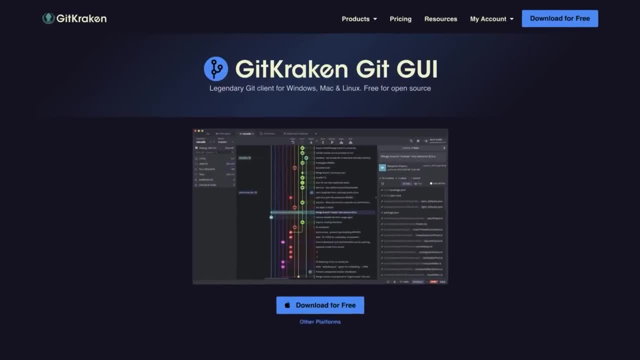 We have tools for Windows, for Windows 10, and for Windows 11.. We have tools for Windows, Mac, Linux, Android and iOS. Out of all these, the two most popular tools are GitKraken and SourceTree. GitKraken is my personal favorite GUI tool for Git. 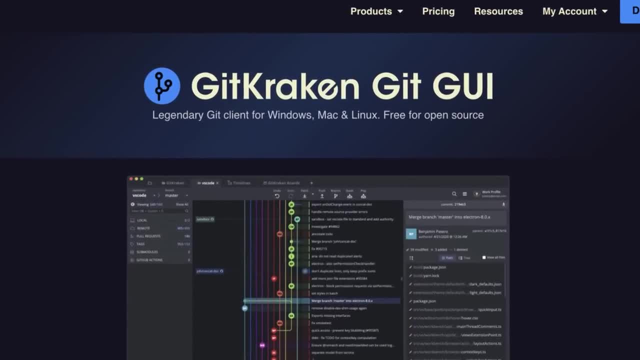 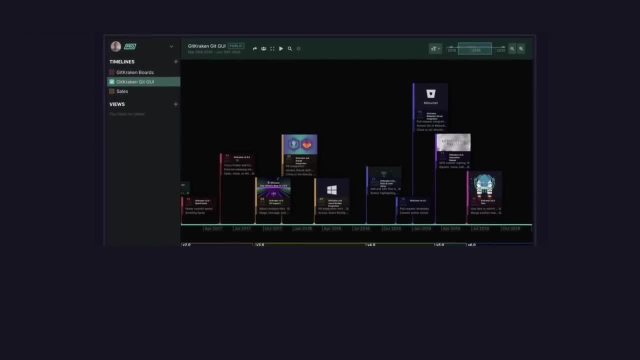 It's beautifully designed, it works across different platforms and it integrates with other GitKraken products, such as GitKraken boards for issue tracking and GitKraken timelines for project management. It's free for open source projects, but for commercial projects you have to pay an annual fee. 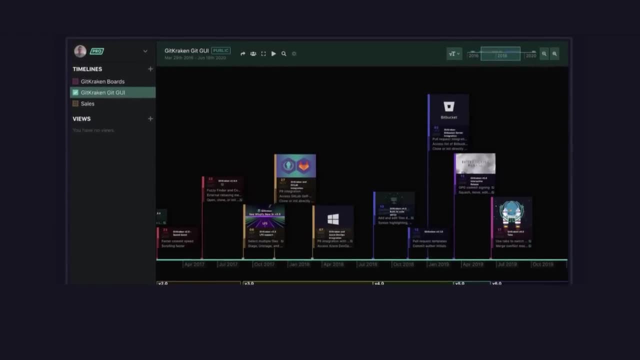 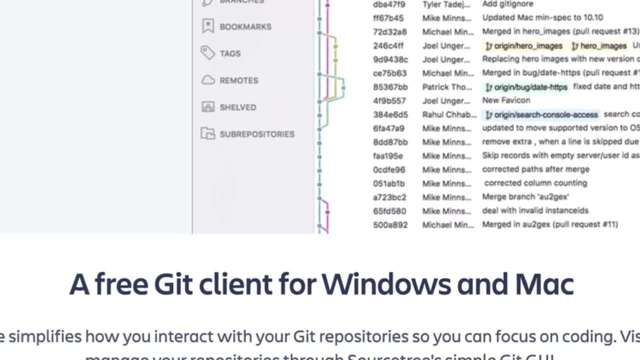 Just to let you know I'm not an affiliate of GitKraken, I'm just a fan. The other option is SourceTree. It's completely free, but it's only available for Windows and Mac, So if you're a Linux user, you have to use GitKraken or another GUI tool. 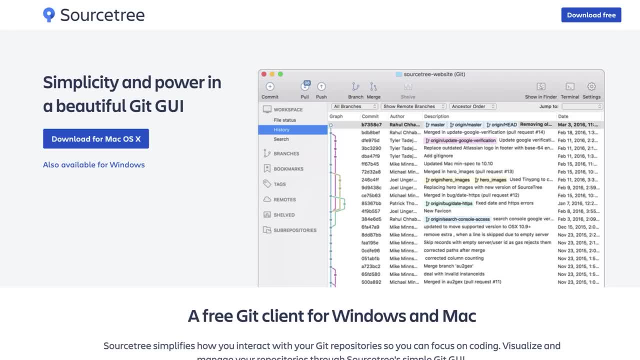 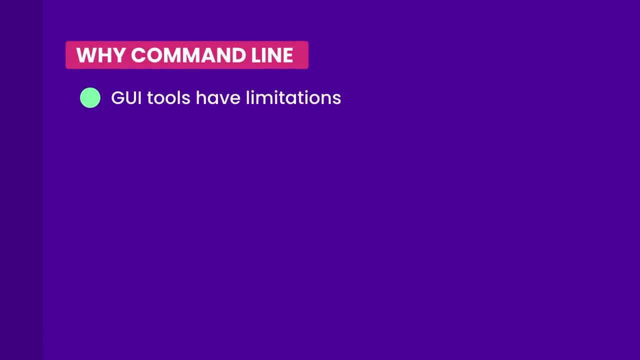 In this course we'll be spending most of our time on the command line for a couple of reasons. The first reason is that pretty much all of these GUI tools have some limitations. They support the Git commands that people use most of the time. 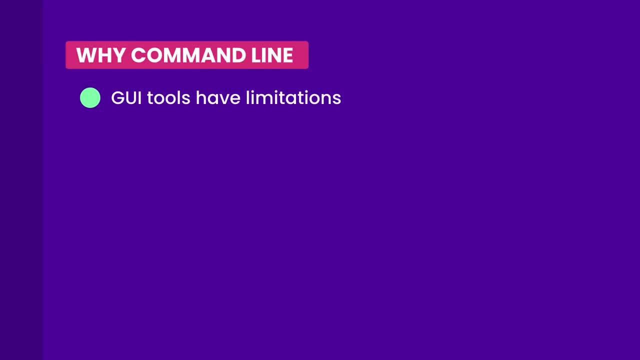 So, even if you want to use a GUI tool, there are times you would have to pay an annual fee. There are times you would have to roll up your sleeves and get back to the command line to get the job done. The other reason is that the command line is always available. 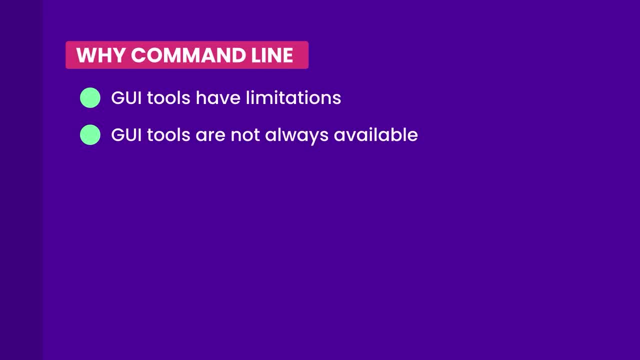 but there are situations where a GUI tool may not be available to you. You might connect to a server remotely and you might not have permission to install a GUI tool. If you don't know how to use the command line, then you're stuck. 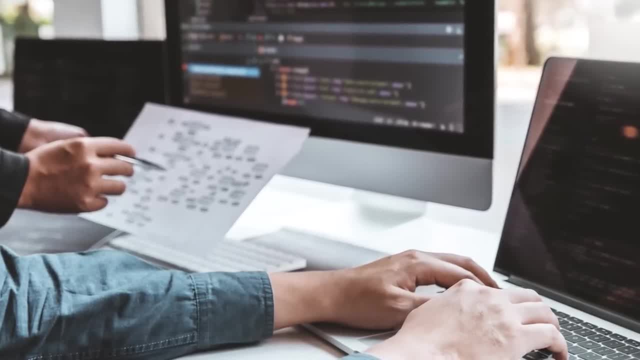 In practice. a lot of people, including myself, use both the command line and a GUI tool, and that's what I'm going to show you in this course. There are times that it really makes sense to use a GUI tool and not a command line. 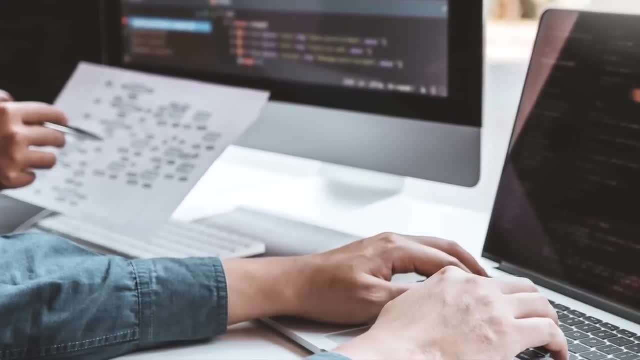 but there are times that it really makes sense to use a GUI tool and not a command line. but there are other times that using the command line is faster and easier. but there are other times that it really makes sense to use a GUI tool and not a command line. 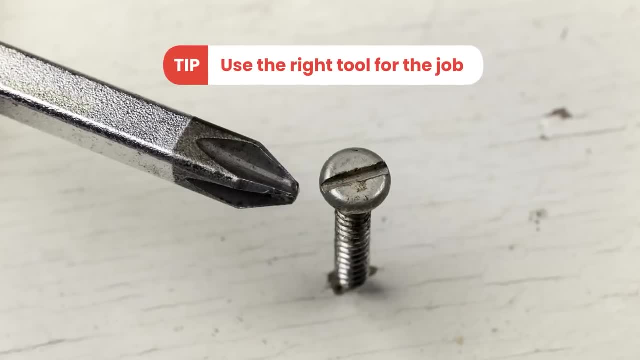 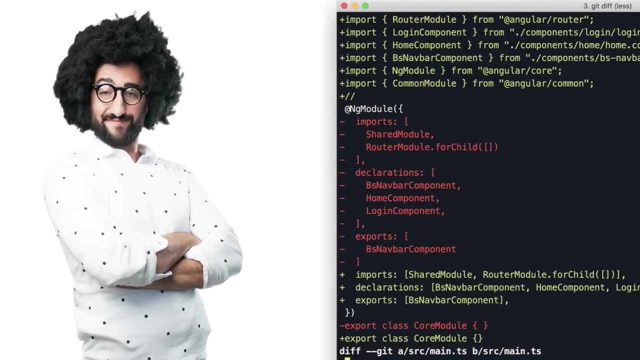 so we'll use the command line. At the end of the day, you should use the right tool for the job. Don't be like this guy. You probably know him, Our popular superstar developer called John Smith. He thinks he's better than everyone else. 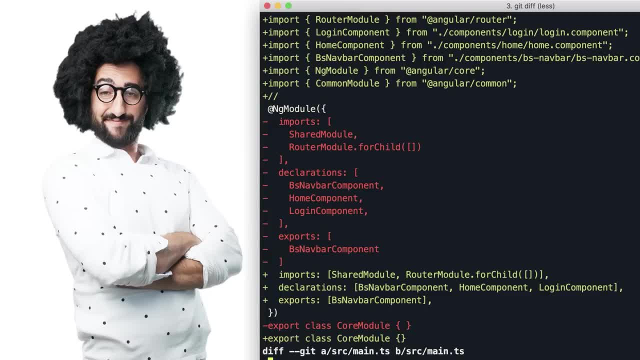 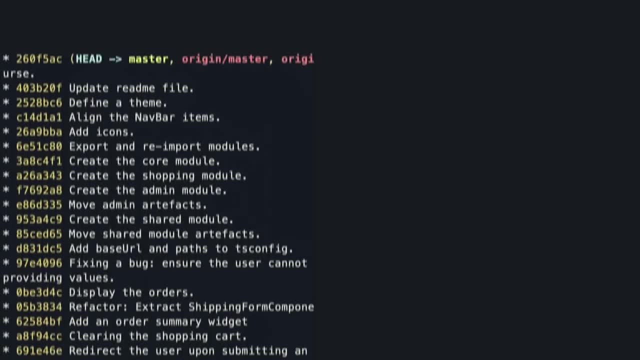 because he does everything in the command line. He never uses a GUI tool and he looks down at people who do. Well, let him think whatever he wants. if that's what makes him happy, Who cares? So we'll be spending most of our time on the command line. 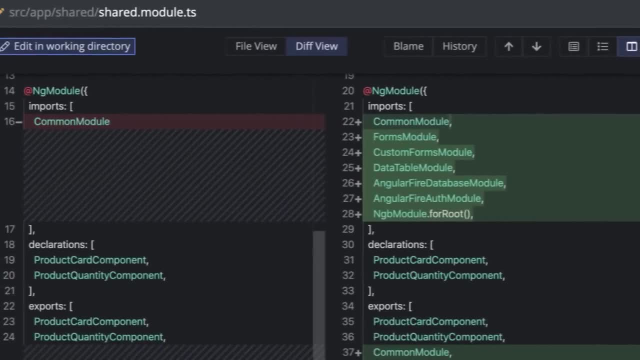 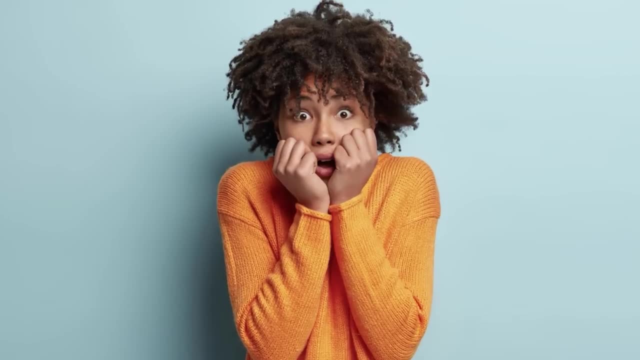 but when it makes sense to use a GUI tool. I'll be showing you examples in VS Code and GitKraken, because those are the most popular tools. Now, if you've never worked with a command line before, don't worry, I'm going to hold your hands. 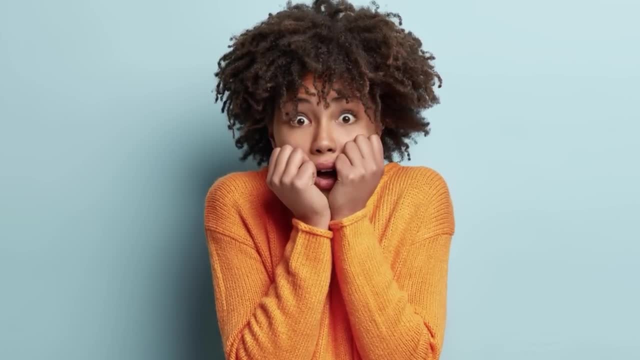 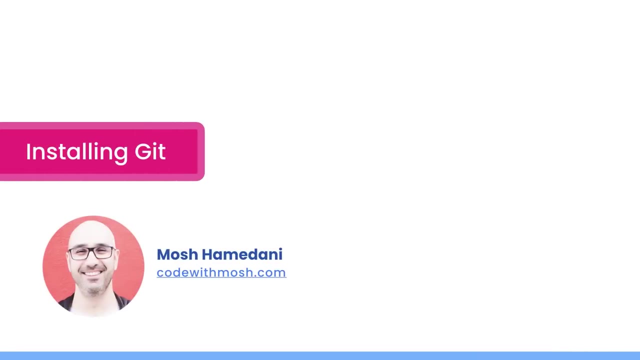 and teach you everything step by step. It's a lot easier than you think. So next we're going to install Git. Alright, let's see if you have Git on your machine or not and if yes, what version you have installed. 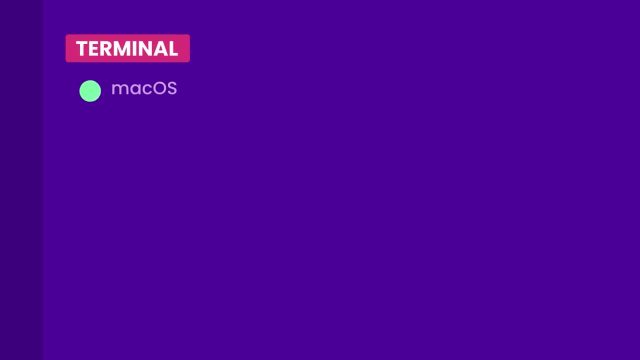 To do this, you have to open a terminal or a command prompt window. If you're on Mac, press command and space and type terminal. If you're on Windows, click the search icon on the bottom navigation bar and type cmd. 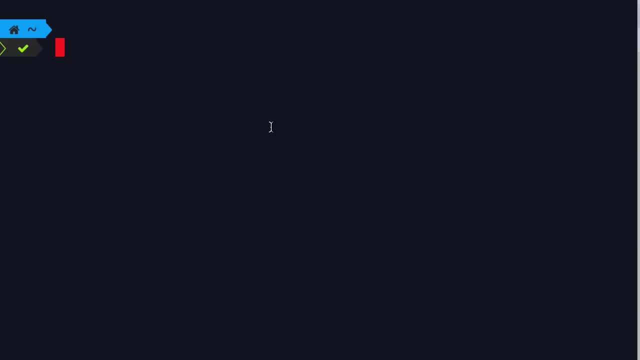 So here's my terminal or console window. your terminal window might look different, it doesn't matter. This is where we're going to execute Git commands, So let's look at the version of Git on this machine. We type git dash, dash version. 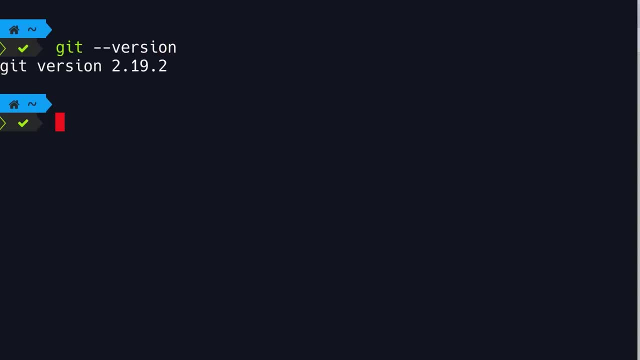 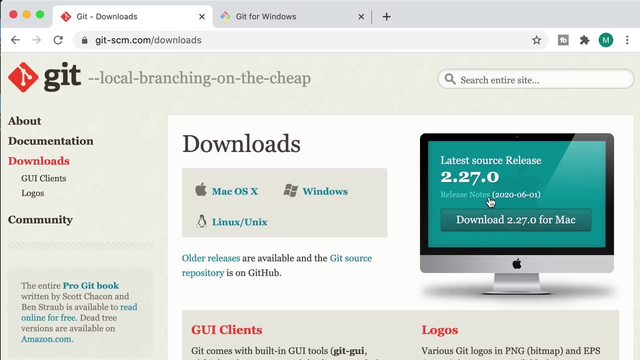 so on this machine I'm using Git version 2.19.2,, but the latest version at the time of recording this video is 2.27.0.. So I highly encourage you to download and install the latest version. just head over to. 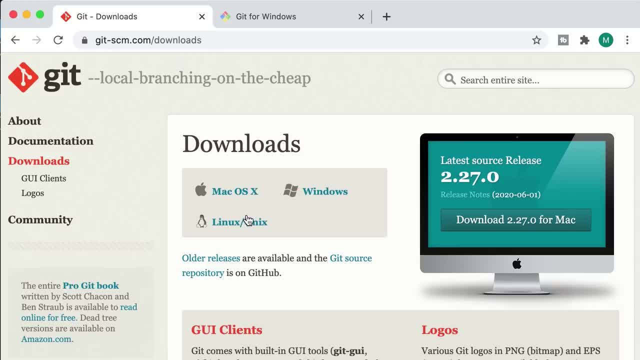 git dash, scm dot com. slash download. Over here you can find instructions for installing Git on different operating systems. it's really easy. you're not going to have any problems. Now, if you're on Windows, once you install Git, you're going to get this application. 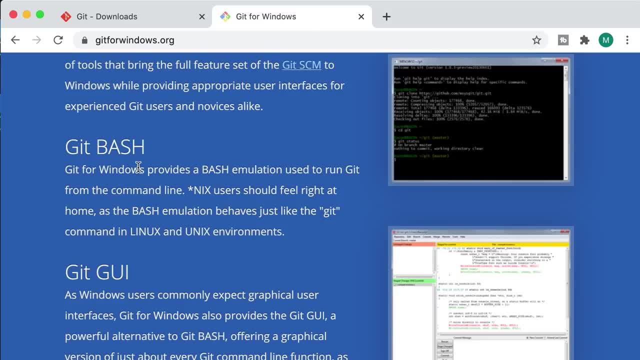 called Git Bash, which is short for born again shell. This is basically a command prompt window like this one over here, but it emulates Unix or Linux environments. So throughout this course, I encourage you to use Git Bash instead of the built-in. 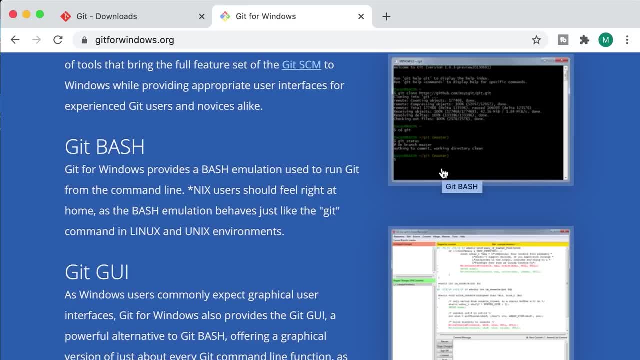 command prompt window. so what you see on the screen looks closer to what I'm going to show you in this course. So go ahead and install Git. in the next lesson I'm going to show you how to customize our Git environment. The first time we use Git, we have 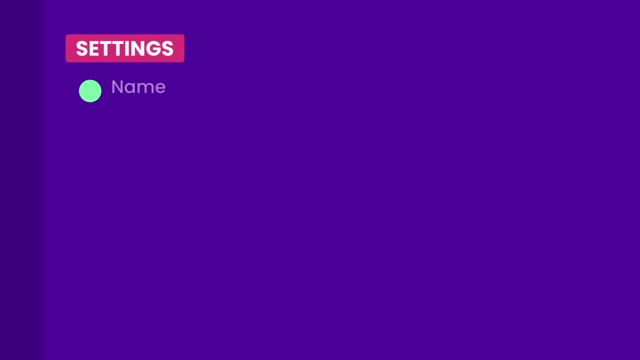 to specify a few configuration settings. We have to specify our name, email default editor and how Git should handle line endings. We can specify these configuration settings at three different levels. At the very top we have the system level: the settings that we have. 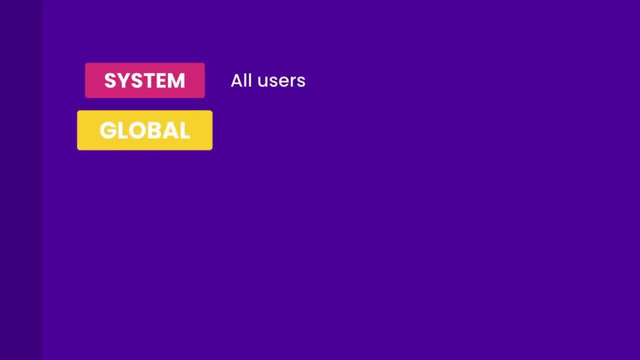 here apply to all users of the current computer. Below this level we have the global level. the settings here apply to all repositories of the current user, And below this level we have the local level. the settings here apply to the current repository or the repository in the current folder. 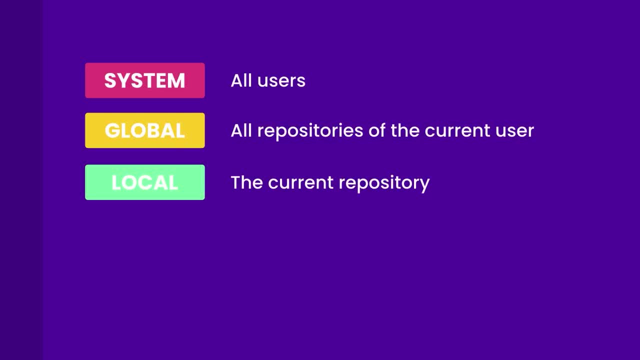 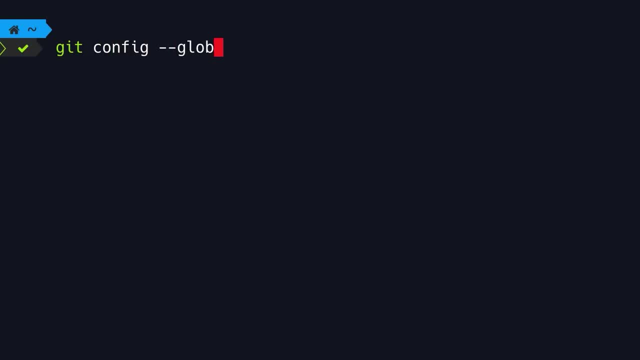 So we can have different settings for different repositories or different projects. So here in the terminal window we type Git config, then we type dash, dash, global, to specify the level at which we are defining these settings. Next we should specify the setting we want to configure, So user. 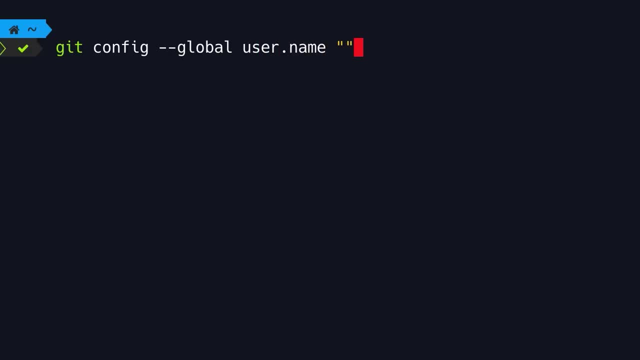 that name. here we type double quotes and type our name now. the reason we are adding double quotes is because we have a space in this value. Okay, So that was the first setting. once again, Git config: dash, dash, global. 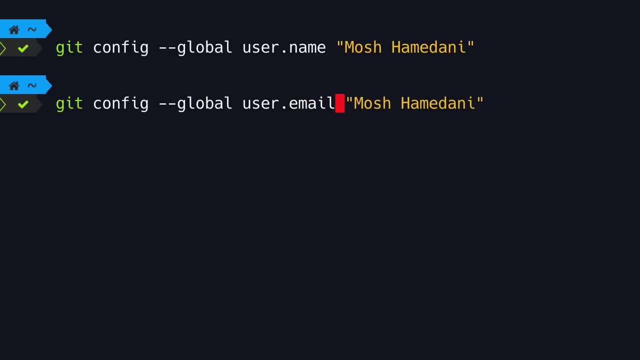 this time we are going to set user that email now, because we don't have a space in emails here. we don't need double quotes, so let's add our email, Alright. next we need to specify our default editor. If you don't, 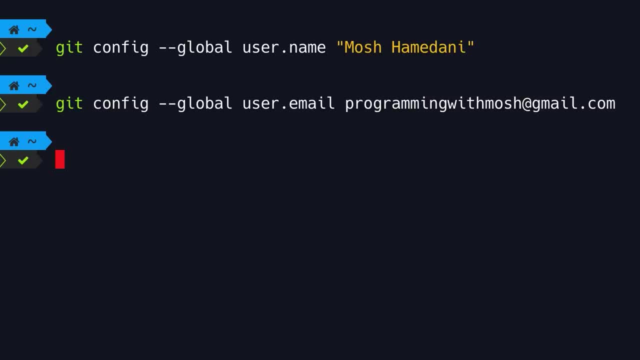 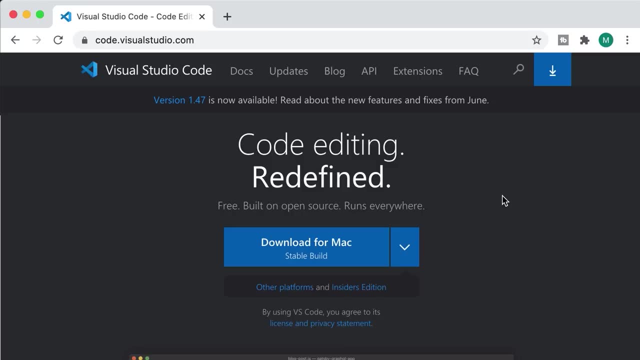 set this on Mac by default. Git is going to use vim, which is a scary editor. a lot of people are freaked out by it. In this course, I'm going to use visual studio code or vs code. you can use any editor that you prefer. 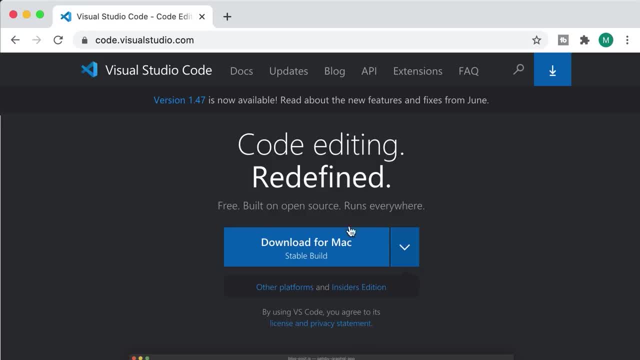 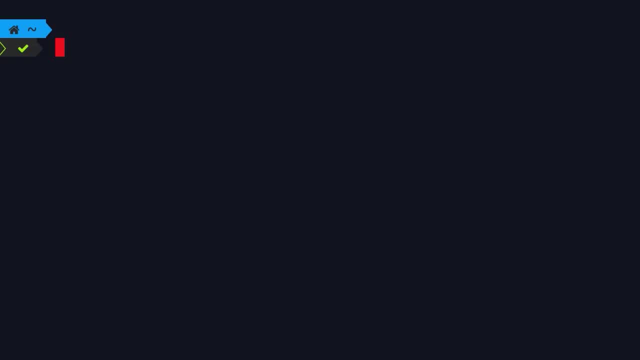 But if you want to follow along with me, I highly encourage you to download the latest version of visual studio code from codevisualstudiocom Now on this machine. I've added visual studio code to my path so I can open it from any folder on my machine. 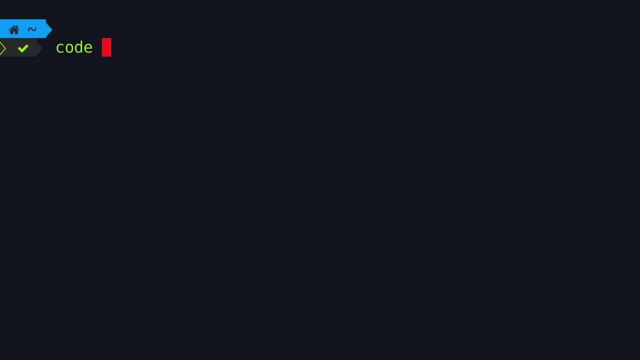 without specifying the full path. So if I type code, here's vs code. if this doesn't work on your machine, you have to troubleshoot the issue yourself. depending on your operating system, there are different instructions for adding vs code to your path. 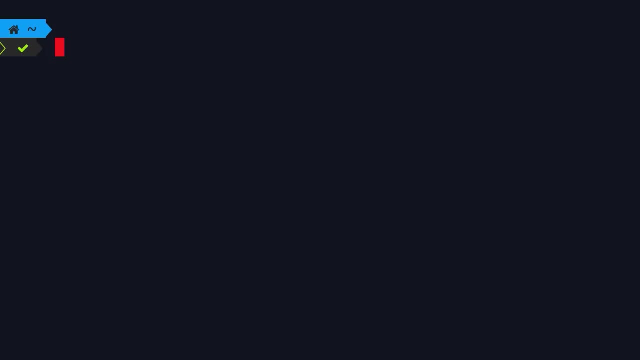 So back to the terminal. let's set the default editor: git config, dash, dash, global. the setting we want to configure is coreeditor. once again, we need double codes, because here we're going to have a space. the value for this setting is code. 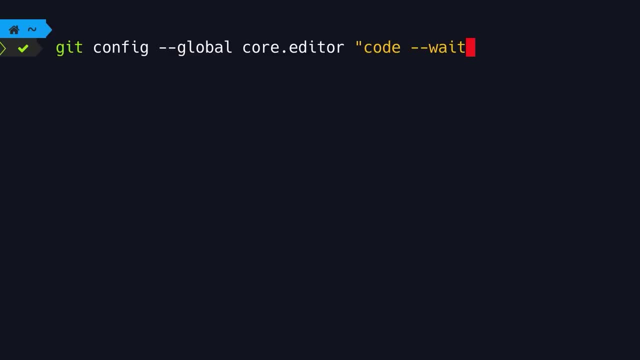 space, dash, dash, wait. With the wait flag we tell the terminal window to wait until we close the new vs code instance. So let's go ahead now. all these configuration settings are stored in a text file. we can edit that file using our default editor. 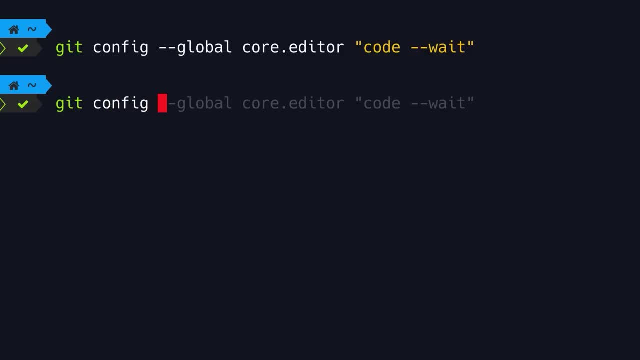 in this case, vs code. So we can type: git config, dash, dash, global, dash e. this will open our default editor to edit all the global settings. let me show you so. alright, here's our configuration file. you can see the full path to this file on the top. 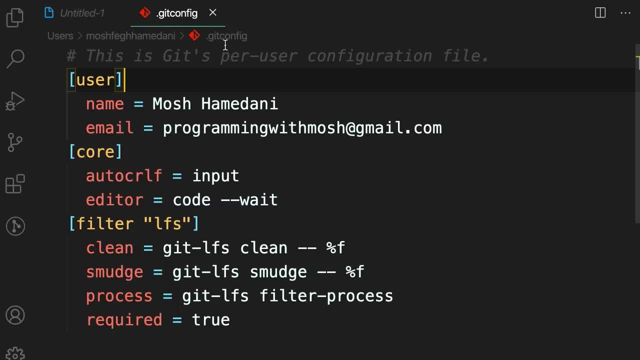 the name of this file is git config. now in this file we have different sections. so we have the user section with two settings: name and email. we have the core section with these two settings, and so on. Now back in the terminal window. 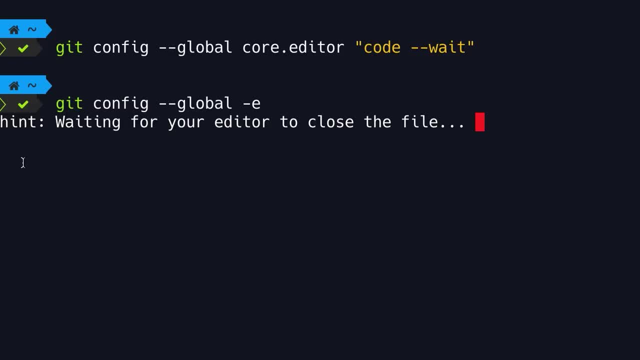 you can see the terminal is waiting for us to close vs code. so let's close this window and let's go back to the terminal. now we are back in the terminal and we can execute the next command. Next, we are going to configure how git should handle. 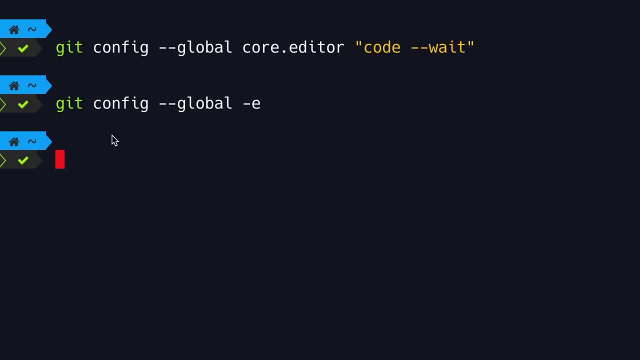 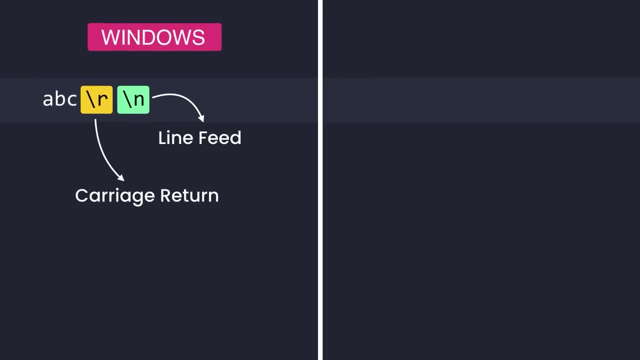 end of lines. this is a very important setting that a lot of people miss. So on windows, end of lines are marked with two special characters: carries, return and line feed. On mac and linux systems, end of lines are indicated with line feed. 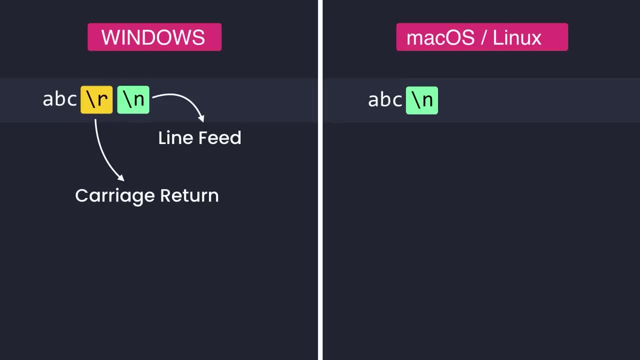 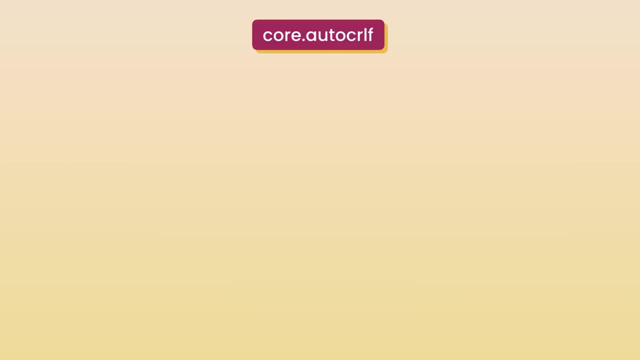 so that means if we don't handle end of lines properly, we are going to run into some weird issues down the road. To prevent this we have to configure a property called coreauto crlf, which is short for carries return line feed. 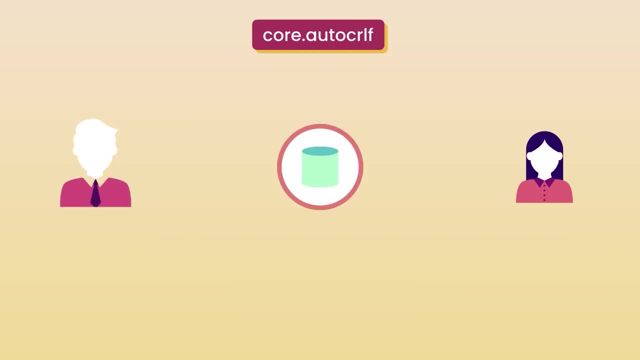 So let me walk you through a real scenario. Let's say we have two people here, John and Julie, working with the same repository. John uses a windows machine, Julie uses a mac, As I told you on windows. end of lines. 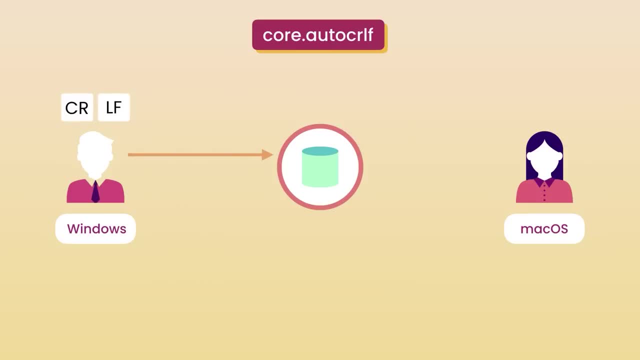 are marked with carries return and line feed. So when John wants to check in his code into the repository, git should remove the carries return character from end of lines. Similarly, when he checks out his code from the repository, git should update end of lines. 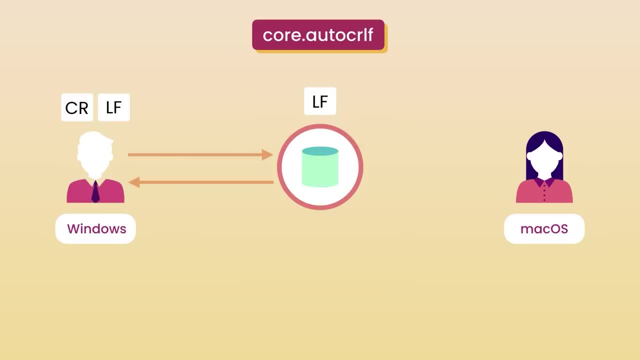 and add the carries return character. To achieve this behavior, we should set this property to true. On the other hand, when Julie checks out the code, she doesn't want the carries return character, So git shouldn't touch end of lines. However. 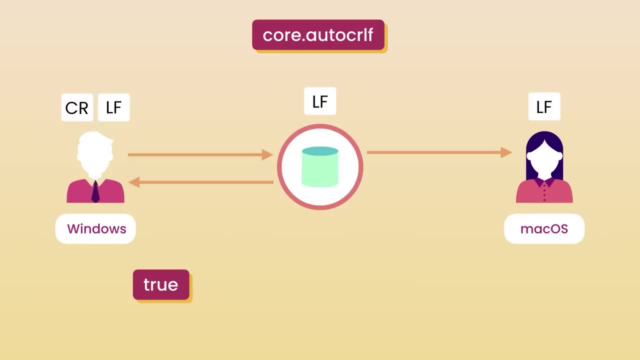 if carries return is accidentally added to end of lines, perhaps because of the editor that Julie is using, git should remove it when storing the code in the repository. To achieve this behavior, we should set this property to input, which means git should only move the. 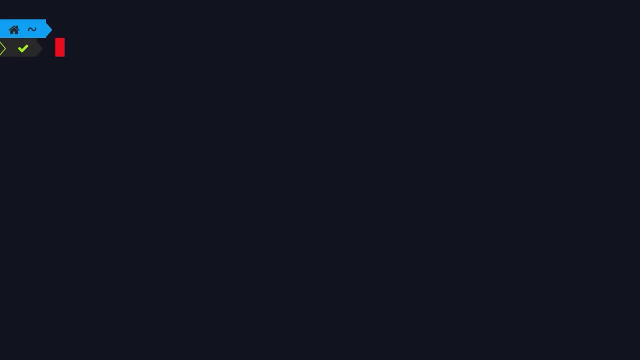 end of lines when storing code in the repository. So back in the terminal we type git config, dash, dash global core dot auto crlf. if you're on windows, you should set this to true. if you're on mac or linux, you should. 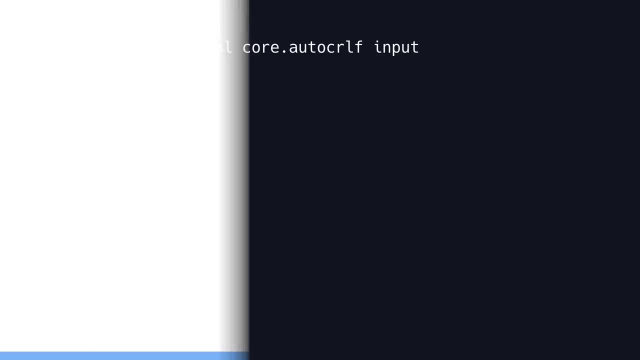 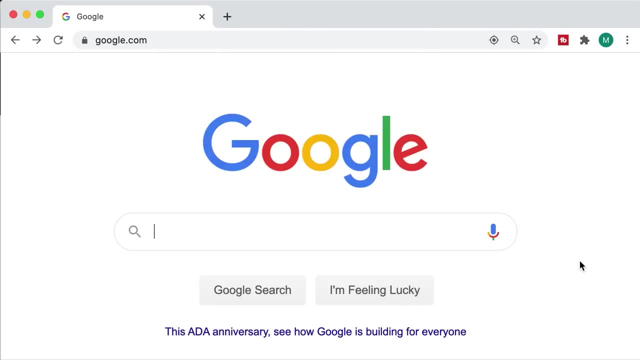 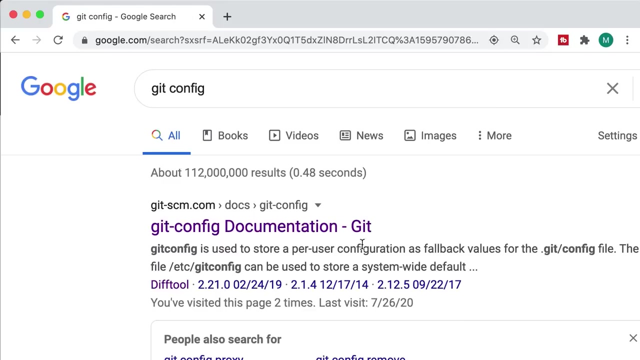 set this to input. Let me show you a few different ways to get help about git commands. Let's say you want to learn more about the config command. You can simply google git config on this page. you can see the full documentation of this command. You can see various options. 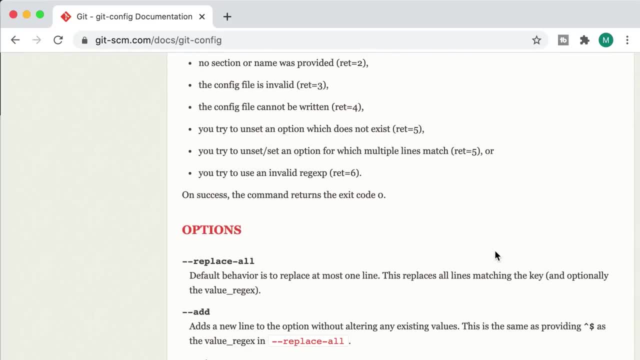 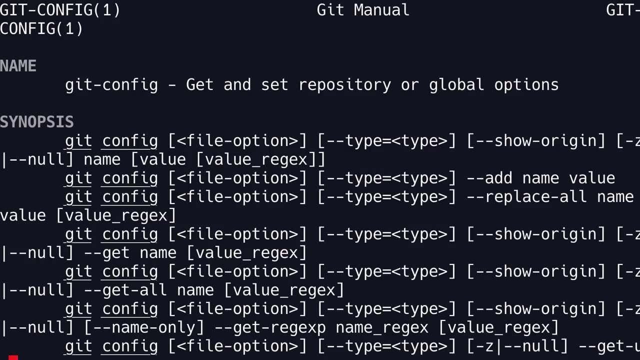 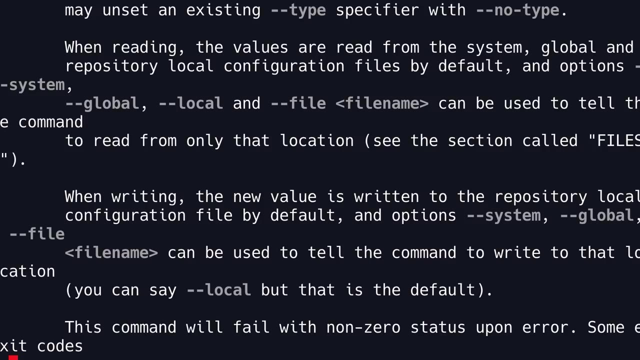 and how they work. We can also access the same page on the terminal window. We simply type git config, dash, dash, help. This is exactly the same information you saw a second ago. Now here we can press space to go to the next page and 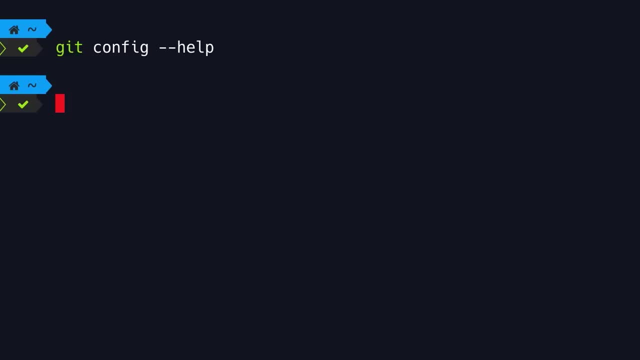 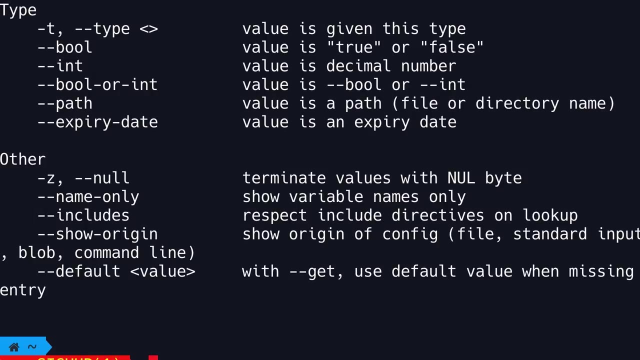 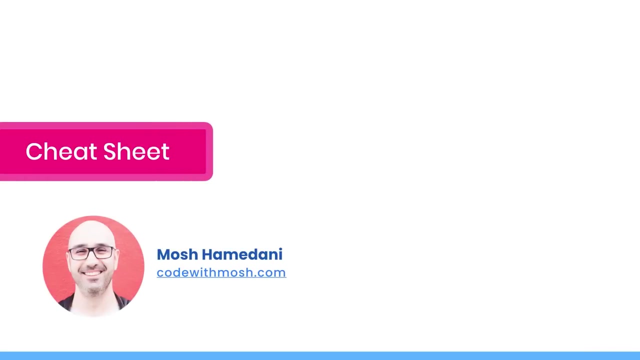 q to exit. Now if you don't need a full blown help, you just need a quick refresher. you can type git config dash h. This gives us a short summary of this command and its options. So we're done with the introductory stuff starting. 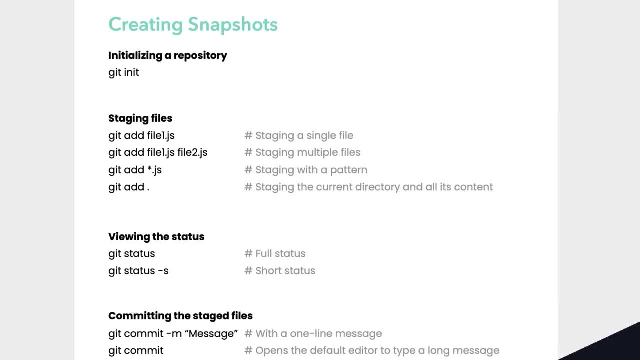 from the next section, we're going to cover a lot of git commands. Now, below this video, we can download a pdf of all the commands we're going to cover in this course. If you're starting out, don't worry too much about memorizing these commands. 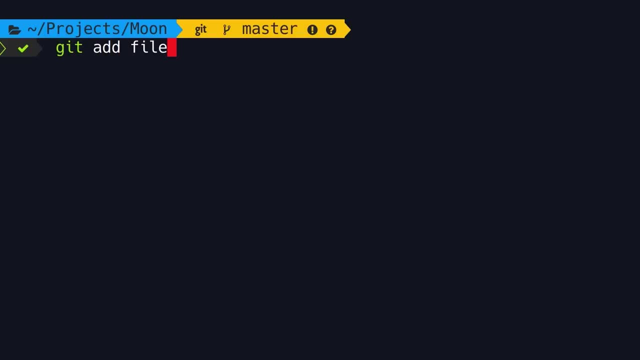 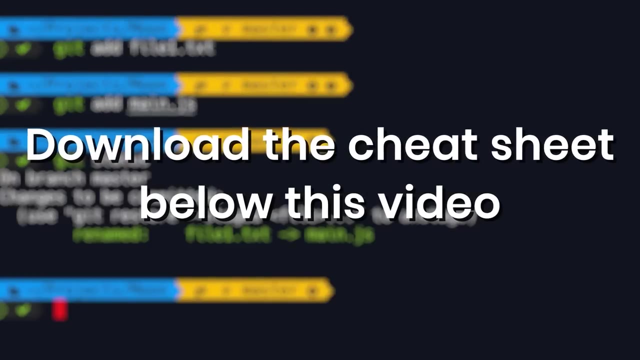 instead try to understand how they work. As you practice git in the real world, all these commands are going to become second nature to you, trust me. So download the cheat sheet below this video, and then I will see you in the next section. 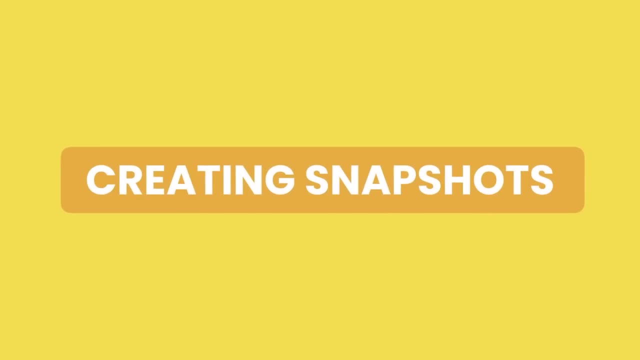 The first thing you need to know to use git effectively is how to take snapshots of your project, which is what we're going to talk about in this section. We'll be talking about the fundamental concepts in git that are often misunderstood, So make sure to watch every lesson in this section. 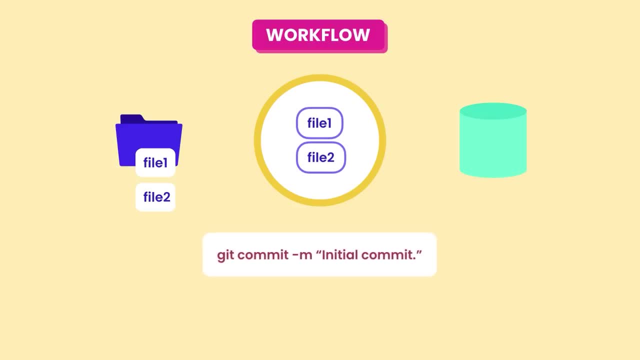 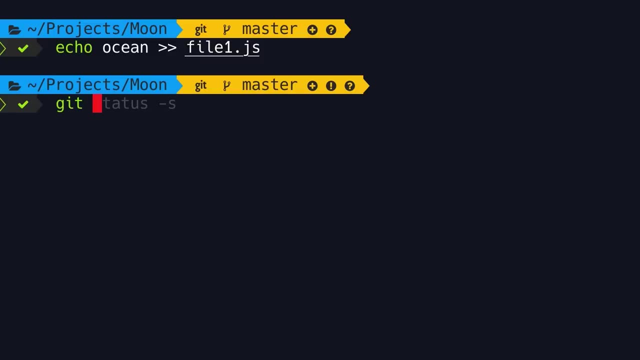 even if you think you know the basics, a lot of people use the basic git commands without having a proper understanding of how git works, and that's why they constantly get stuck. So watch every lesson in this section. Now let's jump in and get started. 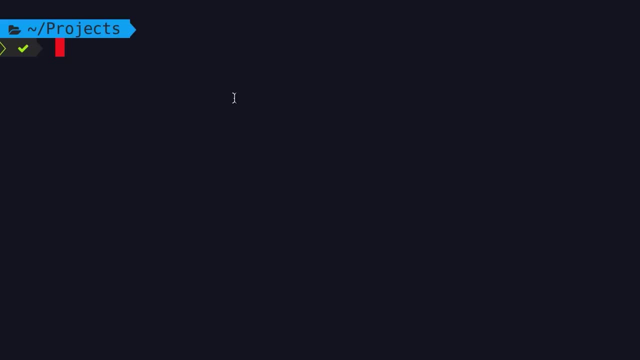 Alright, the first thing we're going to do is create a directory for our project. You can call this directory anything and put it anywhere on your machine, it doesn't matter. I'm currently in the projects directory, so let's create a directory. 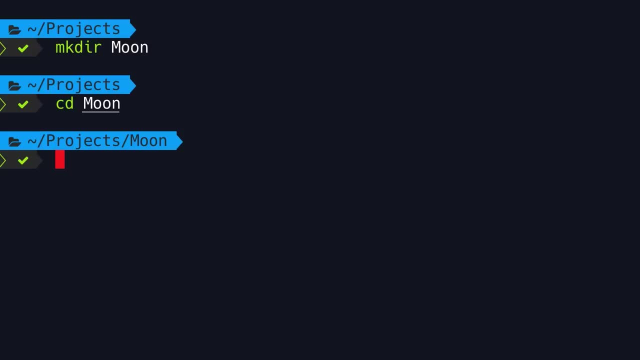 called moon and then go into this directory. so let's imagine this is our project directory and here we can have tens or hundreds of files. The first time we want to add this files to a git repository we have to initialize a new empty repository. 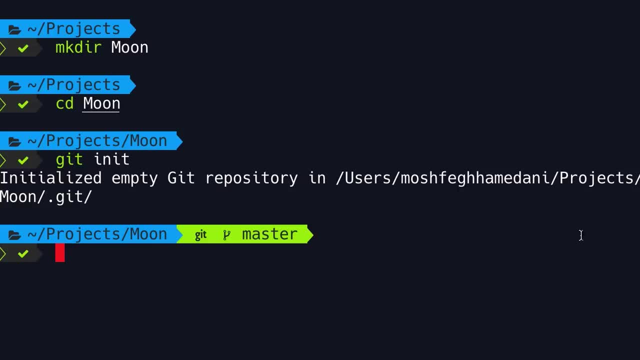 So we type git init. look at this message: initialize empty git repository in. and here's the full path. So we have the moon directory and inside this directory we have to have a subdirectory called dot git. By default, this subdirectory 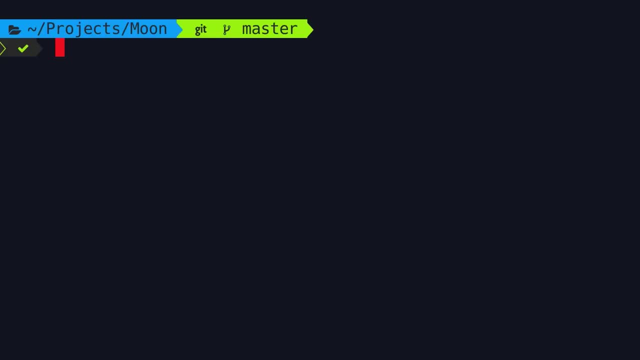 is hidden because you're not supposed to touch it. So if we type ls to list all the files and directories here, we don't see anything. but if we type ls- dash a, which is short for all, we can see the git subdirectory. 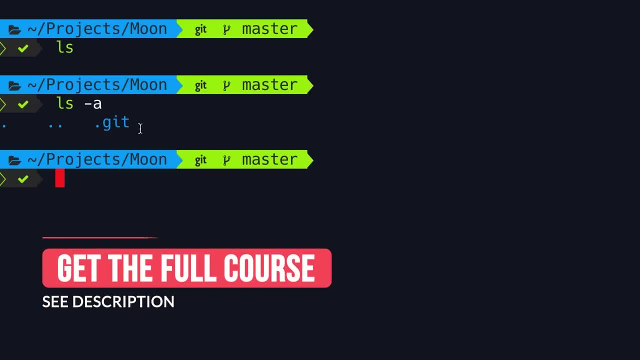 If you're on mac, you can open this with finder, and if you're on windows, you can open it with windows explorer or file explorer- I'm not sure what it's called these days- So let's open dot git. take a look. 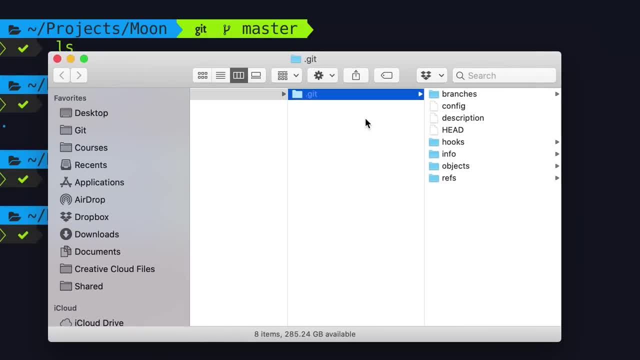 So here's our git directory, or git repository. This is where git stores information about our project history, So we have directories like branches, hooks, info, objects and references. Now, as someone using git, you don't really need to understand. 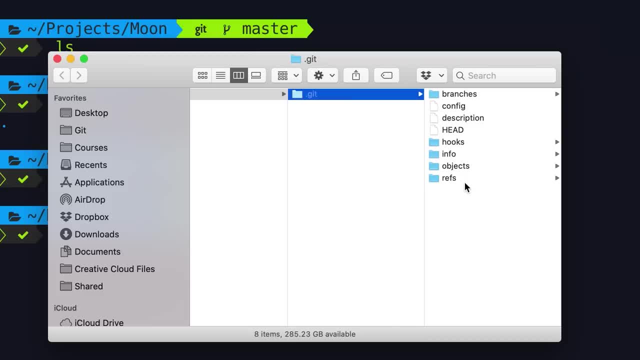 this structure. this is purely implementation detail. It's how git stores information. it's none of our business. That's why this directory is hidden, so you don't touch it. If you corrupt or remove this directory, you're going to lose your project history. 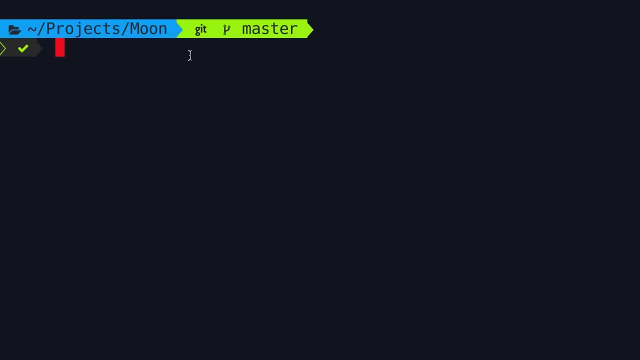 Let me show you. So. back in the terminal, look at this green marker. It says git. That means we have a git repository in this directory. Now if you want to have a pretty colorful terminal window like this on mac, you need to install zsh. 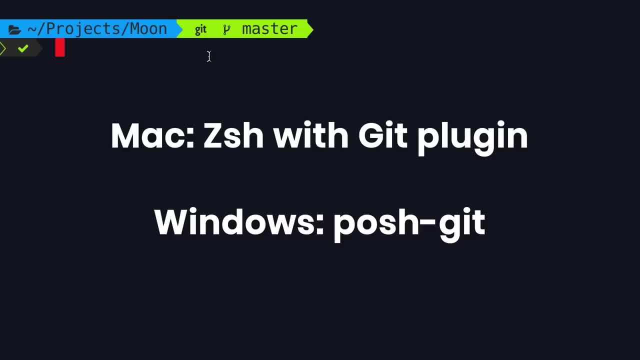 or z shell, and on windows you need to install posh git. But don't worry about it now these tools are completely optional to use git, It's just for making things pretty. So here we have a git repository now, if I 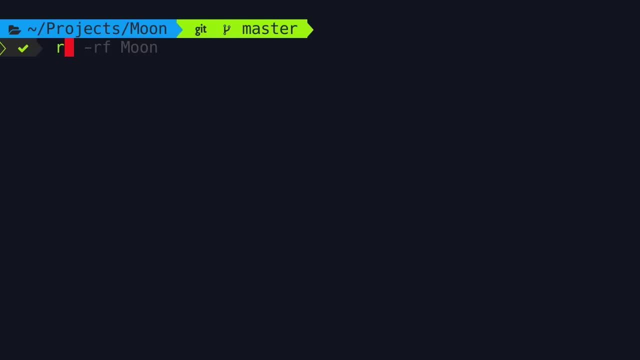 remove the git subdirectory, we're going to lose this repository, So our rm-rfgit. Look, the green marker is gone. We don't have a git repository here anymore, So don't touch this directory Now. once again, let's initialize. 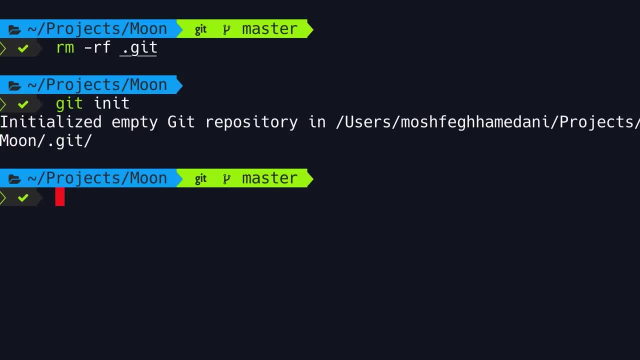 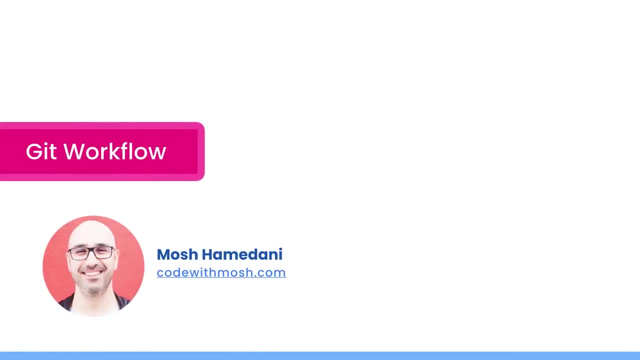 a git repository- beautiful. So now that we have a repository, next we're going to talk about the basic git workflow. Now that we have a git repository, let's talk about the basic git workflow- What we do on a daily basis when using git. So here's our project. 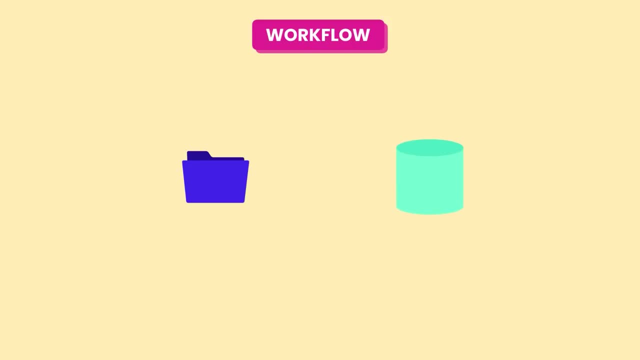 directory. and here's our git repository, which is actually a hidden subdirectory in our project directory. Now, everyday, as part of working on various tasks, we modify one or more files. When our project reaches a state we want to record, we commit. 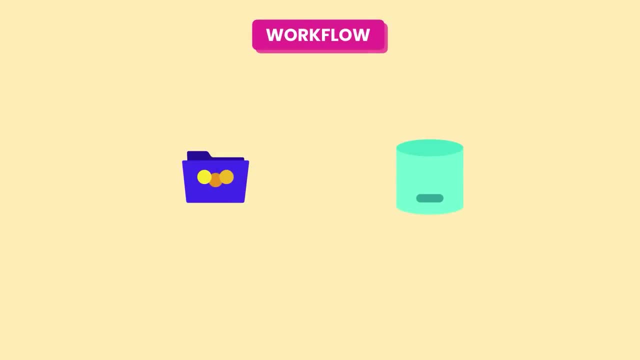 those changes into our repository. Creating a commit is like taking a snapshot of our project. Now in git we have a special area or a special intermediate step that doesn't exist in most other version control systems. It's called the staging area or the index. 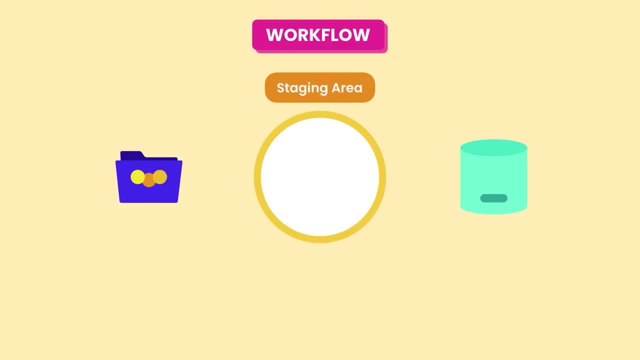 It's essentially what we're proposing for the next commit or the next snapshot. So when we're done making changes, we add the modified files to the staging area or index, review our changes and if everything is good, then we'll make a commit. 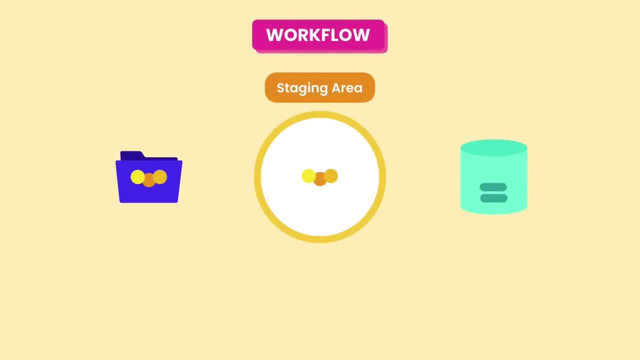 The proposed snapshot will get permanently stored in our repository, So the staging area allows us to review our work before recording a snapshot. If some of the changes shouldn't be recorded as part of the next snapshot, we can unstage them and commit them as part of another snapshot. 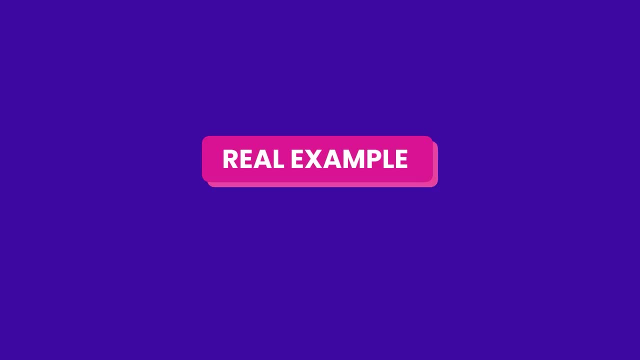 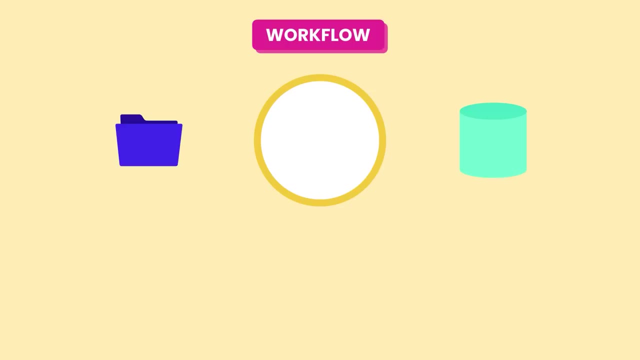 That's the basic git workflow. Now let me walk you through a real example. This example is crucial, so pay close attention all the way to the end, even if you think you know the basics. Our project directory is currently empty, So we add a couple of files here. 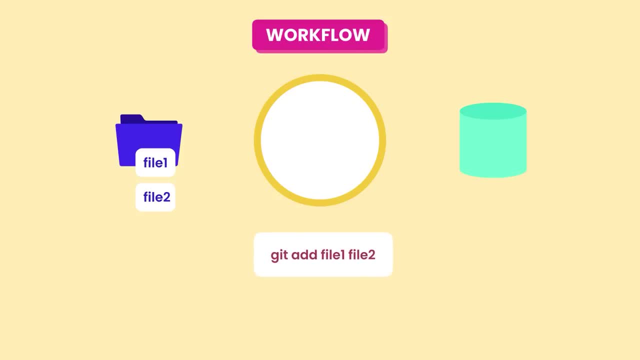 Now we're ready to record this state, So we use the add command to add these files to the staging area. Now these files are in the staging area. This is the state we're proposing for the next commit. We review these files. everything is good, so we use. 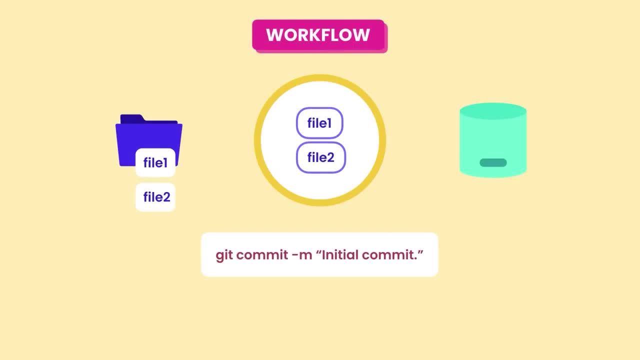 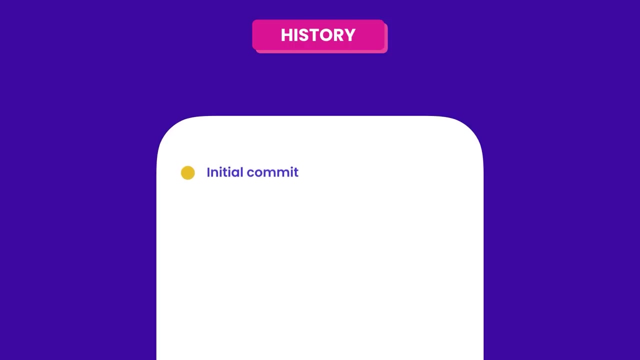 the commit command to permanently store this snapshot in the repository. As part of this, we supply a meaningful message to indicate what this snapshot represents. This is essential for having a useful history. So as we fix bugs, implement new features and refactor our code, we make commit. 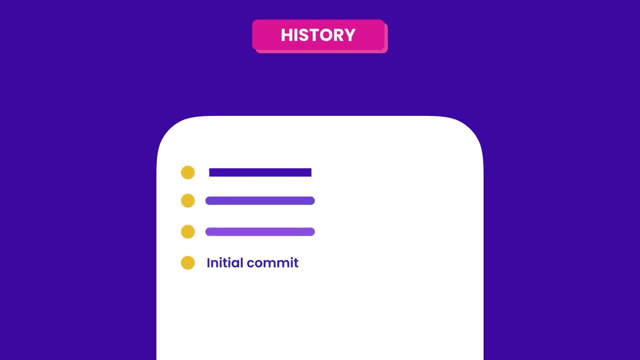 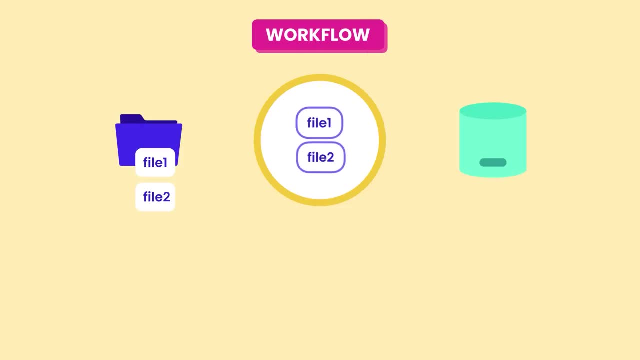 and each commit clearly explains the state of the project at that point in time. So now we have one commit in our repository. Now, a common misconception about git is that once we commit the changes, the staging area becomes empty. This is not correct. 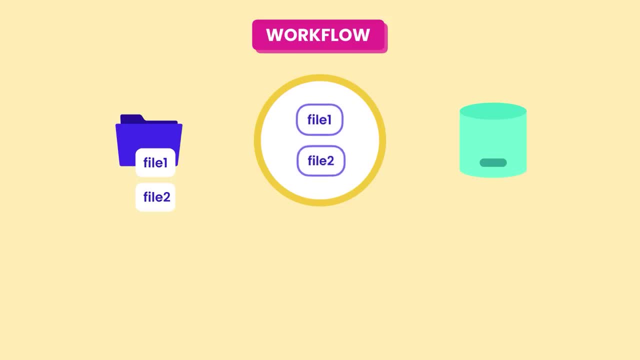 and I think this is why a lot of people find git confusing. So what we currently have in the staging area is the same snapshot that we stored in the repository, So this staging area is actually very similar to a staging environment we use when releasing software to production. 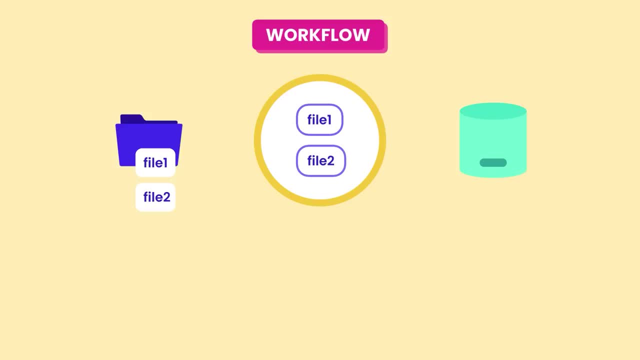 It's either a reflection of what we currently have in production or the next version that's going to go in production. So let's continue with our example. Let's say, as part of fixing a bug, we make some changes to file 1.. 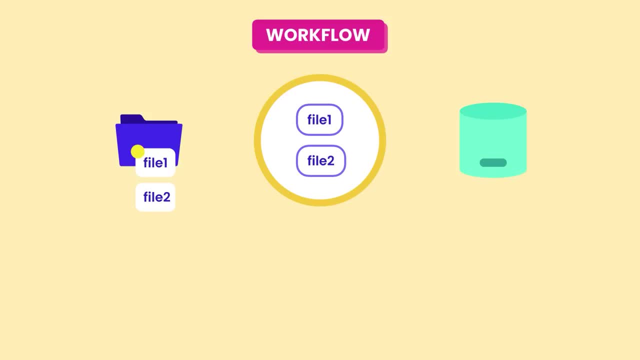 Note that what we currently have in the staging area is the old version of file 1, because we haven't staged the changes yet. So once again, we use the add command to stage the changes. Now what we have in the staging area is the same content we have in our 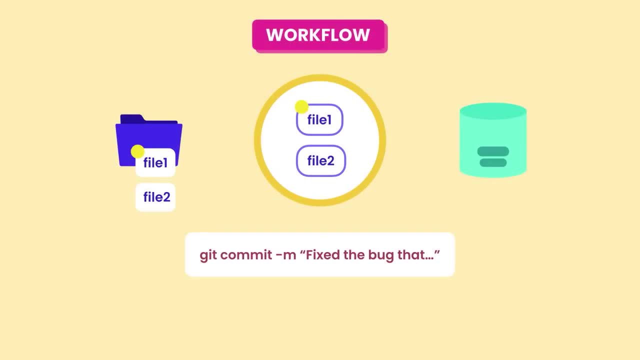 working directory. So let's make a commit to record this state. Now we have two commits in our repository. Also, look at the commit message. it's describing the bug that we just fixed. Now let's say we realize that we no longer need file 2, it contains: 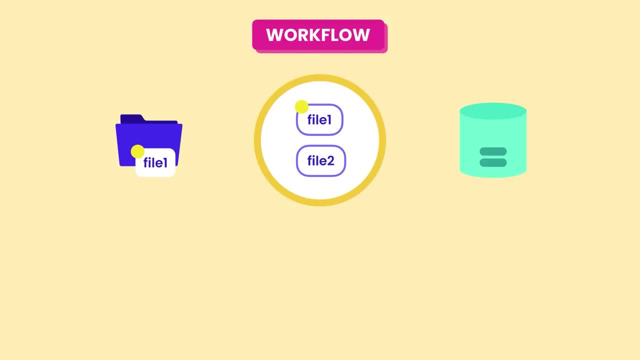 unused code, So we delete it from our working directory, But this file is still in the staging area. So once again, we should use the add command to stage this change, In this case the deletion. This is the interesting part, Even though we're saying add. 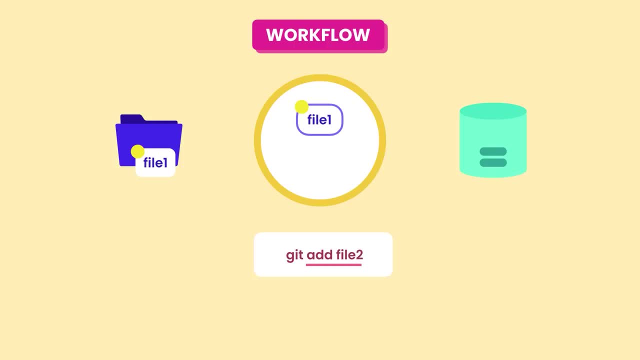 file 2,. git knows that file 2 is actually deleted, So it will delete this file from the staging area or the next snapshot. Again, we make a commit to permanently record this state. Now we have three commits in our repository. Each commit 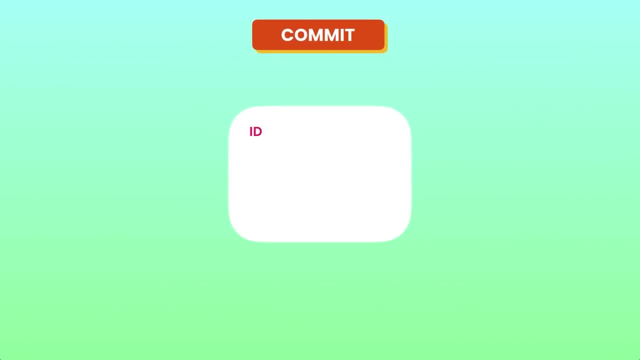 contains a unique identifier that gets generated by git. It's like a revision number. Each commit also contains information about what was changed by who when, as well as a complete snapshot of our project at the time it was created. So, unlike many other version control. 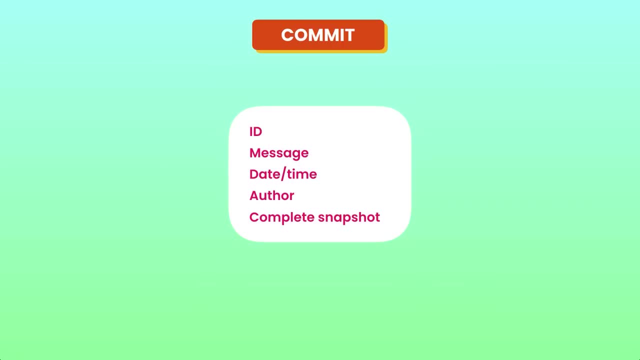 systems. git doesn't store the deltas or what was changed. It stores the full content. With this, it can quickly restore the project to an earlier snapshot without having to compute the changes. Now you might ask: but hey, Mosh wouldn't. storing the full content in every snapshot waste a lot of space. No, Because git is very efficient in data storage. It compresses file contents and doesn't store duplicate content. Now, someone using git- you don't really need to know how git stores data. 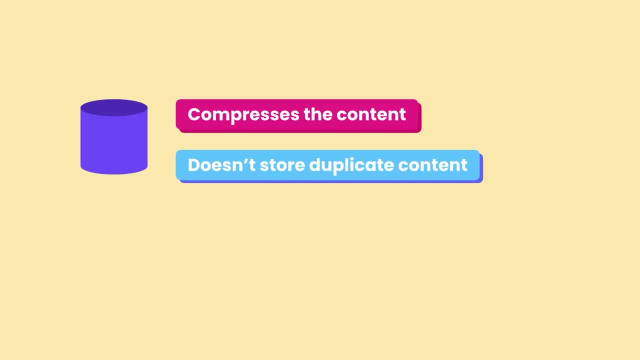 That's implementation detail and may even change in the future. What you need to know is that each commit contains a complete snapshot of our project, and this allows us to quickly get back to a previous state. So that's the basic idea Over the next few. 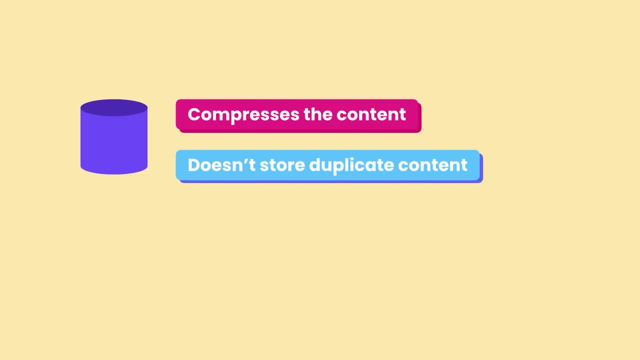 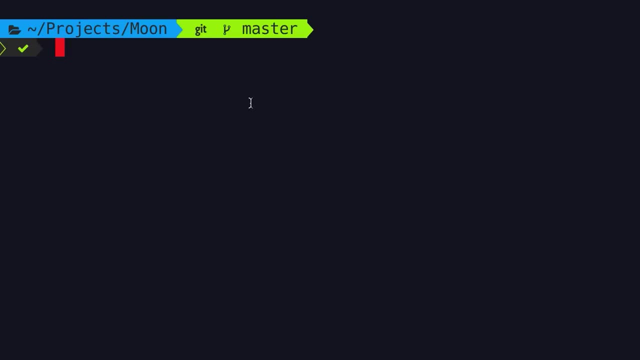 lessons. you're going to see this workflow in action. Let's start by adding a couple of files to our project. To do that, we're going to use the echo command. This is not a git command, it's just a standard unix or linux command. 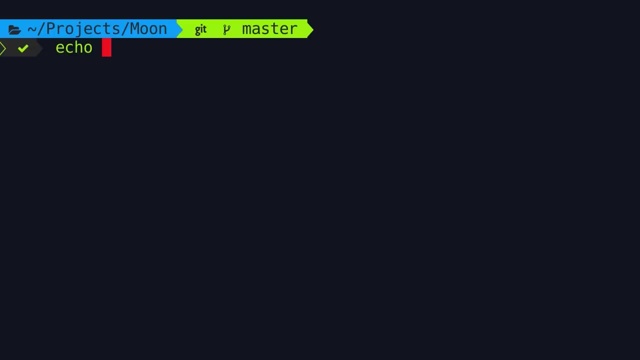 for writing content to a file. So here we're going to write hello to file1.txt. So here I'm working with a text file, because I don't want this course to be specific to people who know a particular programming language, like python or javascript. 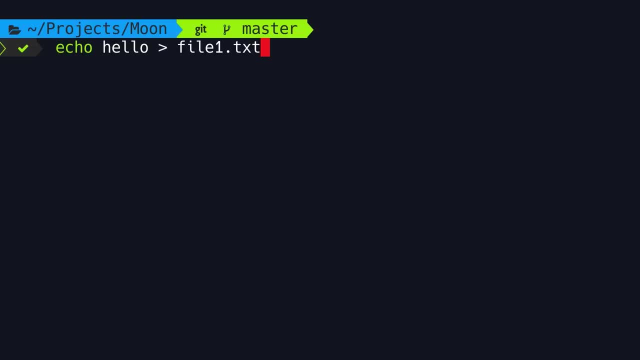 What I'm going to show you in terms of the workflow applies to any programming languages. Okay, So we write hello to file1.txt. Good, Now let's execute this command one more time and change file1 to file2.. So now we have two files in our project. 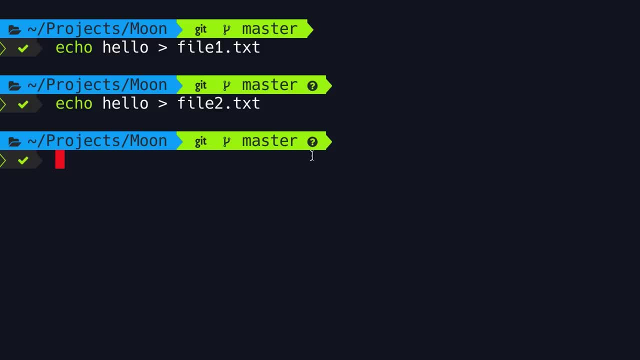 Now look at this question mark here. That means we have new files here that are not tracked by git, Because the first time you initialize a git repository in a directory, git is not going to automatically track your files. So if you have a thousand files in your project, 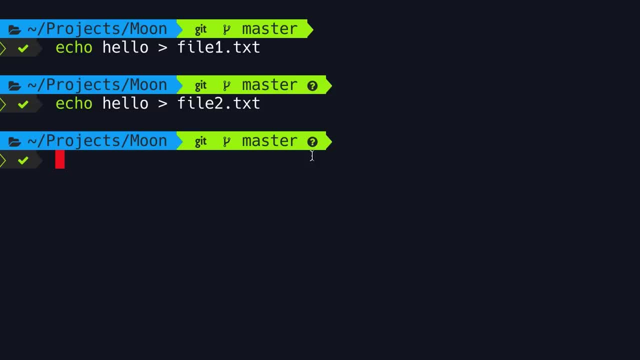 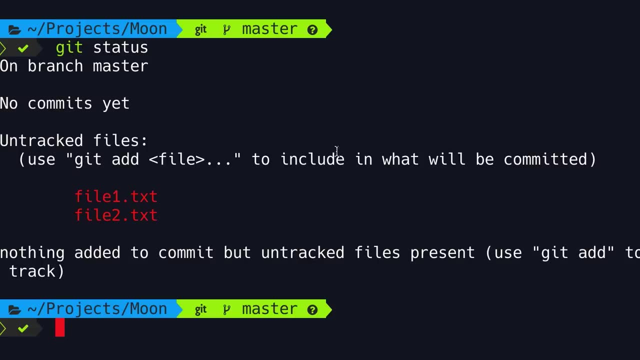 you have to instruct git to track them. Okay, So here we're going to run git status to see the status of the working directory and the staging area. Take a look. So we don't have any commits yet we have untracked files. 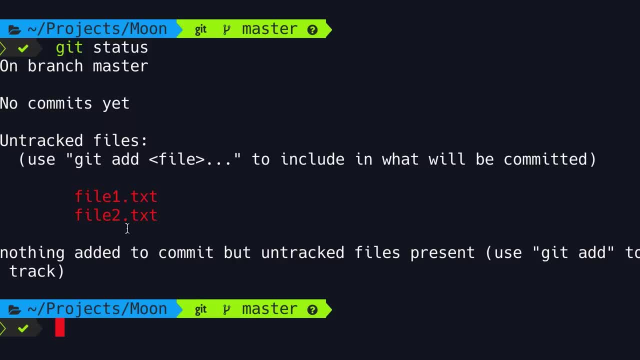 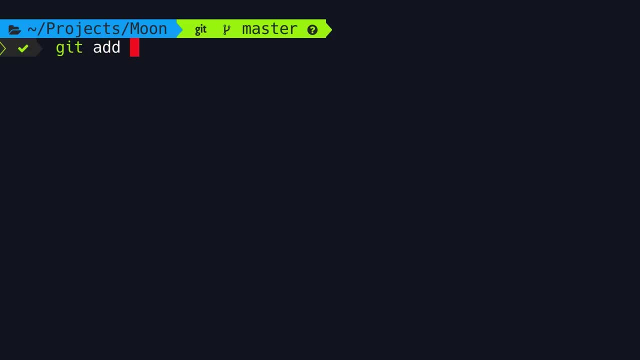 which are file1 and file2, they're indicated by red because they're not in the staging area yet. To add these files to the staging area we use the git add command. Here we can list a single file like file1.txt. 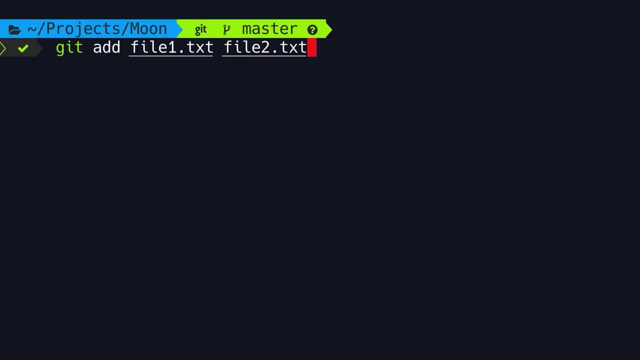 or multiple files separated by a space. we can also use patterns, so startxt, that means all the files with the txt extension. We also have period, which adds the entire directory recursively. Now you have to be a little bit careful with this, because sometimes 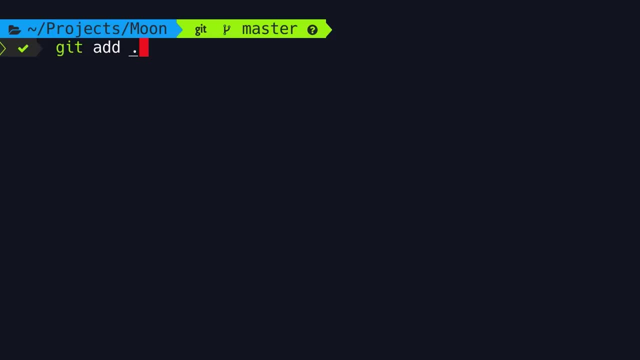 there are files you don't want to add to your repository, perhaps large files like large binary files or log files. you don't want to add these files to your repository because they increase the size of your repository. I will show you how to ignore these files. 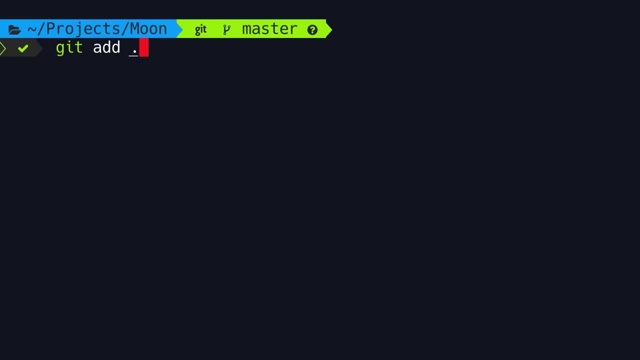 later in this section. So just remember: add period adds the entire directory recursively. In this demo I'm going to go with this command because we only have two files in this directory. okay, Now our green indicator changed to yellow, which means we have: 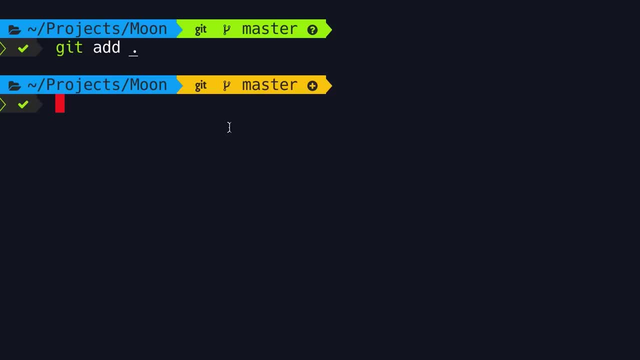 stuff in the staging area that are ready to be committed. So if you run git status again, look, we have two new files and they're indicated by green, which means they're in the staging area. Now let me show you something interesting. I'm going to 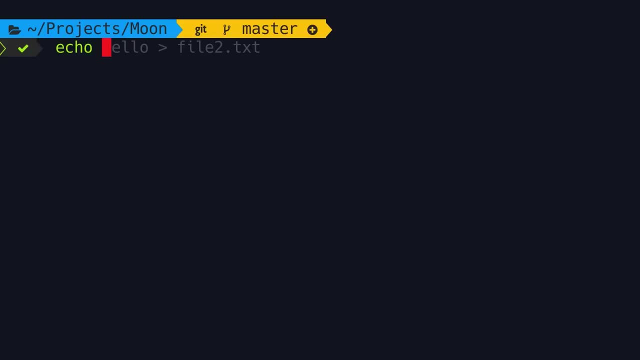 modify file1,. so, once again, we're going to use the echo command to echo world, but here, instead of one greater than one, I'm going to use two greater than signs, which means append, So we're going to append. 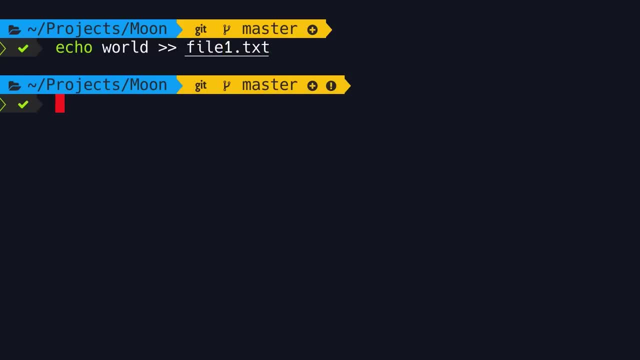 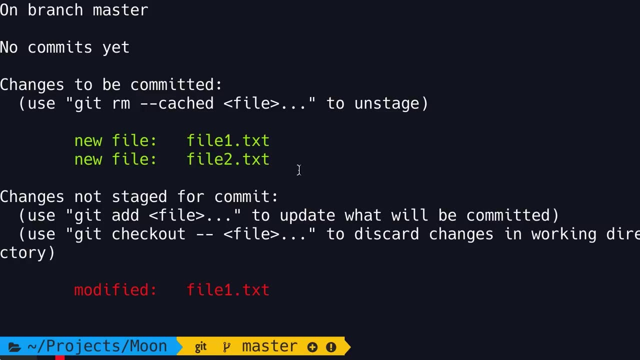 world to file1.txt. Now let's run git status again. look what happened. We have two files in the staging area because they're indicated by green, but we also have one modified file in our working directory. So you might be asking, but hey, Mosh. 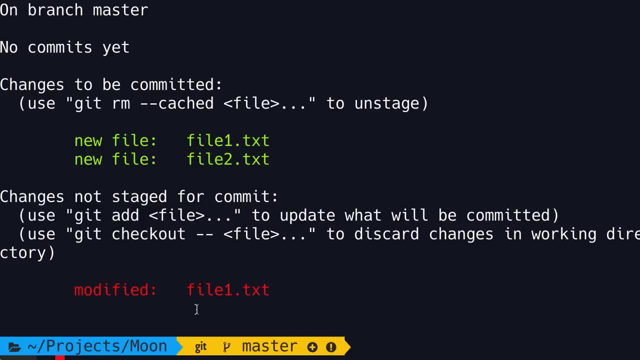 didn't we already add file1 to the staging area? Yes, we did, but when we ran the add command, git took a snapshot of file1 and added that snapshot to the staging area. So we have two files in the staging area. so here's the current situation. 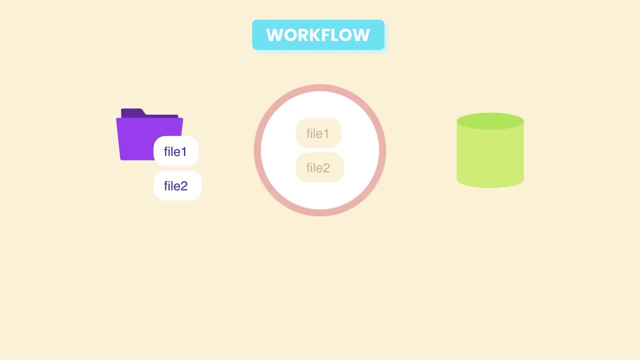 In the staging area we have the first version of file1.. We changed this file after we added it to the staging area, So what we currently have in our working directory is the second version of this file. It has some changes that are not staged yet. 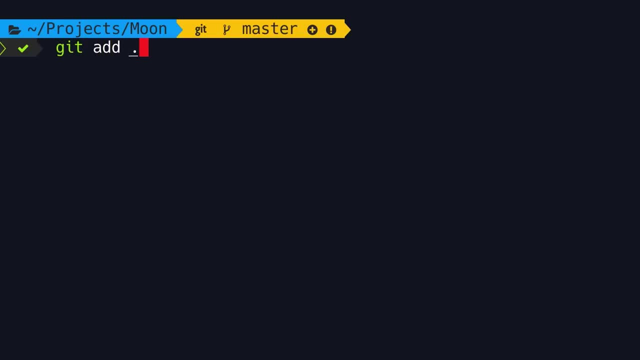 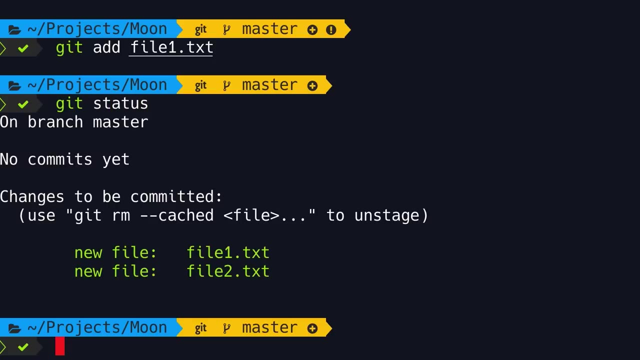 So back to the terminal. we run git add period or git add file1.txt. one more time now look at the status of our working directory. Both these files are in the staging area and we don't have any unsecured files. 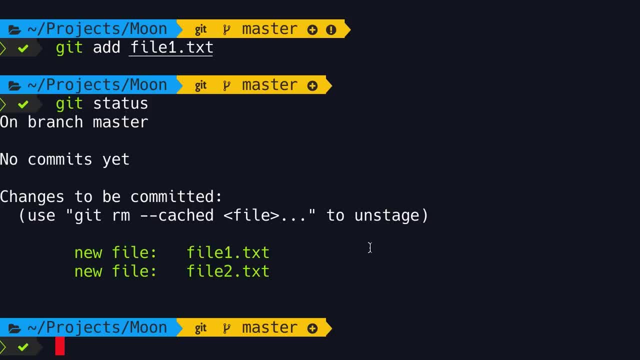 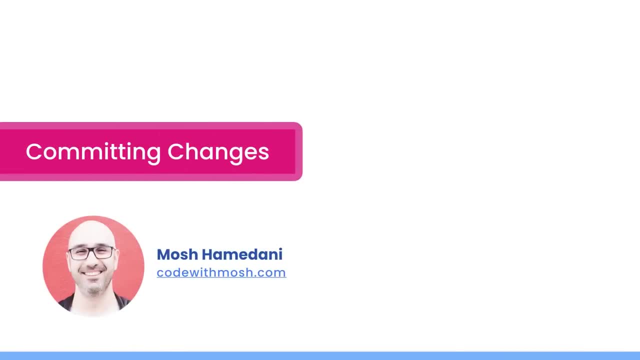 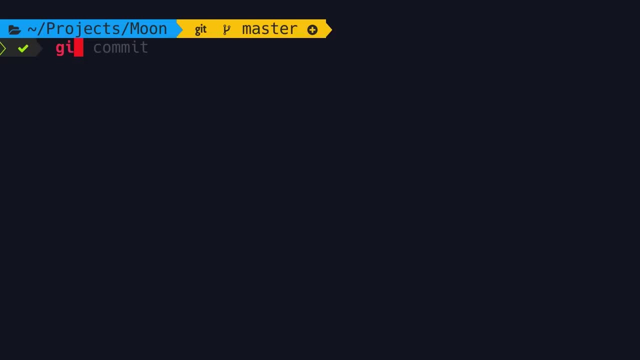 So next I'm going to show you how to commit this snapshot to permanently store it in our git repository. Now we have a snapshot in the staging area ready to be permanently stored in our repository. So we type git, commit, dash m for message and here: 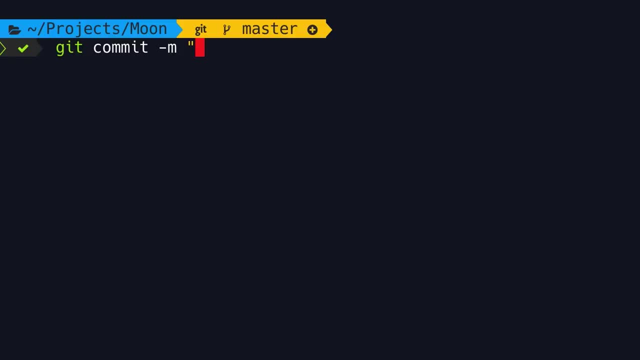 in double quotes we type a short description that identifies what this snapshot represents. So here I'm going to say: initial commit. Now there are times that a short, one liner description is not sufficient. You want to explain some details, to give context. For example, if you worked 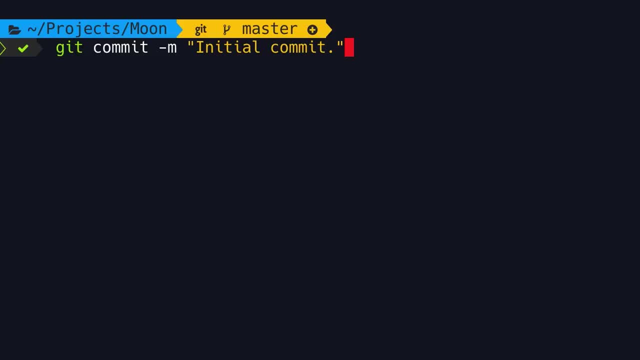 on a bug and there were some constraints at the time you committed your code. you may want to explain those constraints. This is very valuable to both you and your co-workers. So in situations like this, we drop the message, we just type git. 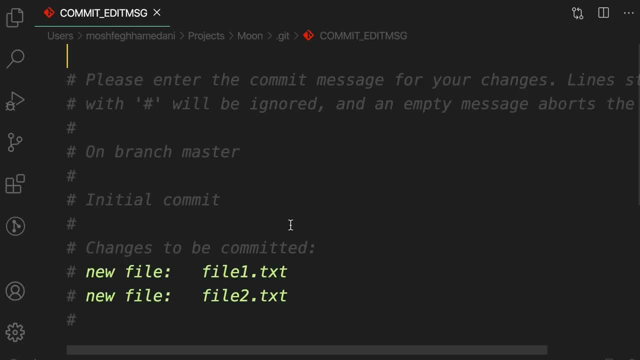 commit. Now, when we press enter, this opens our default editor, in this case vs code, because at the beginning of the course I configured my default editor to be vs code. Okay, So here we're trying to edit this file: commit. 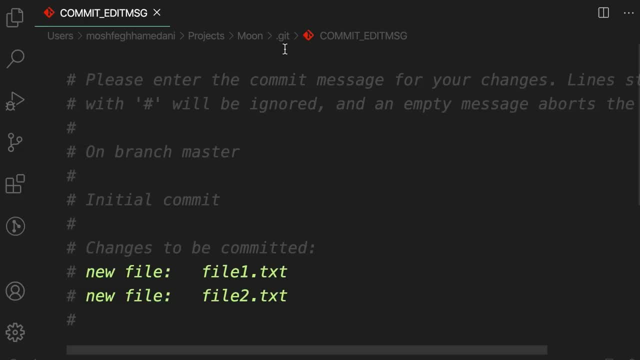 underline edit message, which is stored in our git sub directory. So on the top we can type a short description- ideally this should be less than 80 characters- then we add a line break and after that we can type a long. 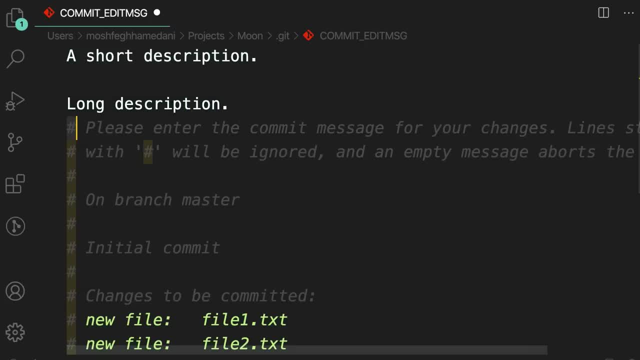 description. Now these lines that start with a pound sign are comments. they're going to get ignored, So we type whatever we want here. in this case, I'm going to say initial commit and this is our first commit. Of course this is repetitive. we don't want to have commit. 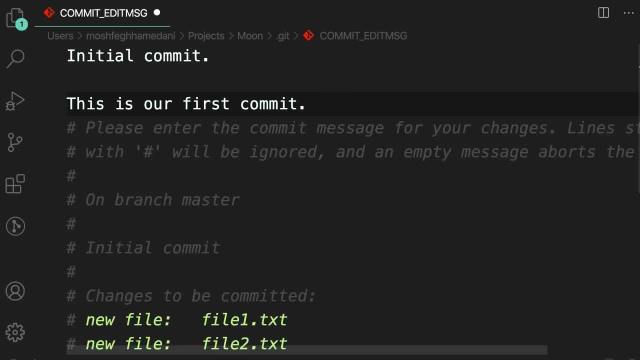 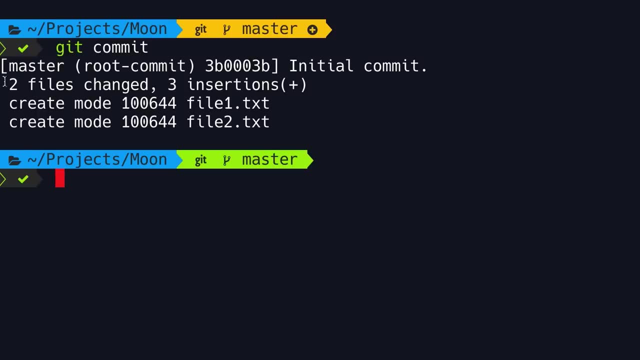 messages like this, but for this demo I'm going to go with this message. So we save the changes, then we close this window back in the terminal, our snapshot is committed and here we have basic statistics about what was changed. So 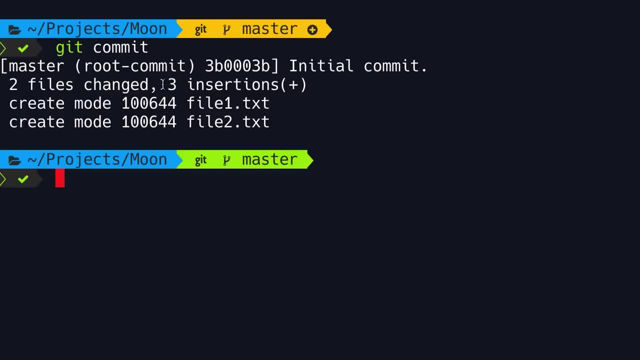 two files were changed, which are file 1 and file 2, and we have three insertions. three lines were inserted. In file 1, we insert two lines- hello world- and in file 2, we inserted one line. Now look at this indicator. it turned. 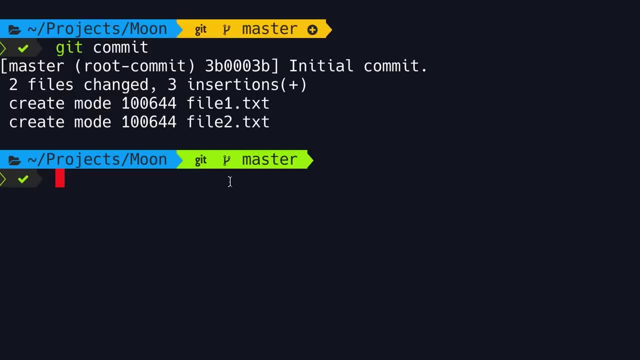 green because our working directory is now clean. it doesn't have any new changes, So what we have in our working directory is exactly the same content we have in our staging area, which is exactly the same content we have in the last commit. 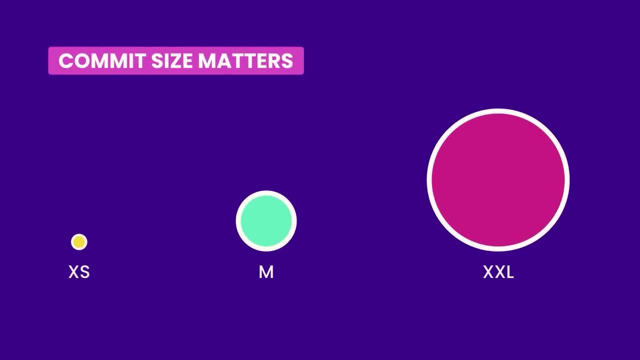 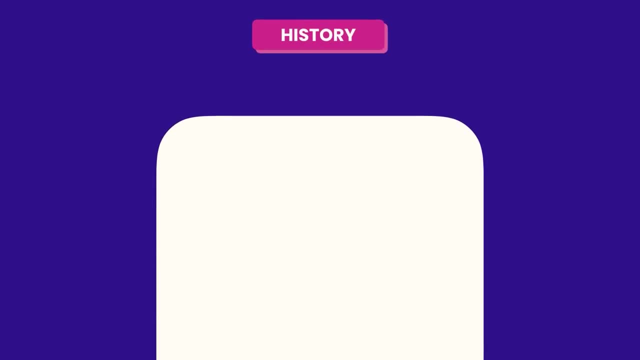 Let's talk about the best practices for committing code. First of all, your commit shouldn't be too big or too small. We don't want to make a commit every time we update a file. that's just useless because we'll end up with commits. 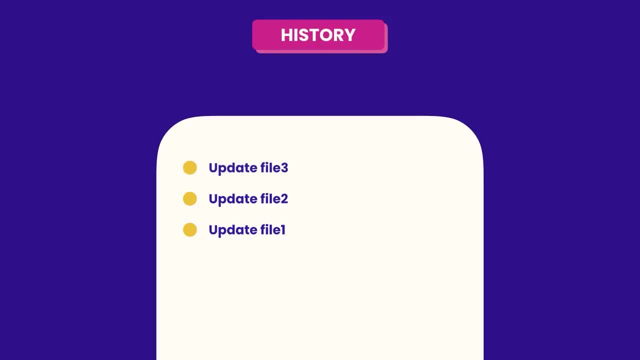 like update file 1,, update file 2,, update file 3, it's just useless. On the other hand, we don't want our commits to be too big. we don't want to wait and implement a feature end to end before committing it. 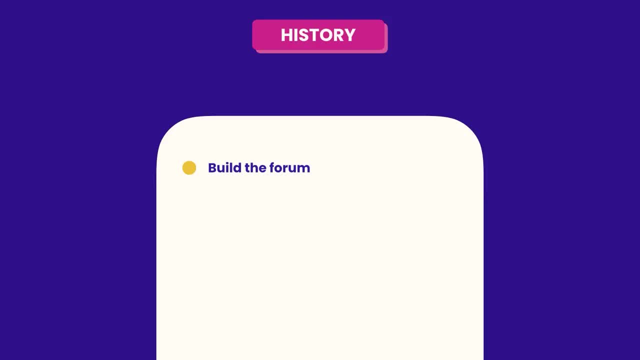 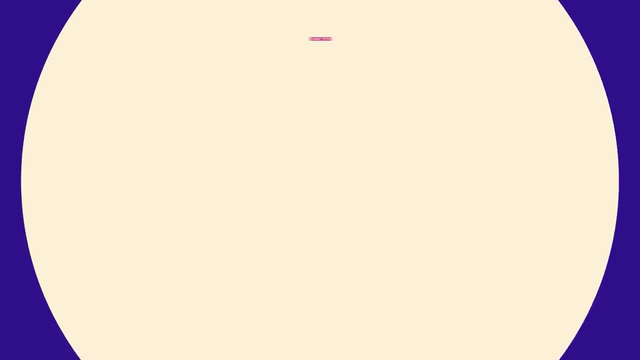 We don't want to code for three days and then make a commit, because the whole point of committing is to record checkpoints as we go. So if you screw up we can always go back and recover our code. So try to commit often. 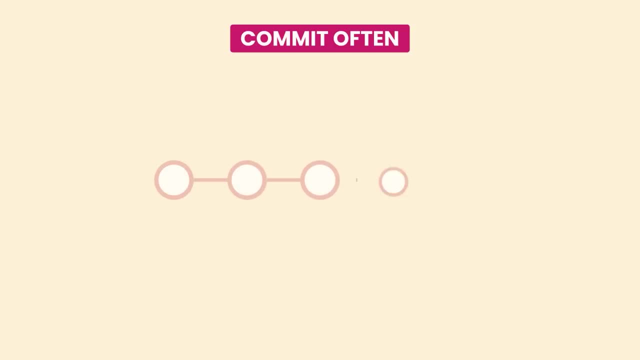 In the real world you might commit 5 to 10 times a day, or even more, depending on the kind of work you are doing. But this is just a basic guideline. Don't take it as a rule. Don't try to aim. 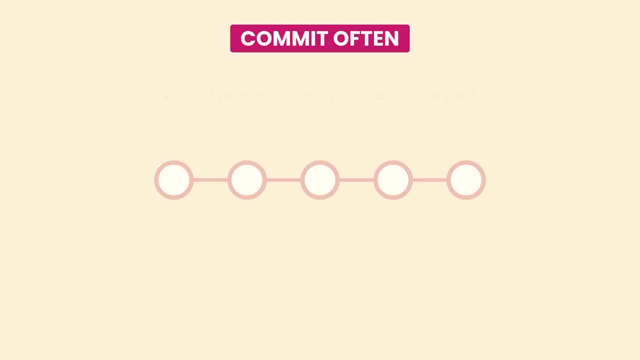 for 5 or 10 commits a day. So as you're coding, as you reach a state you want to record, then make a commit. Also, each commit should represent a logically separate change set, So don't mix things up. For example, if you're fixing a bug, 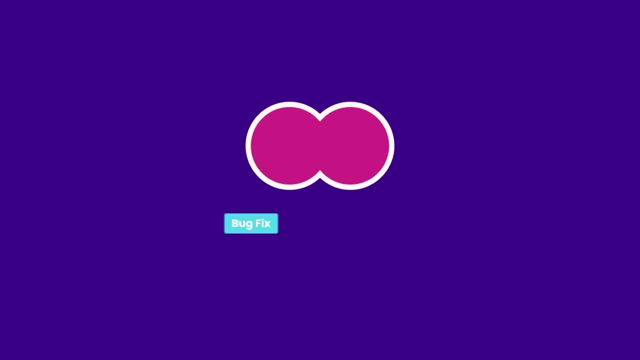 and then you accidentally find a typo in your app. you shouldn't commit both these changes in one commit. You should have two separate commits: One commit for the typo, another one for the bug fix. Now, if you accidentally stage both these changes, 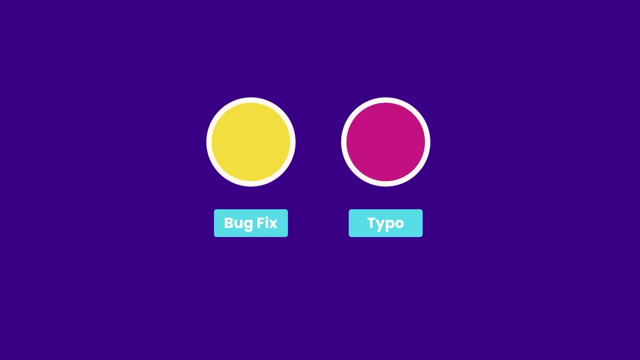 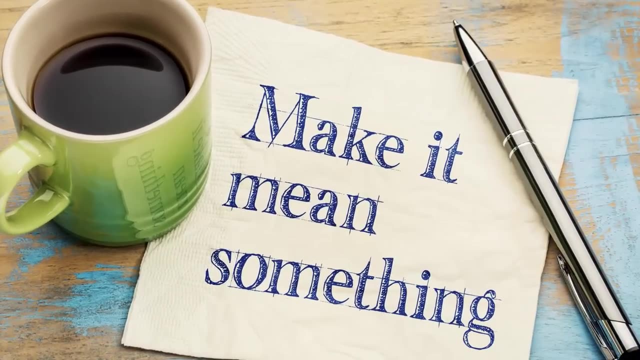 you can easily unstage them. I'll show you how to do this later in this section. Next, you should give yourself the habit of creating meaningful commit messages, Because all of these messages are going to show up in history. So if your messages are cryptic, 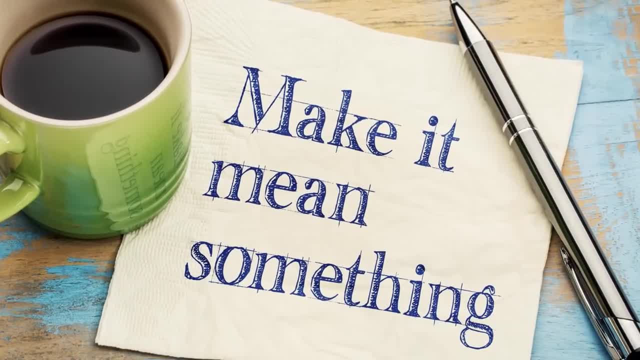 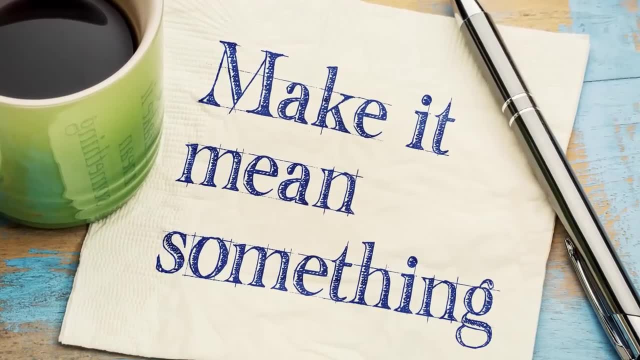 they're not going to be helpful to you or other team members. If you followed my previous advice, if your commit represents a single unit of work, it would be easier to come up with a message for your commit If you're doing too many things. 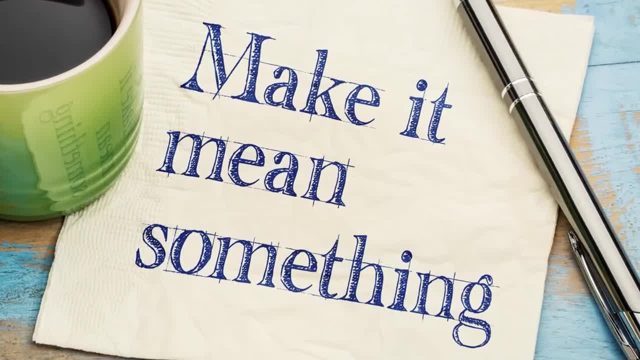 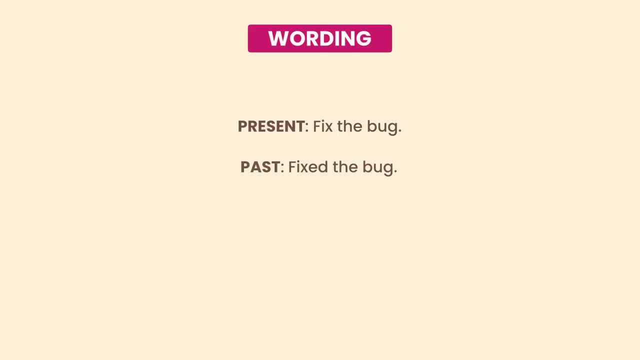 in one commit, you're not going to come up with a good message. Okay Now, in terms of the wording, most people prefer to use the present tense in their commit messages. So instead of fix the bug, you should say: fix the bug If you don't like this convention. 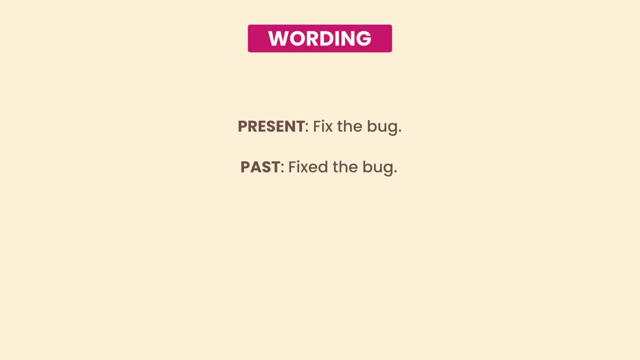 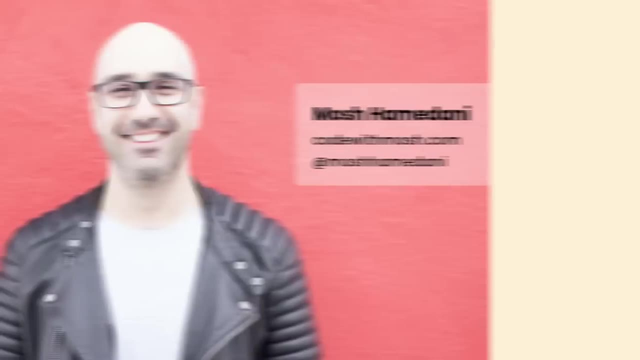 that's totally fine, but whatever convention you use, make sure that you and other team members stick to it. So always take these best practices in mind when committing code. Hey guys, Mosh here. I just want to let you know that this video you've been watching is actually 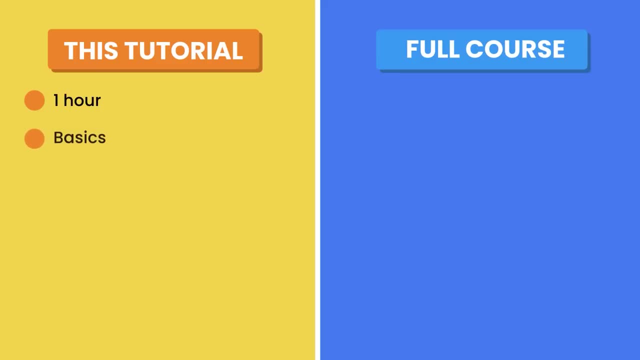 the first hour of my complete Git mastery course and covers only the basic stuff. So after you finish this video, if you want to learn more, take a look at my full course. The complete course is 5 hours long and covers intermediate to advanced level concepts. 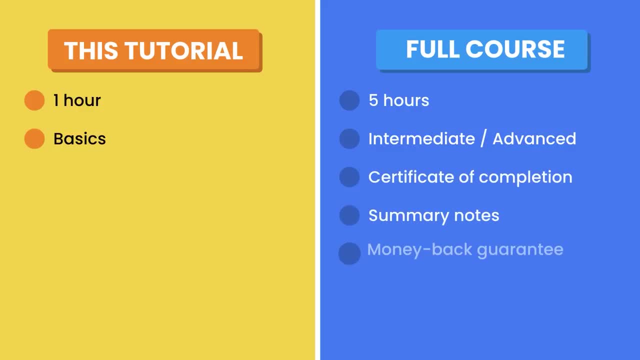 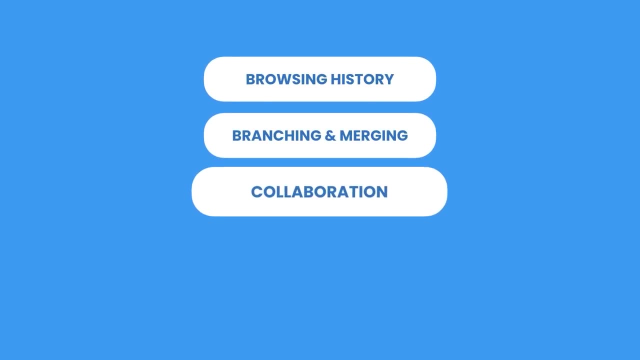 It comes with a certificate of completion, downloadable summary notes and a 30 day money back guarantee, So if you're not happy, you can ask for a refund. You will learn all about browsing history, branching and merging, collaborating with others using Git and GitHub and rewriting history. 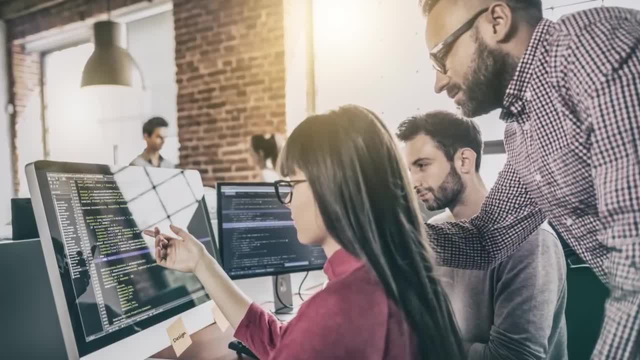 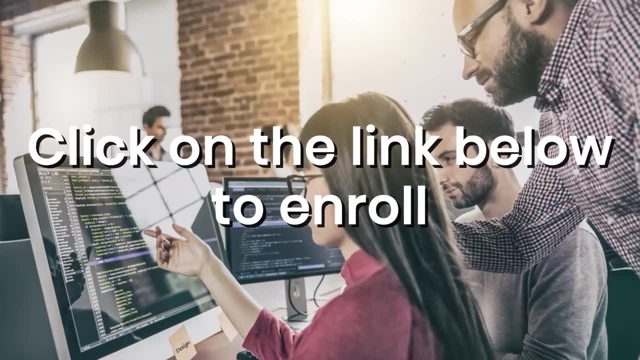 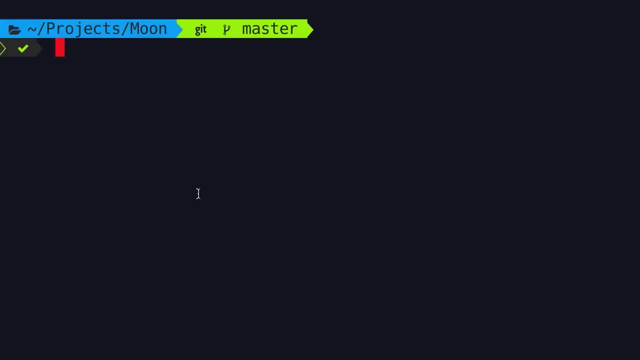 So by the end of this course you would be able to use Git like a pro and work effectively with others in your team. If you're interested, click on the link below this video to enroll. One of the common questions a lot of beginners have is: 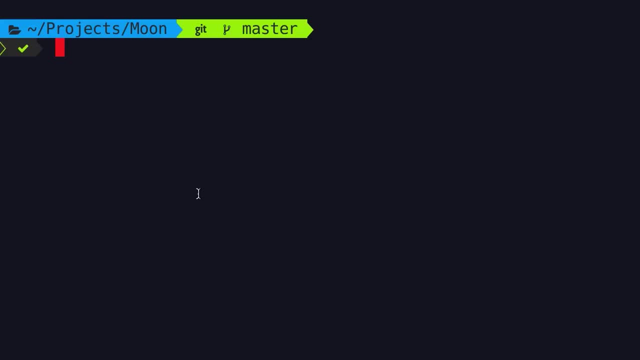 do we always have to stage our changes before committing them? Well, the answer is no, And in this video I'm going to show you how to skip the staging area. But do this only if you know what you're doing, If you're 100% sure that. 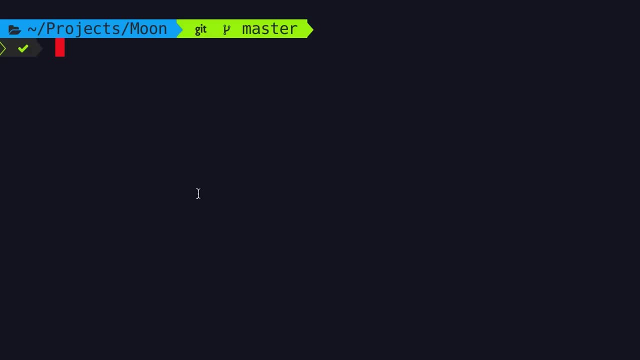 your code. your changes don't need to be reviewed, because that's the whole point of having a staging area. So let's modify file 1, and then commit it in one step. We're going to say echo test to file1.txt. 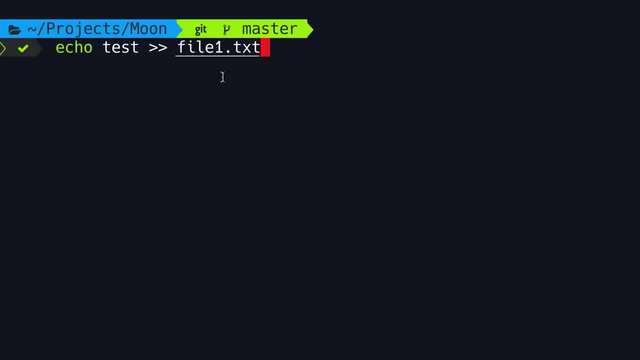 Once again, we're appending this line to file1.txt. okay, Alright, now we have a yellow indicator because our working directory is dirty. So instead of running git add and then committing it in two steps, we're going to commit. 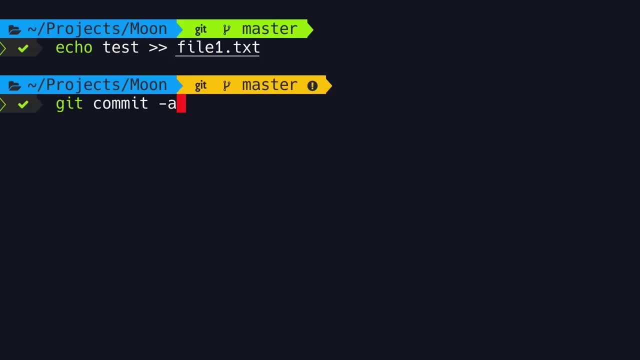 here we're going to supply the option dash a, which means all that means all modified files, And then, just like before, we supply a message, or we can combine these two options. So let's supply a message, fix the bug that. 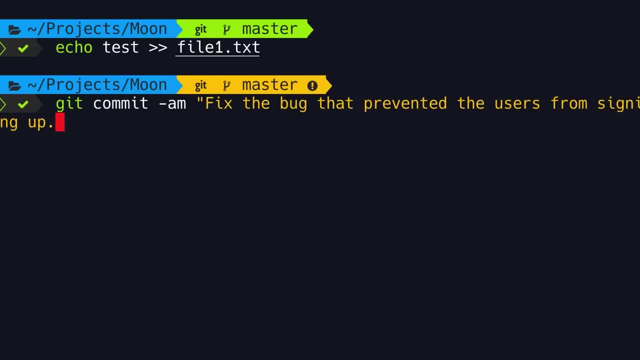 prevented the users from signing up. Let's go. our code is committed, one file was changed and we have one insertion, So this is how we can skip the staging area. But, once again, do this only if you know what you're doing. 99%. 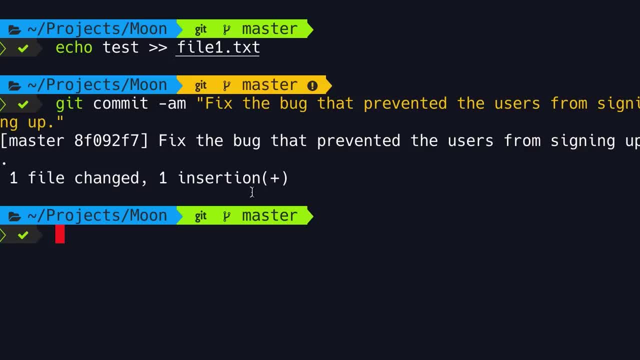 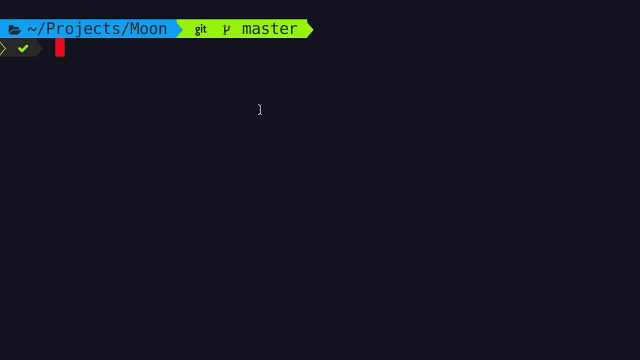 of the time. you should always stage your code before committing it to the repository. Let's say that we just discovered that we no longer need file2 in our project because it contains unused code. So to remove this file, we type: 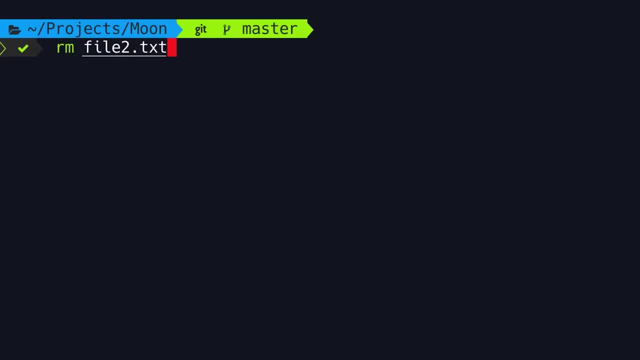 rm- file2.txt. Again, this is not a git command, because it doesn't start with git. it's just a standard unix command. okay, So let's go with this. Now we have a yellow indicator, which means our working directory is dirty, so let's. 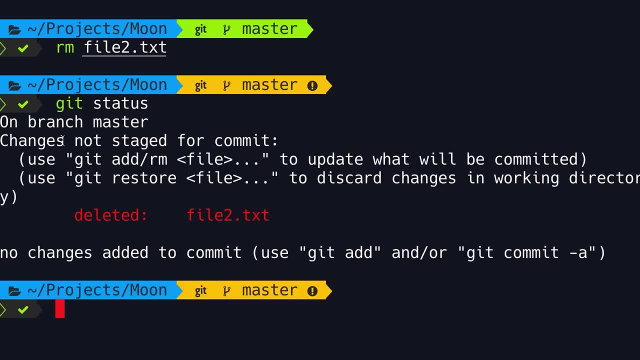 run git status. We have a one change that is not staged for commit. So we remove file2 from our working directory, but it still exists in the staging area. Let me prove it to you. So we type git: ls-files. 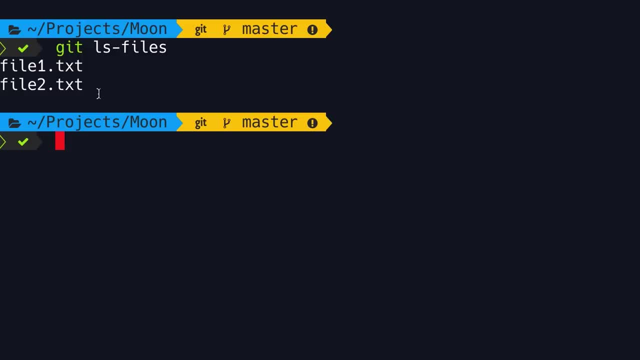 these are the files in our staging area. So file2 is still here, even though we removed it from our working directory. So, as I told you before, every time we make changes, we have to stage those changes using the add command. 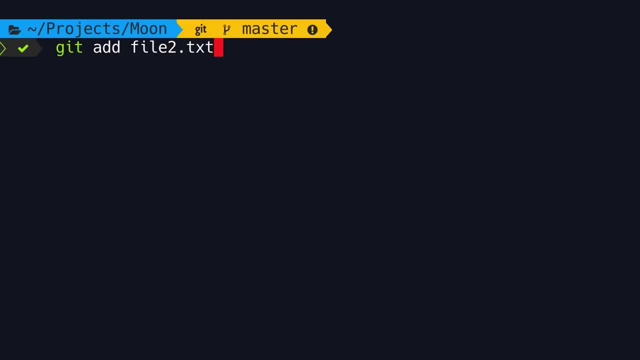 So here we type git add file2.txt to stage this change or this deletion more accurately. Now let's run git ls-files one more time. So file2 is no longer in the staging area. Beautiful, Let's run git status. 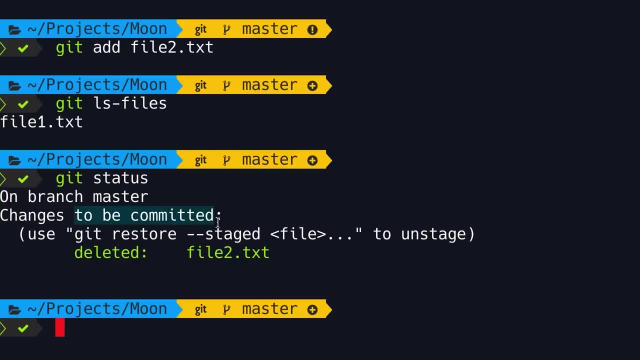 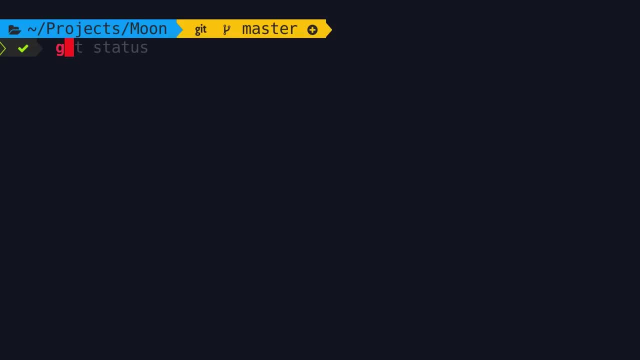 We have one change that is ready to be committed and, as you can see, it's indicated by green, which means it's in the staging area. So let's commit this change. and here we're going to say: remove unused code. 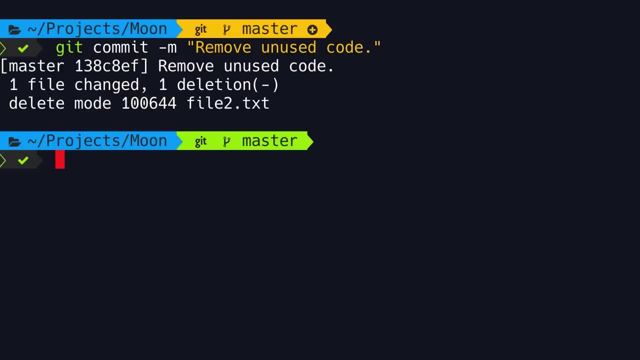 So to remove unused code, so to remove a file, we have to remove it from both our working directory as well as the staging area, Because this is a very common operation. git gives us a command that does both of these steps in one go. Let me show you. 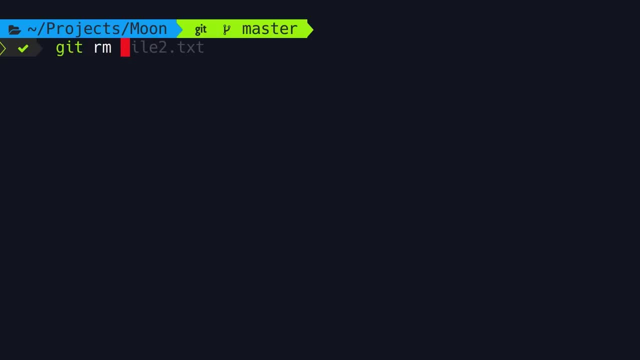 So we type git rm. so instead of using the standard rm command in unix, we use git rm. Here we list a file name like file2.txt. we can also specify multiple files. we can also use patterns, like all text files. 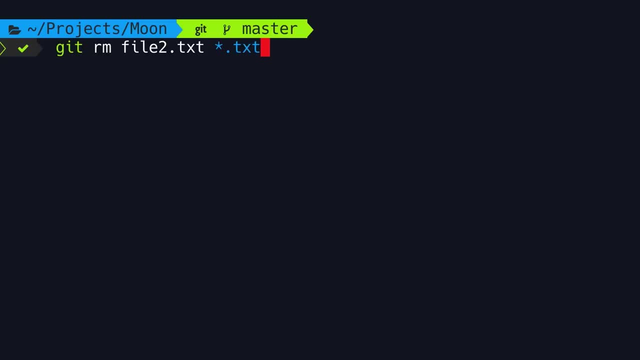 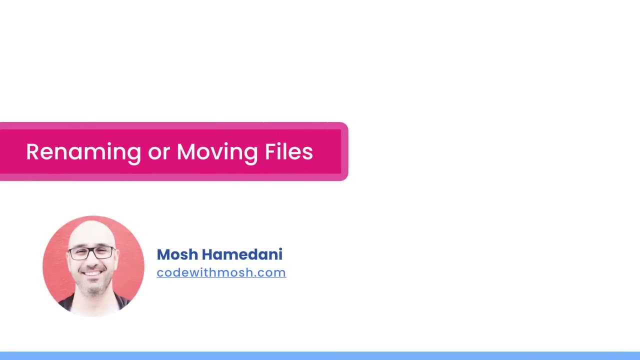 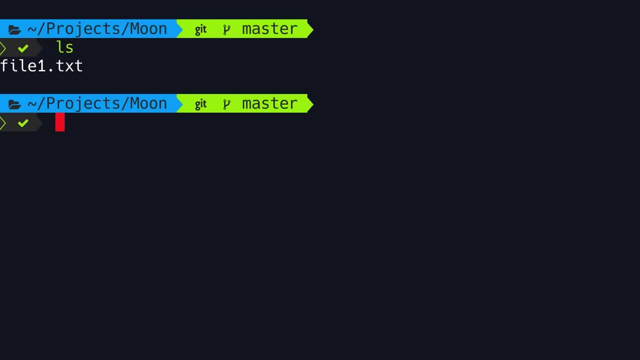 When we execute this command, we can see that git removes this file from both the working directory as well as the staging area. Now let's talk about renaming, or moving files. So currently we have a single file in our working directory and that is file1.txt. 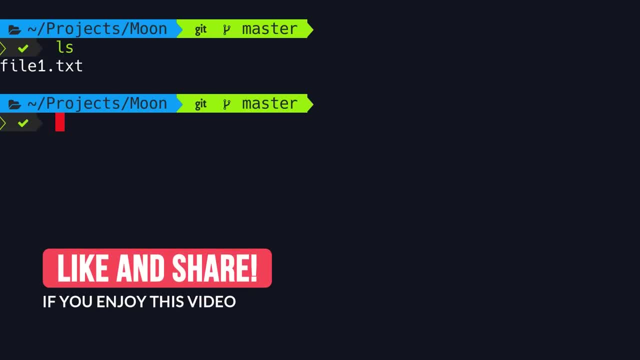 Let's rename this to mainjs. So we use the move command in unix to rename file1.txt to mainjs. So with this command we can rename or move files and directories. Okay, Now our working directory is dirty, so 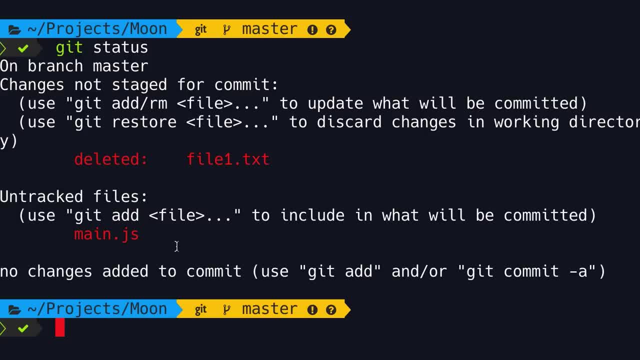 let's run git status. We have two changes and both these changes are unstaged Because they are indicated by red. We have a delete operation, we deleted file1.txt and under untracked files we have a new file. So, as you saw at the beginning, 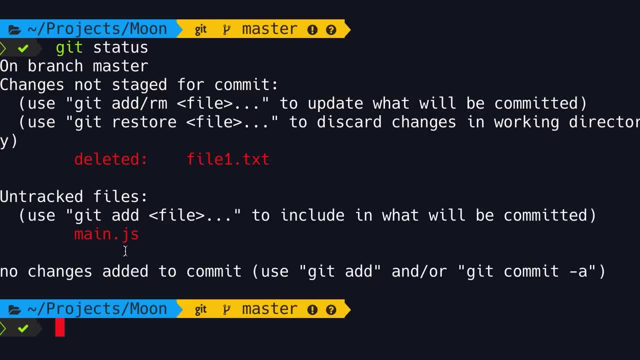 of this section. git doesn't automatically track all your new files. Every time you have a new file in your project, you have to add it to the staging area, so git starts tracking it. So once again we have to use the add command to stage. 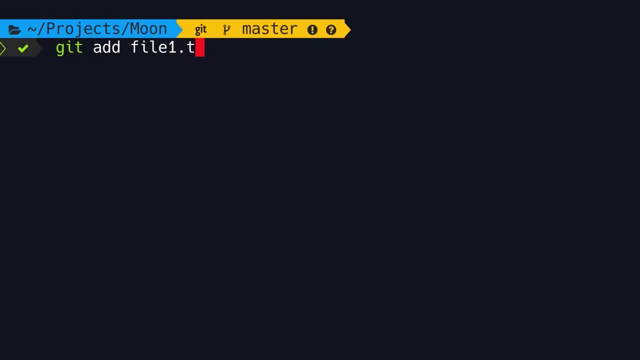 both these changes. git add file1.txt. this is for staging the deletion. and now let's add the new untracked file, mainjs. Now let's run git status one more time. look, git recognizes that we renamed file1.txt. 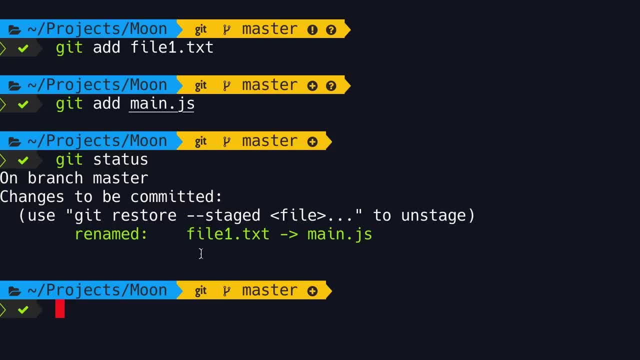 to mainjs, And this item is indicated by green, which means this is in the staging area. So renaming, or moving files, is a two step operation. First we have to modify our working directory and then we have to stage two types of changes. 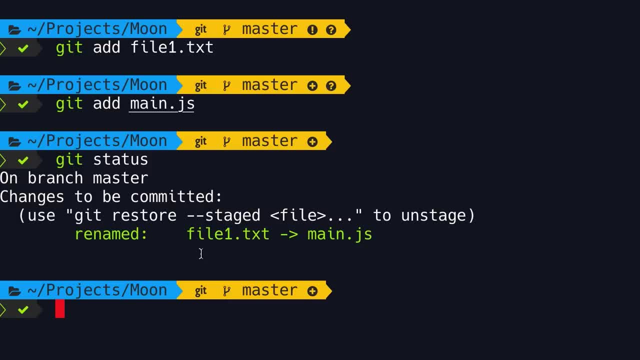 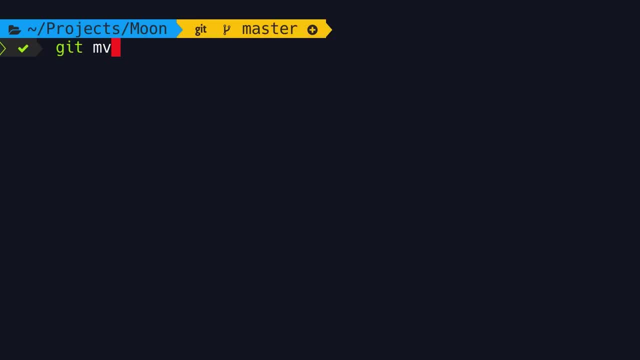 an addition and a deletion, So similar to removing files. git gives us a special command for renaming or moving files, That is git move. So instead of using the standard move command in unix, we're going to use git move. Now let's rename. 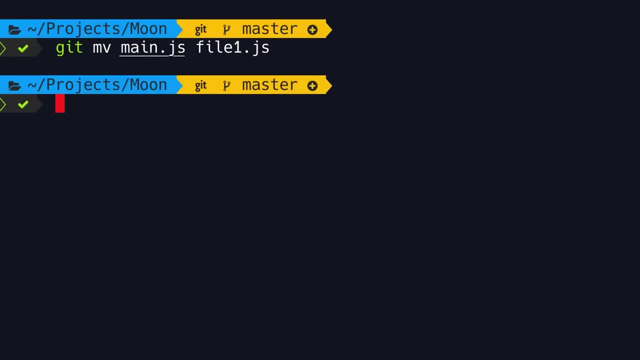 mainjs to file1.js And then run git status one more time. so we have a rename operation for renaming file1.txt to file1.js. So when we use the move command the changes are applied to both the working directory and the staging area. 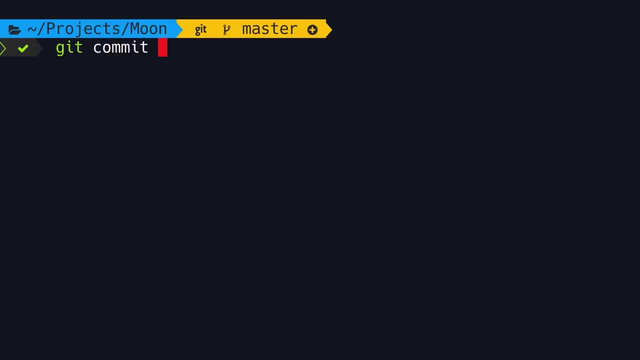 Now let's commit the changes for the message. I'm going to say refactor code. Now look at the statistics. one file was changed. we have zero insertions because we haven't added any new lines to any of our files, And we also have zero deletions. 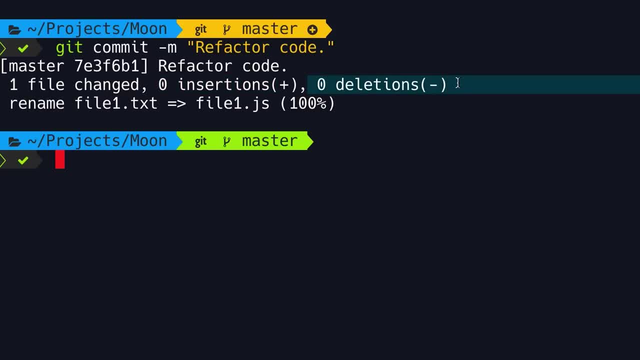 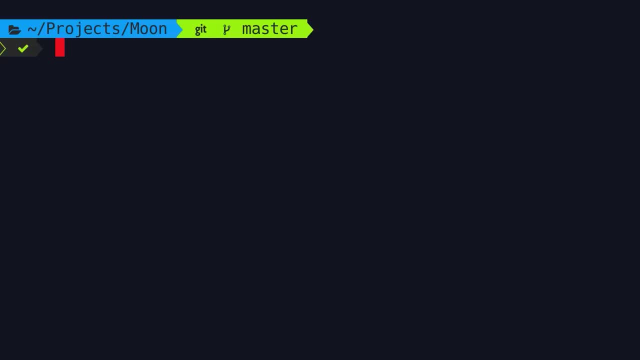 because we haven't removed any lines from any files. Now let's look at the. in almost every project, we should tell git to ignore certain files and directories. For example, we don't want to include log files or binary files that get generated. 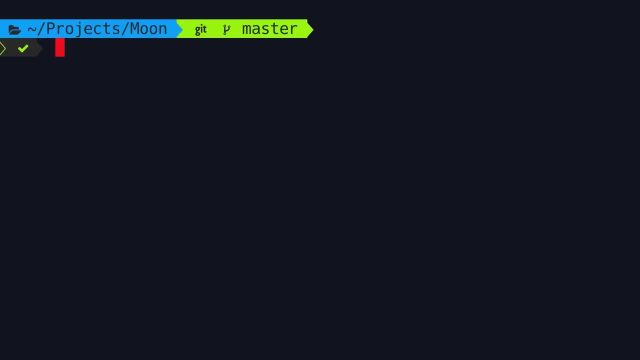 as a result of compiling our code. Adding these files is just going to increase the size of our repository without providing any values. Every developer can have their own log files, right. So log files are not something we want to share and synchronize with other team members. 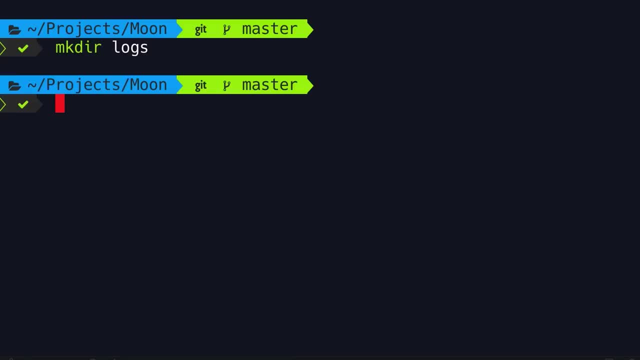 So for this demo, let's create a directory called logs and then add a log file here. Once again, we can use the echo command to write hello to logs. slash dev dot log. Now let's run git status. so git is saying that: 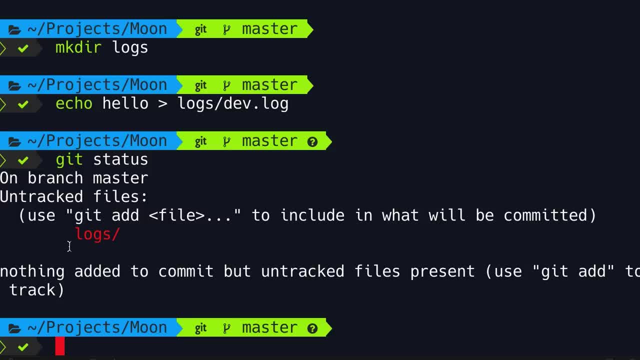 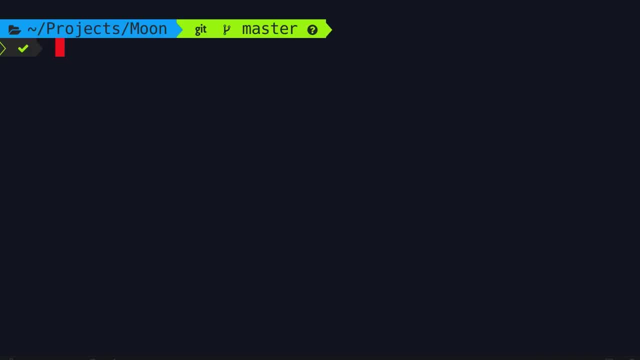 we have an untracked directory called logs, but we don't want to add this to the staging area because we don't want git to track this. So to prevent this we have to create a special file called dot git ignore. So this file has no name. 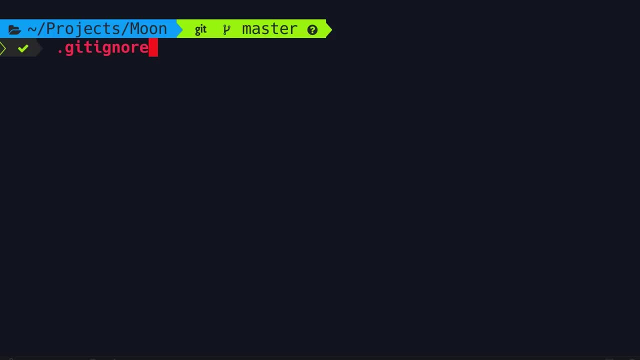 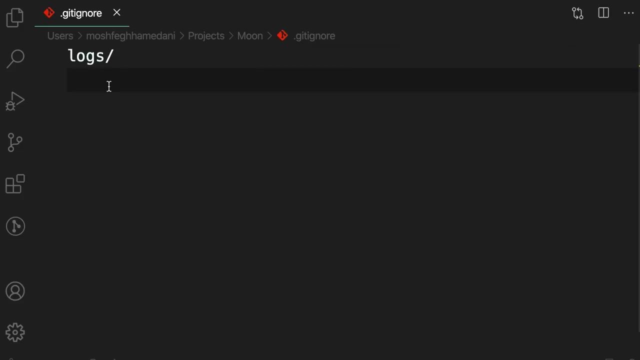 it only has an extension and it should be in the root of your project. So let's echo logs forward. slash two dot git ignore. Now I'm going to open this file using vs code, so code git ignore. so in this file we have a single entry. 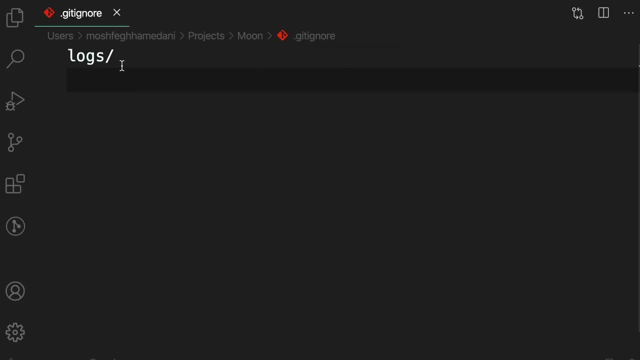 logs forward. slash, which indicates a directory. We can list as many files and directories we want here. For example, we can include main dot log. we can also use patterns like all log files, and so on. Once we are done, we save the changes. 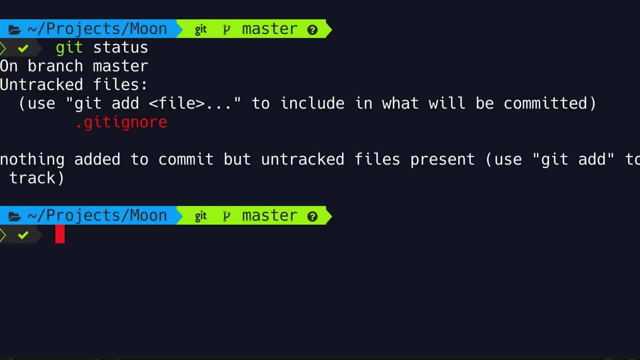 back in the terminal. now we can if you run git status one more time. git no longer says that we have a new directory called logs, because it's ignoring it. Instead it says we have a new file called dot. git ignore. So let's add this. 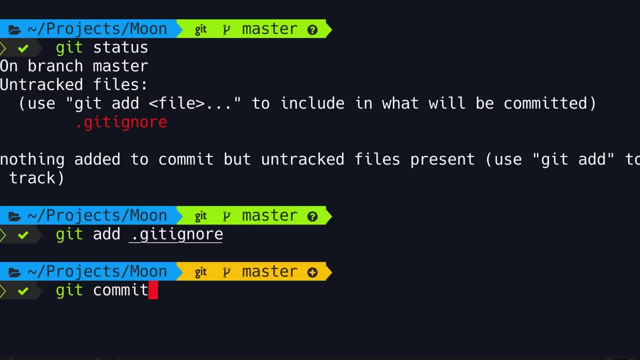 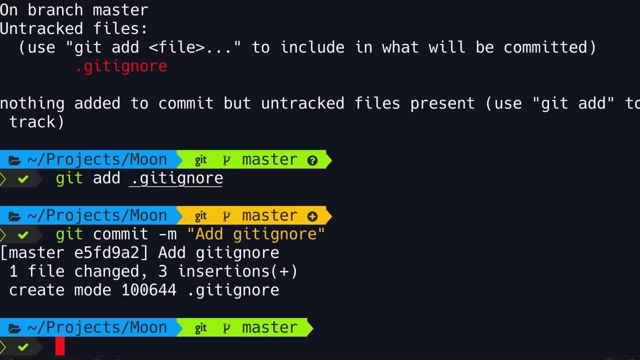 file to the staging area and then commit our code. So add git, ignore. So this is how we can ignore files and directories in git. Just remember this only works if you haven't already included a file or a directory in your repository. 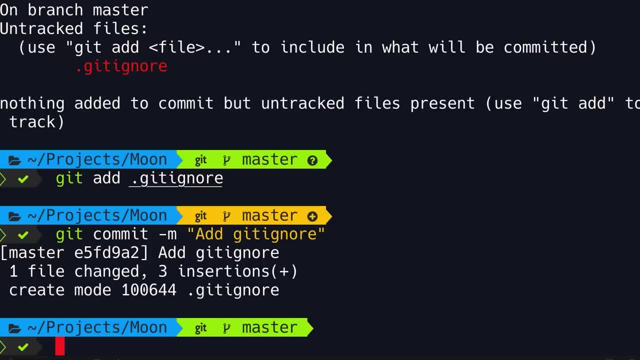 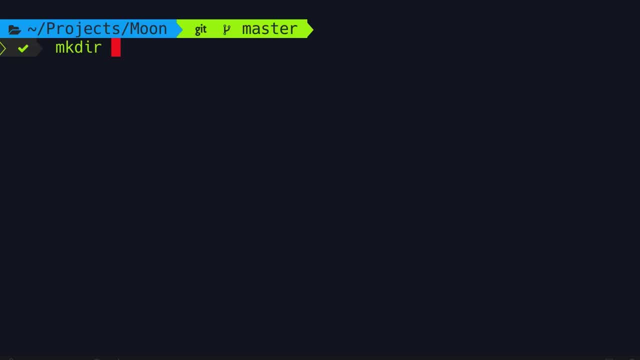 In other words, if you have a directory and accidentally include a file in your repository and then later add it to git, ignore git is not going to ignore that. Let me show you. So let's create a new directory called bin. 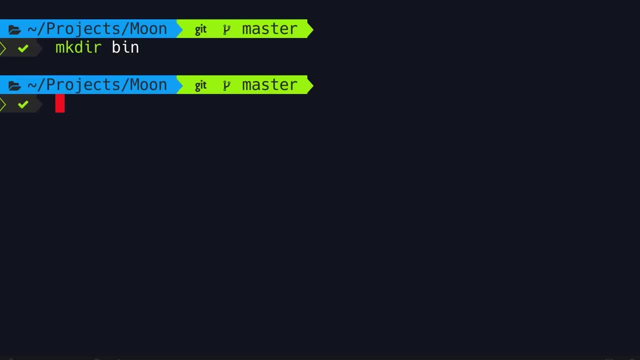 Let's imagine that this directory contains our compiled source code. So, using the echo command, I'm going to write hello to bin slash app dot bin. Now let's run git status. So we have a new directory. now we want to accidentally commit this to our repository. 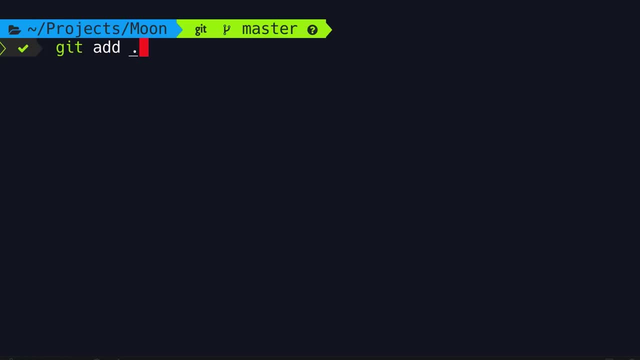 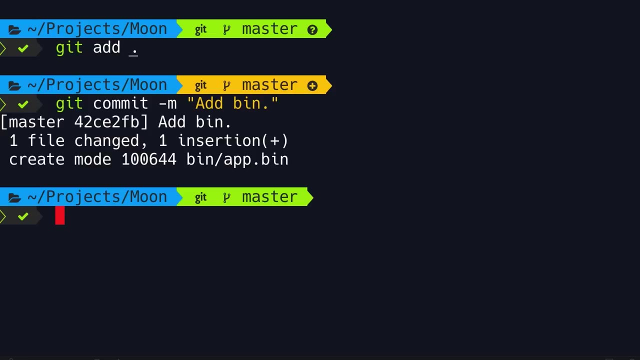 So we add all the changes and then commit our code Add bin. Here's the problem. every time we compile our code, git is going to say that this file, bin slash, app, dot bin- is changed. so we have to stage it and then commit it. It doesn't. 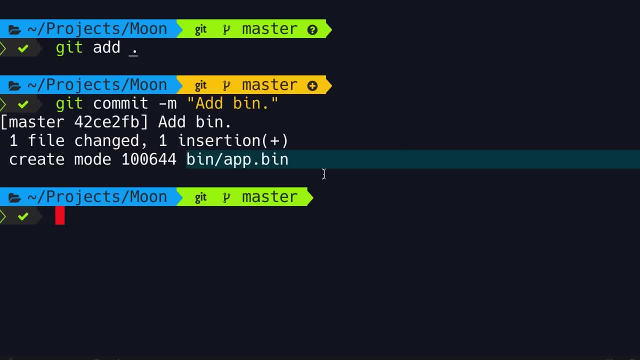 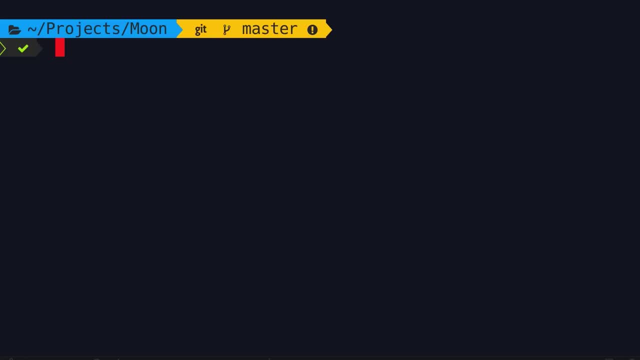 make sense. Why do we have to commit this file every time we compile our application? So back to git. ignore, let's add the bin directory here as well. Now back in the terminal, let's run git status. so we have modified git. ignore, beautiful, let's stage. 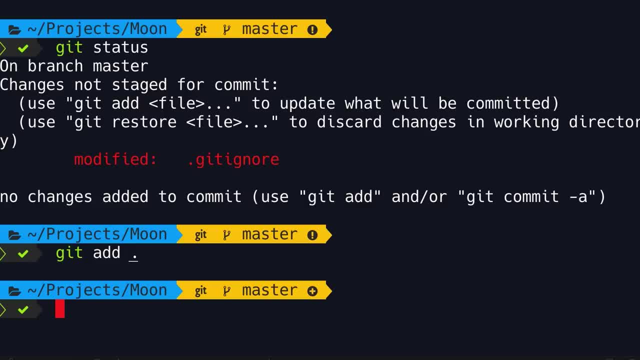 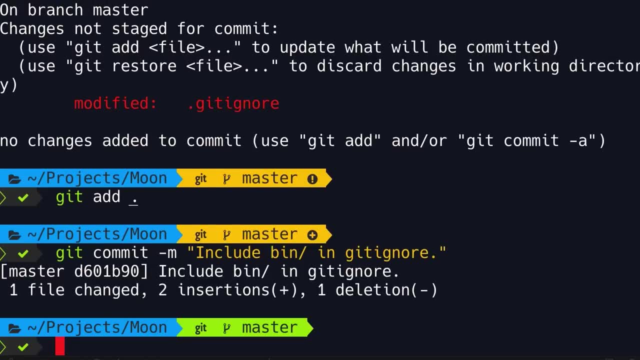 and commit this change. so git add period and then git commit, include bin slash and git ignore. Now, in this case, git is not going to ignore the changes in this directory because it's already tracking this directory. So let's modify our bin. 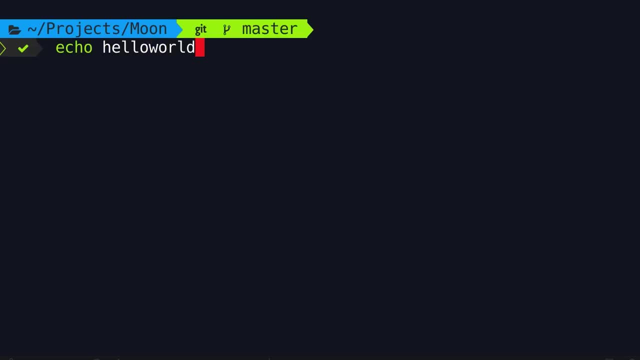 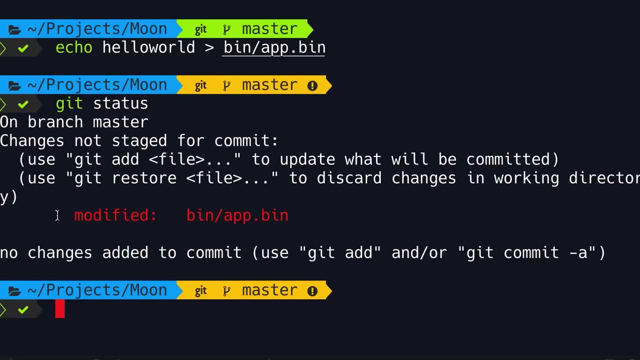 file by saying: echo, hello world to bin slash app dot. bin Git status. look, git is saying that this file is modified. This is not what we want. To solve this problem, we have to remove this file from the staging area, which is what we're. 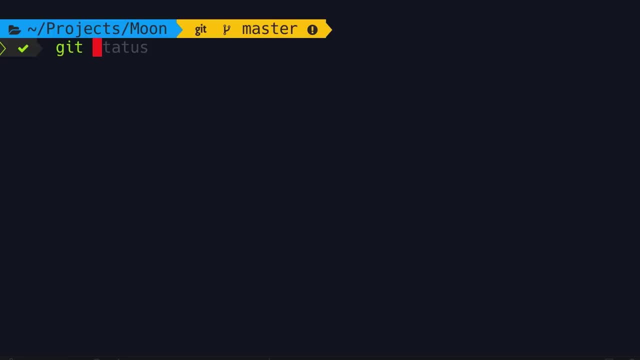 proposing for the next commit. So earlier we talked about git ls dash files. This command shows the files in our staging area. So, as you can see, this bin file, or the bin directory, is already in the staging area. We should remove it here. How. 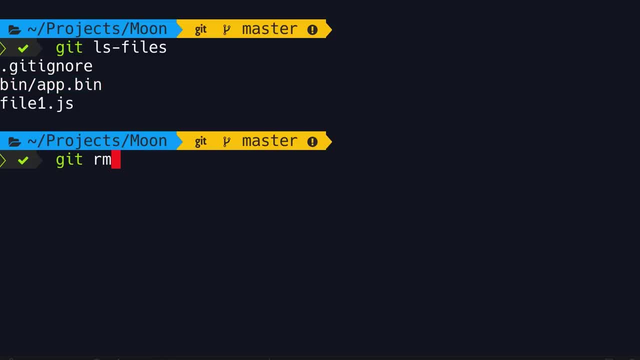 Well, earlier we talked about the git remove command. I told you that with this command we can remove a file or a directory from both the working directory as well as the staging area, But in this case we don't want to remove this file from our 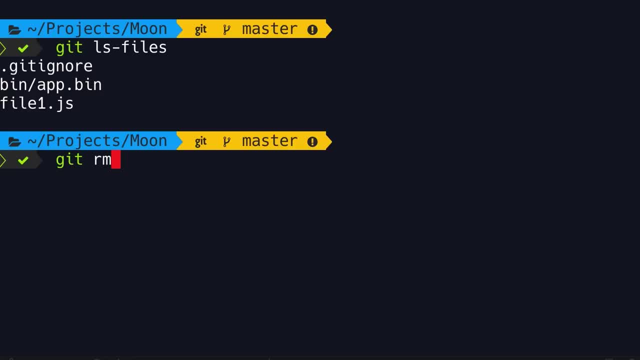 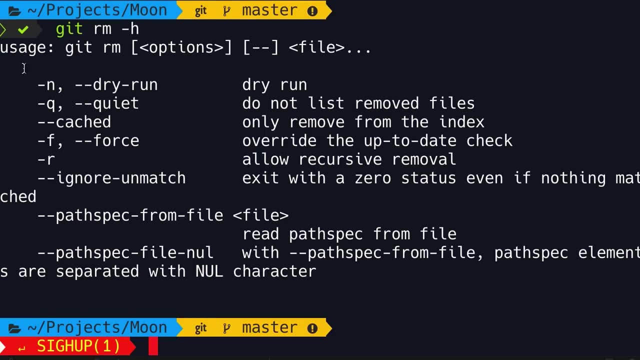 working directory, because that's how we launch our application. So we want to remove this file only from the staging area. How Well, let's add dash h for a quick help. So we type git rm, then we can add zero or more options. 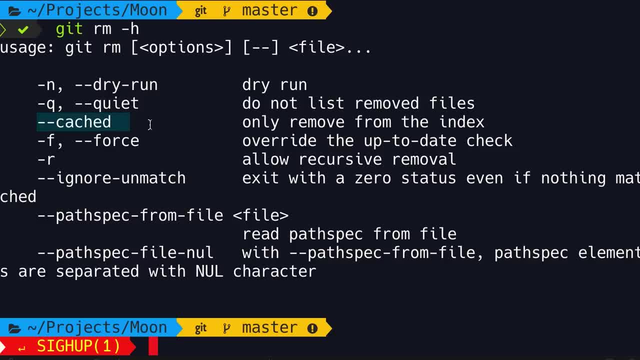 Now here we have this option called dash dash cache. With this we can remove stuff only from the index. Index is the old term for the staging area, So when you look at git documentation, most of the time you see index. So using this option, 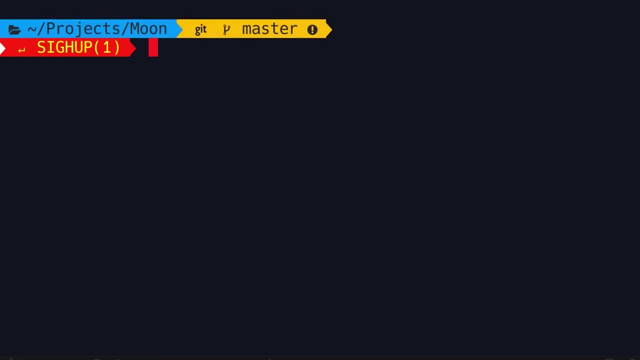 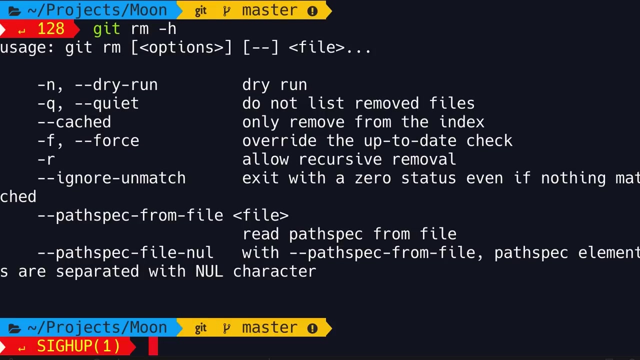 we can remove the bin directory from the index. So git rm, dash, dash, cache bin forward slash. Now we get an error saying not removing bin recursively without dash r. So one more time let's look at the help for this command We have. 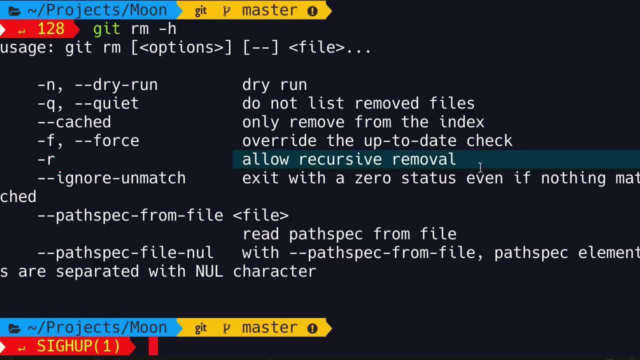 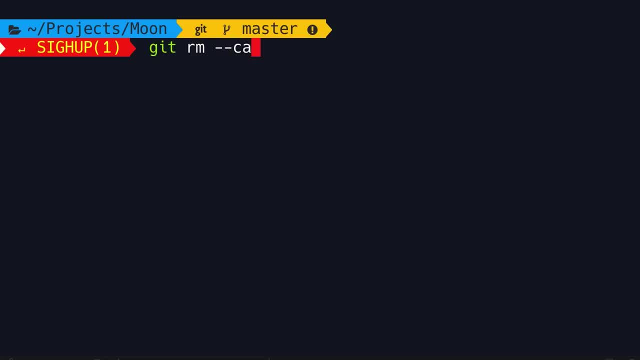 another option called dash r for recursive removal. So we want to remove the entire bin directory from the staging area. To do that we type: git rm dash dash cache, dash r bin forward slash. Beautiful, Now this entire directory is removed from the staging area. 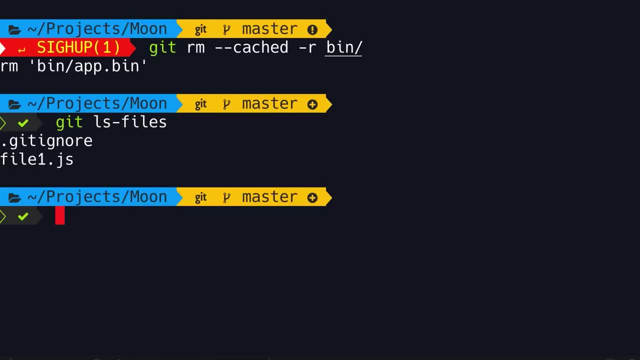 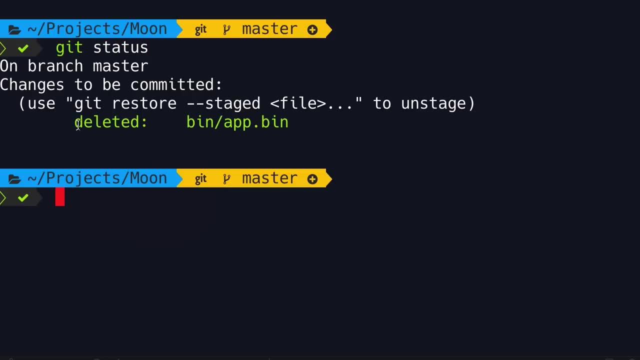 Let's verify it. So git ls files. our bin directory is no longer here. Now let's run git status. Look, we have one change that is ready to be committed. This directory is directly deleted from our staging area, So. 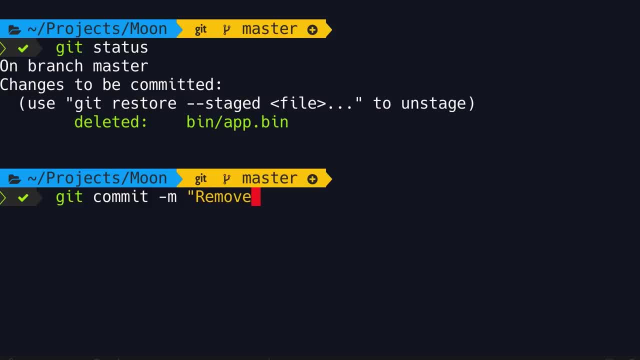 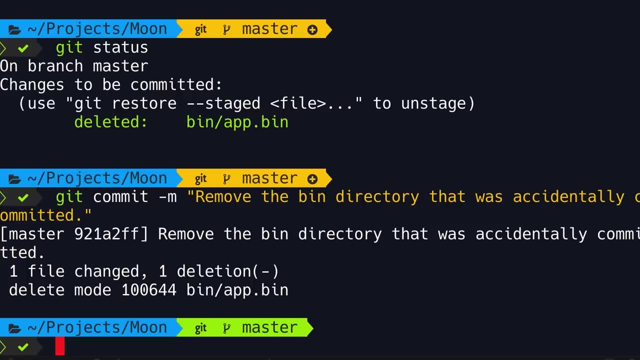 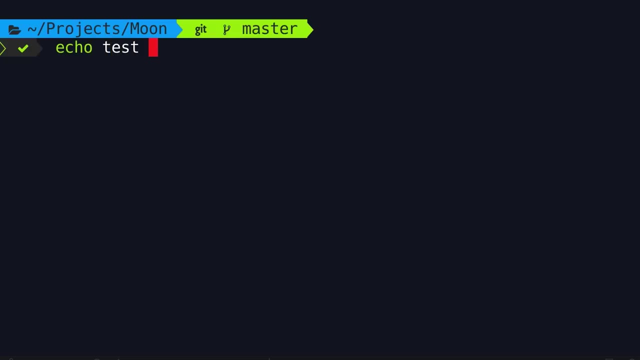 let's commit the change, remove the bin directory that was accidentally committed. Okay, from this point forward, git is no longer going to track the changes in this directory. So if we encode test to bin slash appbin, you can see our working directory. 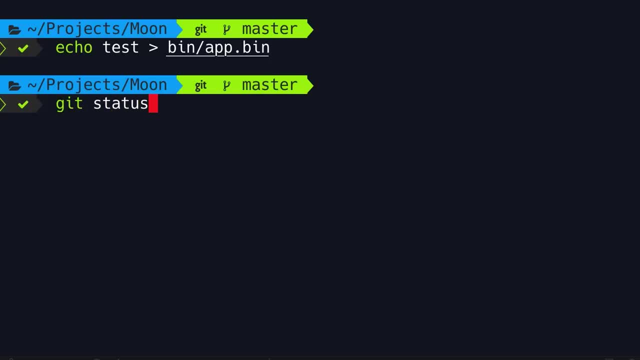 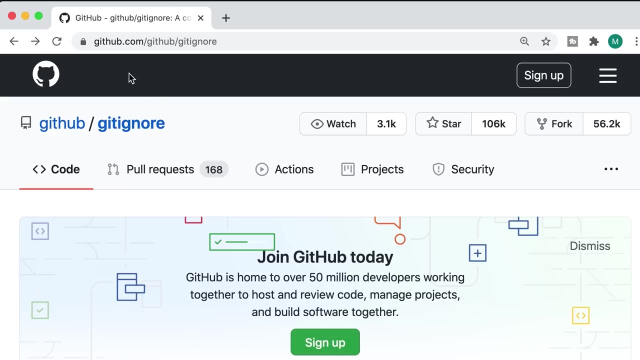 is still clean. we don't have any changes. we can verify it using git status as well. So this is how we can ignore files and directories in git. Now, if you head over to githubcom, slash, github, slash, gitignore, you can see various gitignore. 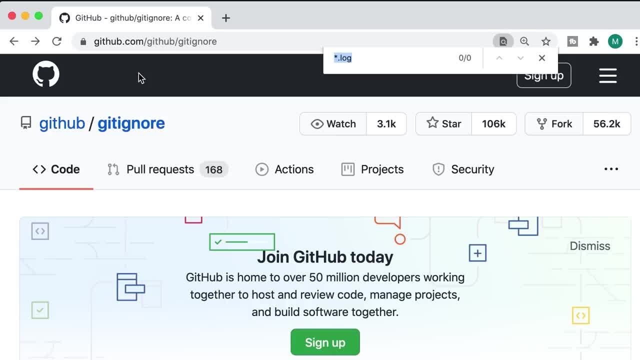 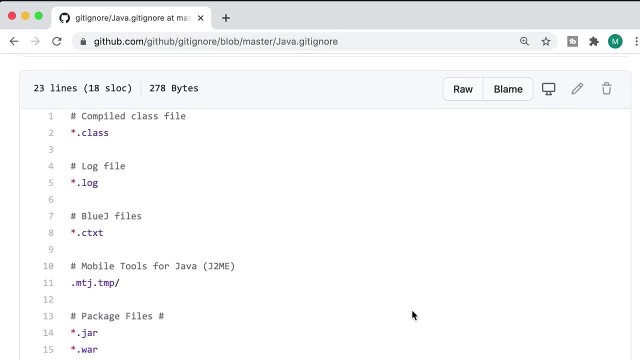 templates for different programming languages. For example, let's look at the template for java. So for java projects, it's a great idea to exclude all the class files, because these files get automatically generated when you compile your code, So there's no need to include them in your repository. 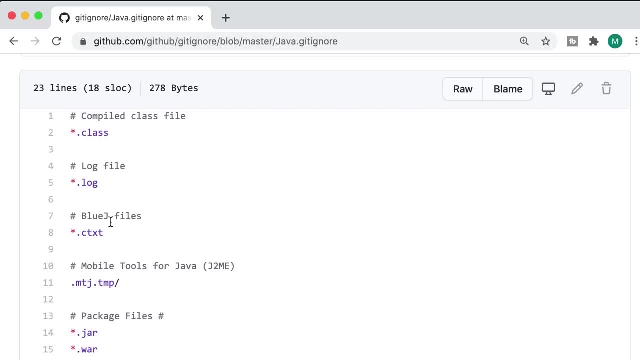 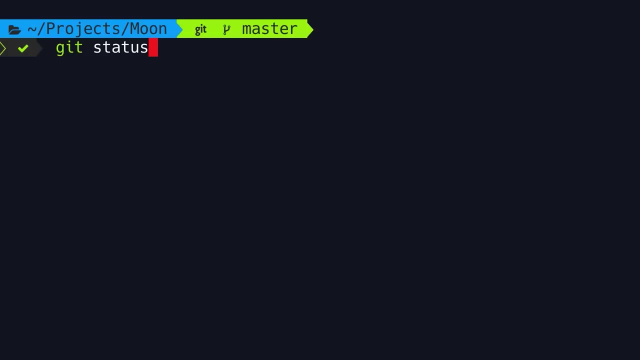 So here we have various patterns, like all the class files, or all the class files, all the log files, the lines that start with a hash sign. these are comments, so they get ignored by git. So you have learned how to get the status of the working directory. 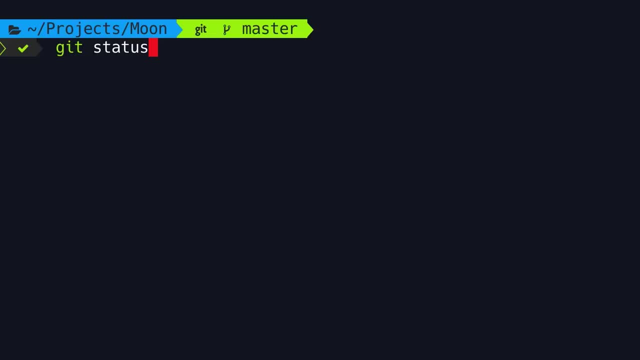 and the staging area using the status command. The output of this command is very comprehensive, but it's also very wordy, So as an alternative, we can supply the short status flag or dash s. Let me walk you through a few examples. So for this, 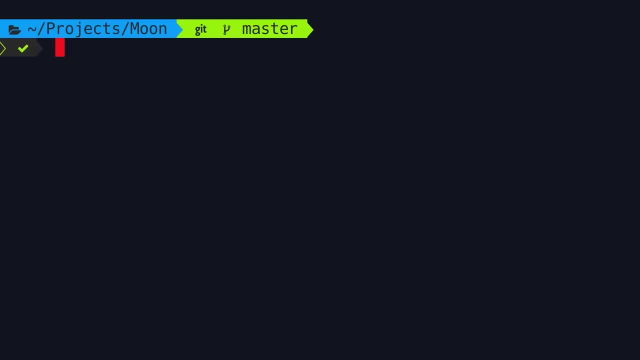 demo. we're going to modify one of our existing files and then add a new file. So echo sky to file1.js. So we're appending sky to file1.js. Now let's create a new file. so, once again, echo sky. 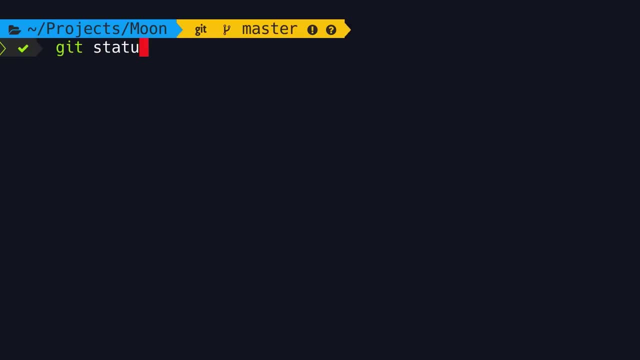 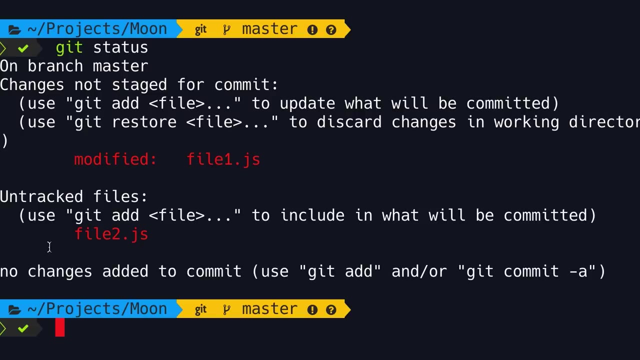 to file2.js. Now let's run git status. we have modified file1, and we have a new untracked file. So, as you can see, the output of this command is very comprehensive, but also very wordy. Now let's run. 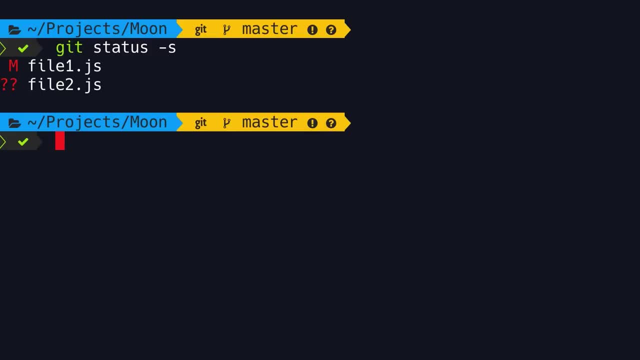 git status dash s. this is much easier to the eyes, So let me show you how this works. Here we have two columns: The left column represents the staging area and the right column represents the working directory. So we have modified file1,. 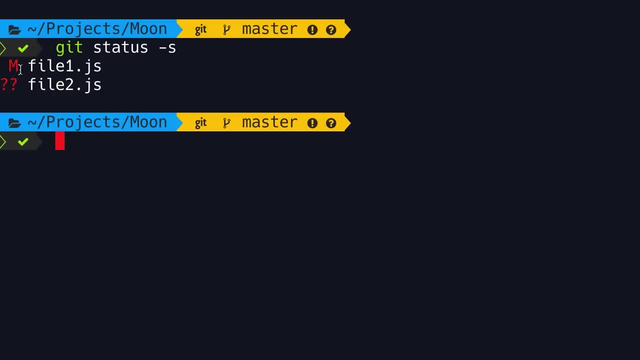 and that's why we have a red m in the right column, which is the working directory. So we have some changes here, but these changes are not in the staging area. That's why we don't have anything in the left column. Now. file2 is a new file. that's why we have 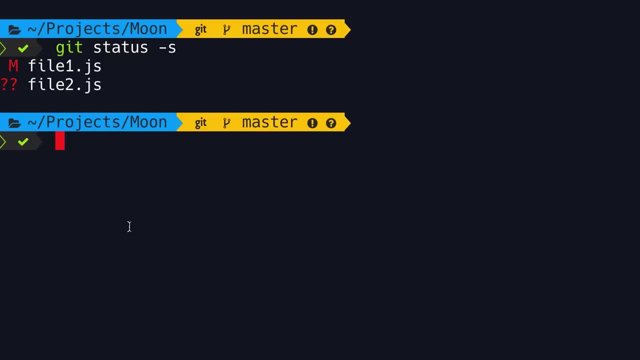 two question marks in both these columns. Now let's add file1 to the staging area. So git add file1, and then do another short status. Look for file1,. we have a green m in the left column or the staging area column. 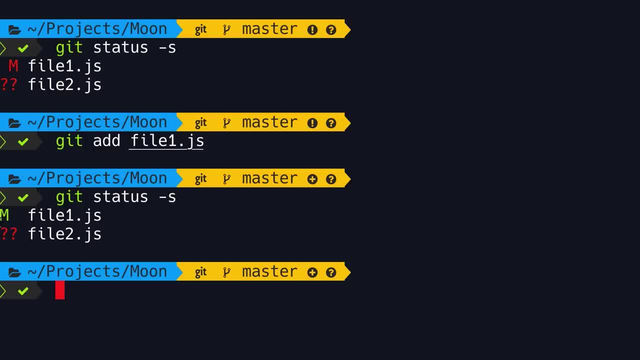 So all the changes that we had in the working area are now in the staging area In the right column. we don't have anything. we don't have any extra changes Now. earlier in this section I told you that when you stage a file, git takes a snapshot. 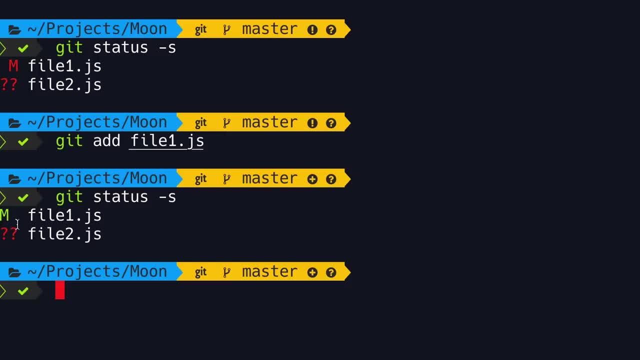 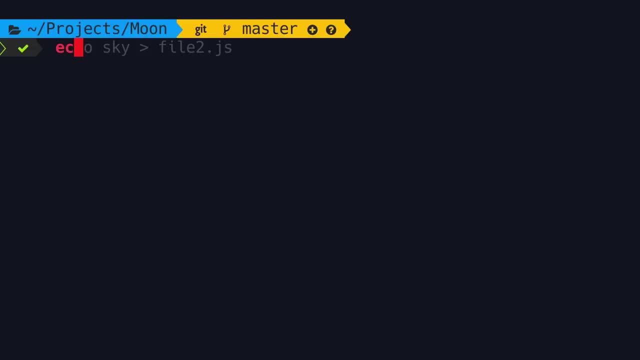 of that file and puts it in the staging area. So if you modify that file after, you have to restage the changes. Let me show you this one more time. So I'm going to modify file1 one more time. Let's echo ocean. 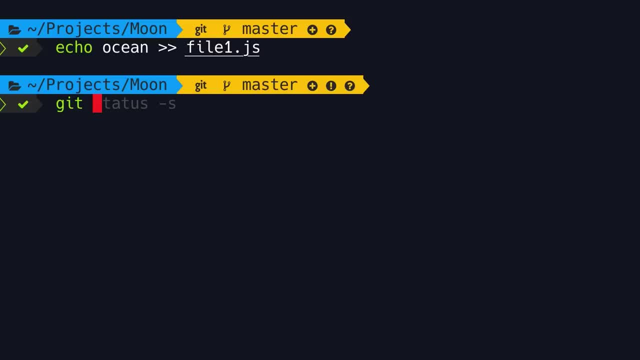 to file1.js and then run git status dash s. Look what we have here. so in the left column we have a green m, which means we have some changes in the staging area, but we have some additional changes in the working directory that are not. 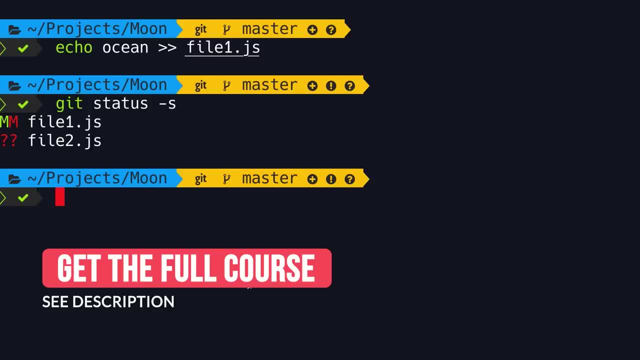 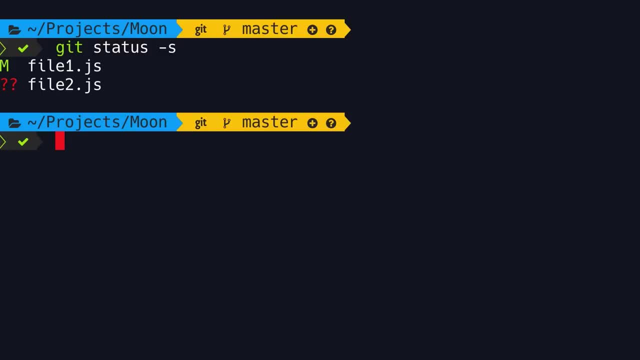 added to the staging area. So let's add file1 to the staging area one more time And then run git status dash s. Now all the changes that we had in the working directory are now in the staging area. So we're done with file1,. 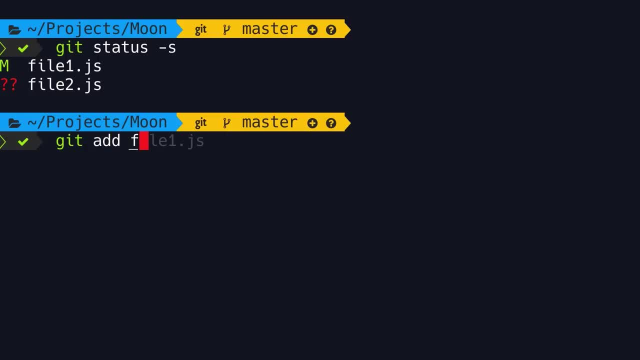 let's look at file2.. So I'm going to add file2 to the staging area as well And then run git status dash s For file2. we have a green a in the left column, which represents added. So file2 is added. 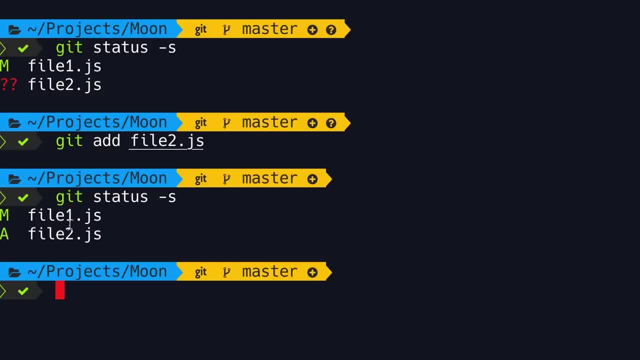 and file1 is modified. This is how the short status output works. So we have staged a couple of changes. now, before committing what we have in the staging area, we need to review our code, because we don't want to commit bad code or broken code. 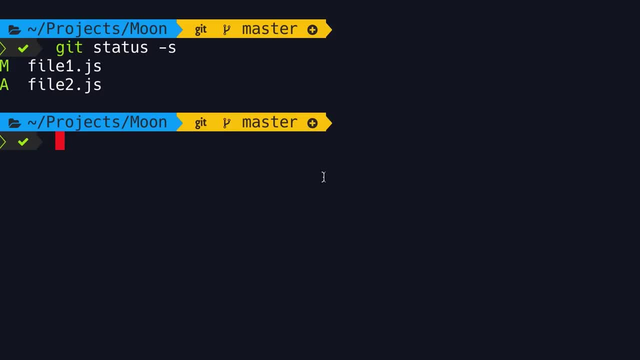 to our repository. So, as a best practice, always review what you have in the staging area before making a commit. Now the status command only shows the files that have been affected, but how can we see the exact lines of code that we have staged? We use the diff command. 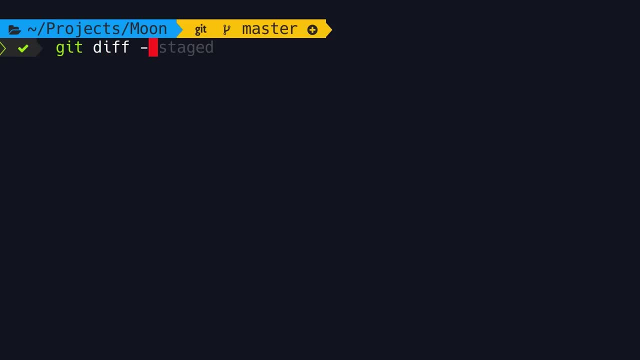 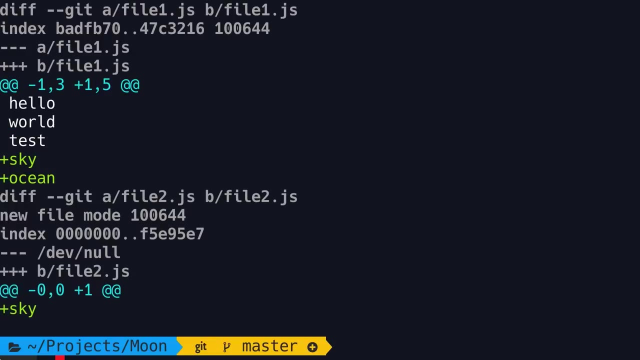 So we type git diff, dash, dash, staged- to see what we have in the staging area that is going in the next commit. So let's take a look here Now. quite frankly, comparing files using the terminal window is not really the best way to do this. 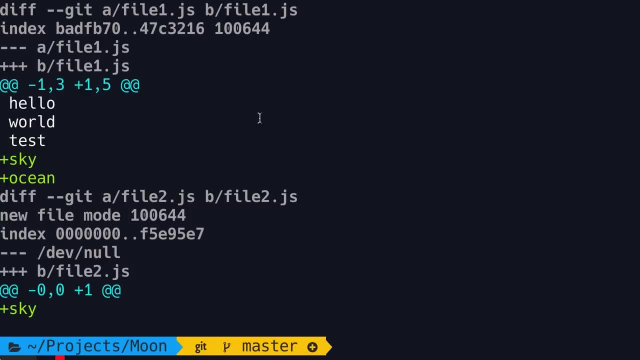 quite often we use visual tools- and I'm going to talk about that in the next video, But I think it's essential for you to understand the output of this command, because there are times that you may not have access to a visual tool. 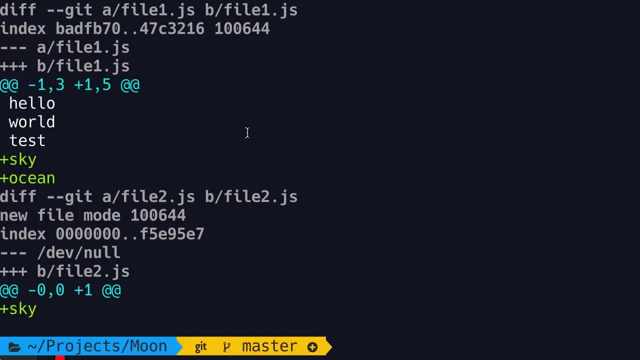 or at least you may go to an interview and you may get asked: what is the output of this command? So you need to be able to explain it. So on the top you can see that the diff utility was called with these arguments. 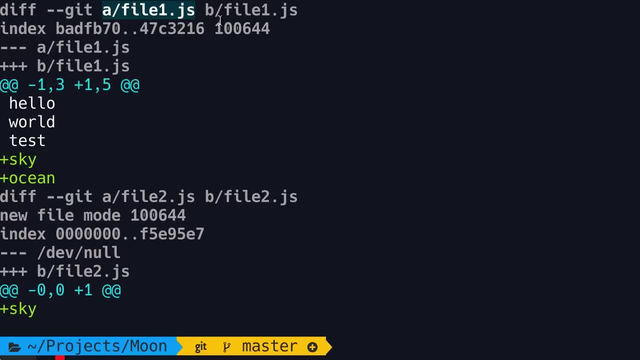 So we are comparing a slash file1.js with b slash file1.js. So we are comparing two copies of the same file. The first copy is the old copy, which is what we have in the last commit, and the second copy, which is the newer copy. 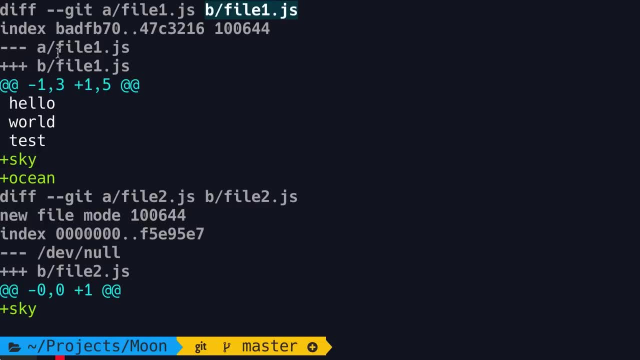 is what we currently have in the staging area Now. below that we have index, whatever. this is just some metadata, it doesn't really matter. After that we have a legend. So changes in the old copy are indicated by a minus sign and changes in the new copy. 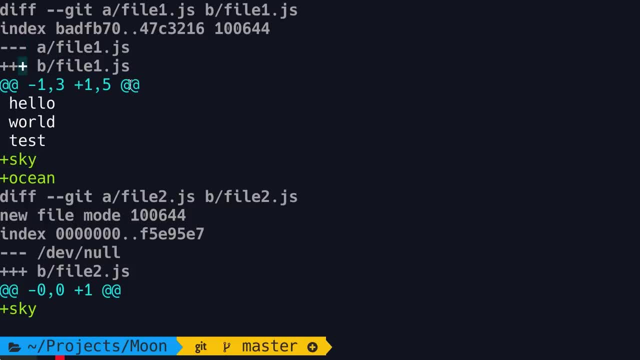 are indicated by a plus sign. After that we have this section. this is a header with some information about what parts of our file is changed. So currently our files are very short. they have only a few lines of text. but in the real world your file might have. 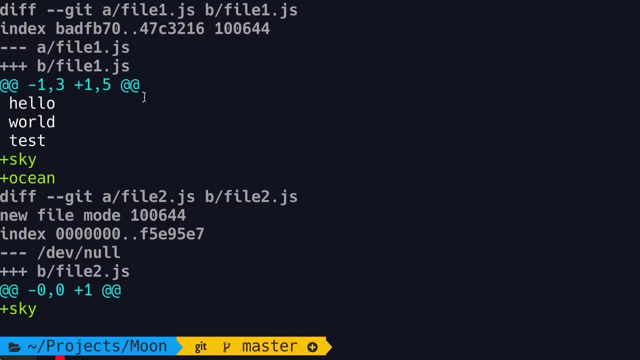 hundreds of lines of code. If you change only a couple of lines, it is not going to show the entire file. It's going to divide that file into chunks and what we have here is just a single chunk. So every chunk has a header. 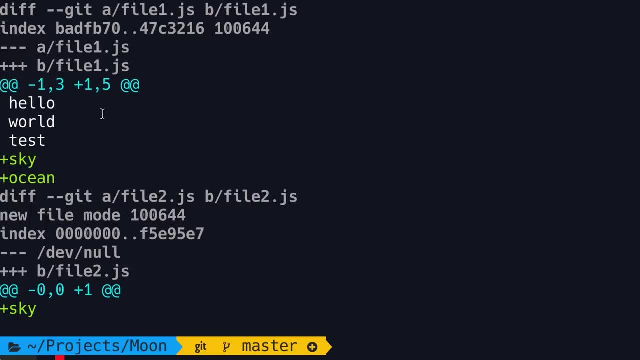 with some information that gives you context. So let's see what we have here. We have two segments. the first segment is prefixed with a minus sign, so this gives us information about the old copy, what we have in the last snapshot. The second segment: 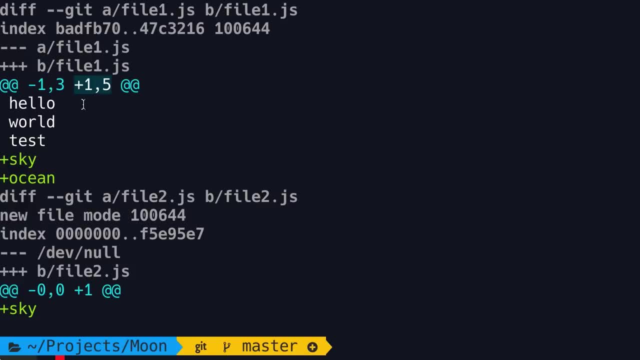 is prefixed with a plus sign. so this contains information about the new copy, which is what we have in the staging area. So in the old copy, starting from line one, three lines have been extracted and shown here In the new copy. 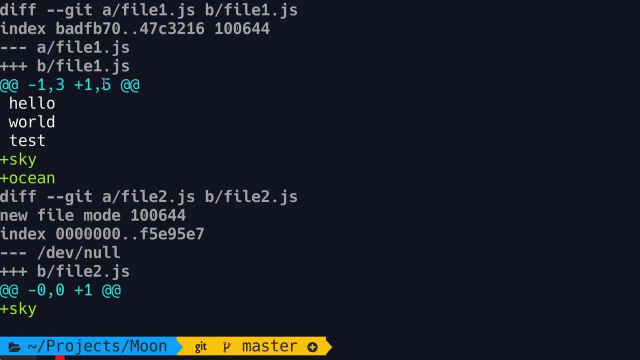 once again, starting from the first line. five lines have been extracted and shown here, So these are all these lines over here. Now you can see that these two lines are prefixed with a plus sign. so these are the lines that we have added in the new copy. 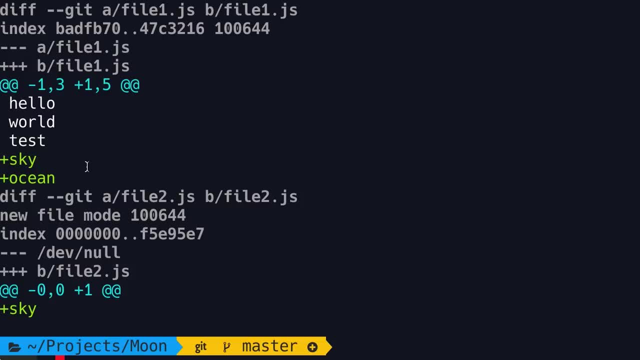 So we have added these lines in the staging area. They're green, which means they're new lines. So pretty straight forward. Now, after that, we have in the last call to the diff utility. this time we're comparing two copies of file, two Now in this case. 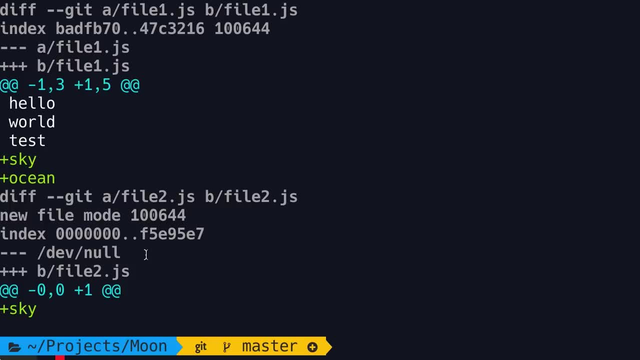 look at the legend. We don't have an old copy because this is an entirely new file. So in the last commit we didn't have a file called file two. That is why in this header we have zero comma zero, which means starting from line zero. 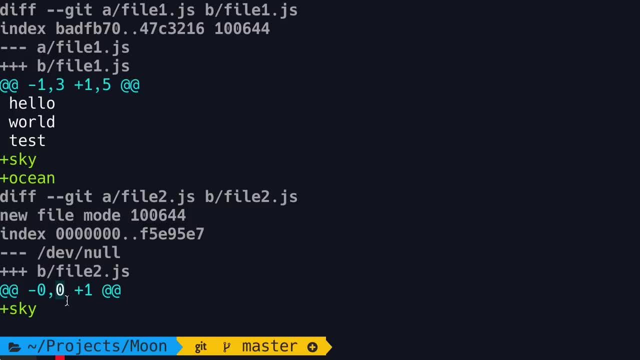 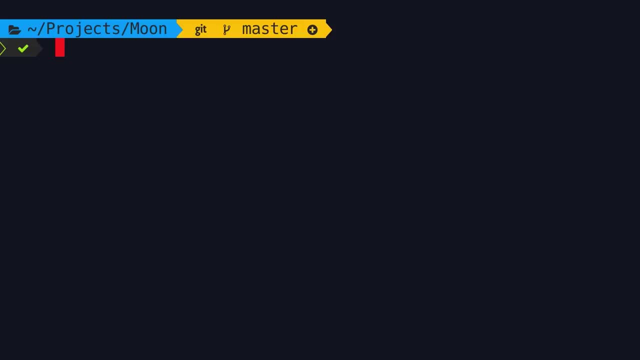 zero lines have been extracted Because there is no old copy of this file. Now what if you want to see the changes in our working directory that are not staged yet? To do this, we run get diff without any arguments. So this compares. 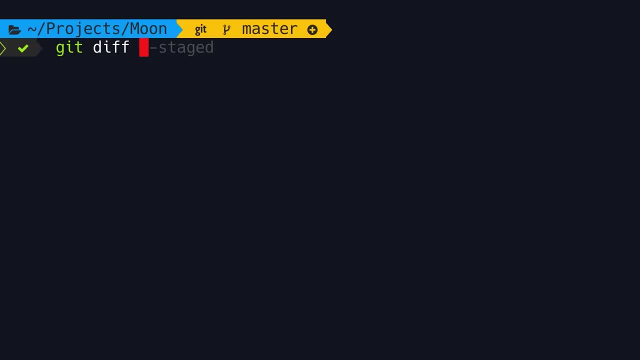 what we have in the working directory with what we have in the staging area. Take a look. There is no output here because we have staged all the changes in our working directory. We can also verify this using our short status command. So all the changes in our working directory are. 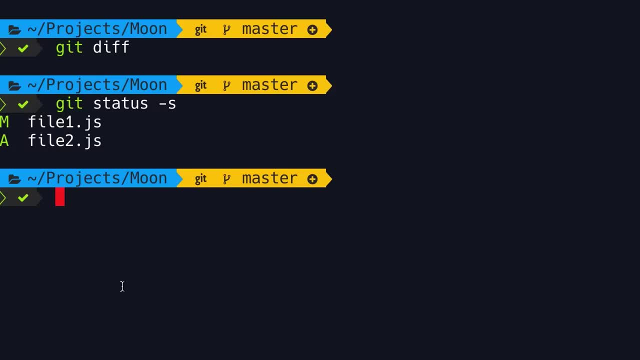 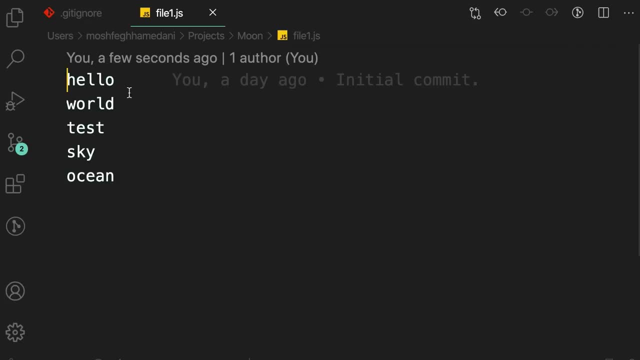 now in the staging area. So for this demo I'm going to make a change to file one. So let's open it with vs code or our favorite editor. So I'm going to change the first line to hello world, Save now. 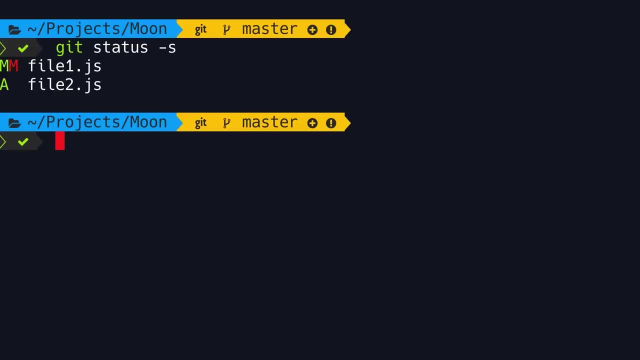 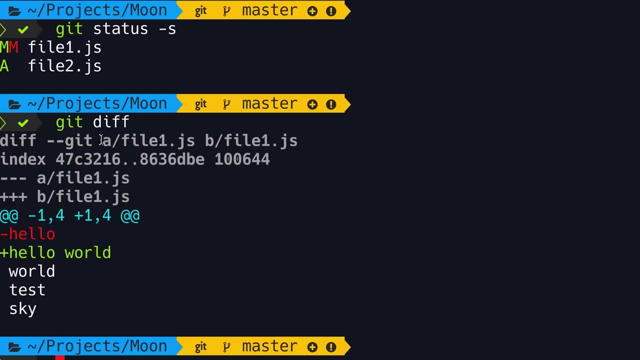 Let's run another short status. So for file one, we have some changes in our working directory that are not in the staging area. Let's look at these changes using the diff command. So get diff without any arguments. take a look. So here we are comparing two copies of file one. 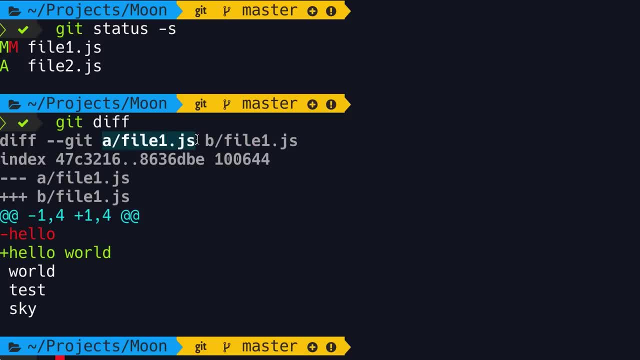 The old copy is what we currently have in the staging area And the new copy is what we have in the working directory. Now take a look In the old copy, which is indicated by a minus sign, we have this line: hello. 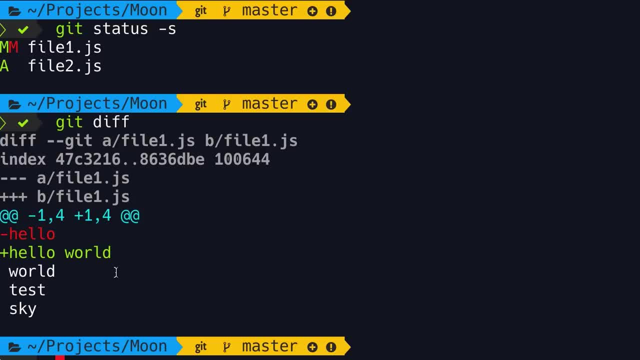 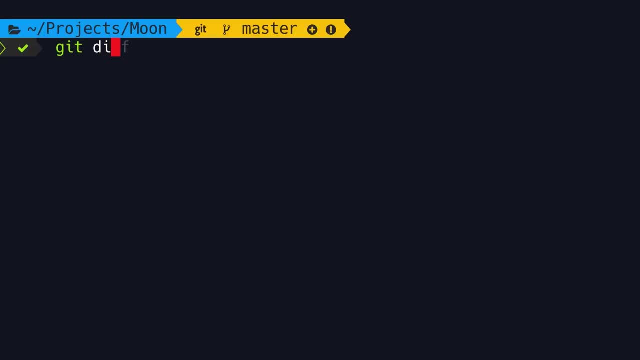 which is removed because it's red, And in the new copy, which is what we have in the working directory, we have this new line: hello world. So, to recap, if we run get diff without any arguments, we can see unstaged changes. 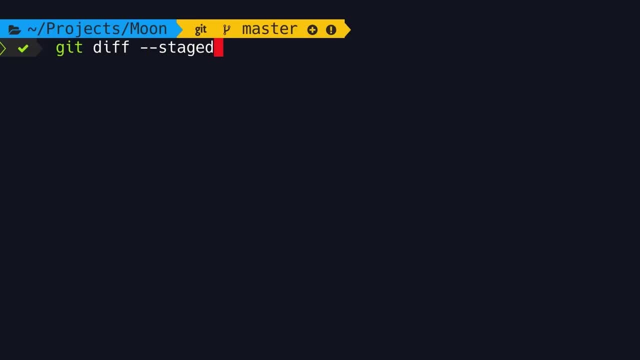 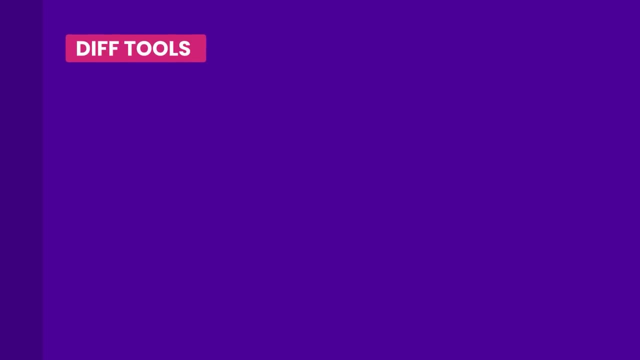 and if we pass dash dash staged, we can see the state changes that are going to go in the next commit. In this case, I'm going to show you how to use a visual tool to easily compare files. As I told you in the last lesson, quite often we use 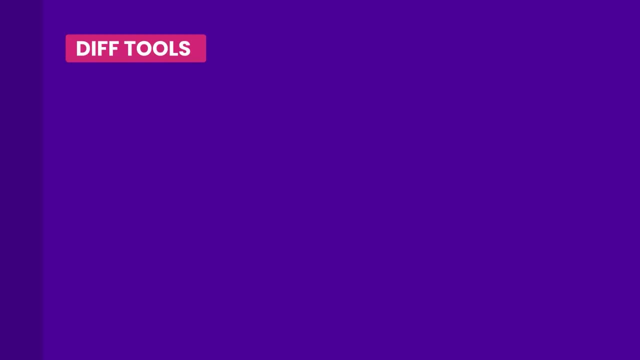 visual diff tools for comparing files. There's so many visual diff tools out there. the most popular ones are kdiff and p4merge, which are cross platform, and winmerge, that runs only on windows. In this lesson, I'm going to show you how to use. 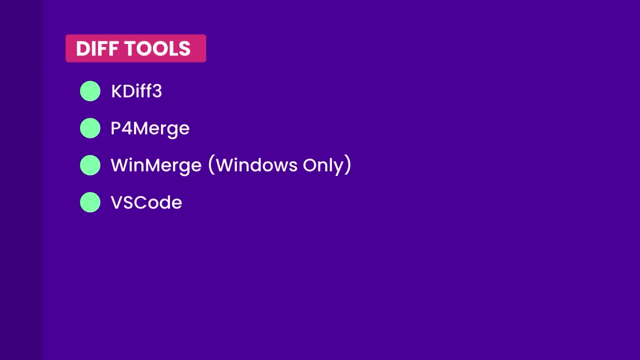 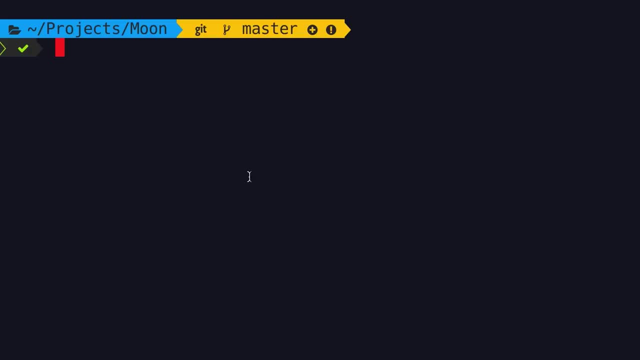 vs code for comparing files. If you want to use a different tool or a different editor, you have to look up this link in the description. So here in the terminal first we have to tell get that we want to use vs code as our default diff tool. 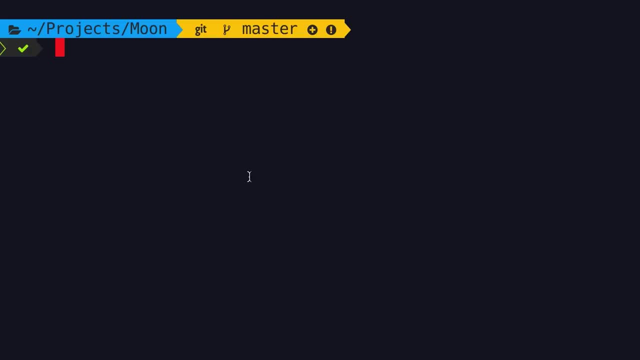 So we have to set two configuration settings. so once again we type: get config, dash, dash, global. so the global settings apply to all of our repositories. Now the setting we're going to set is diff dot tool. we're going to set that to vs code. 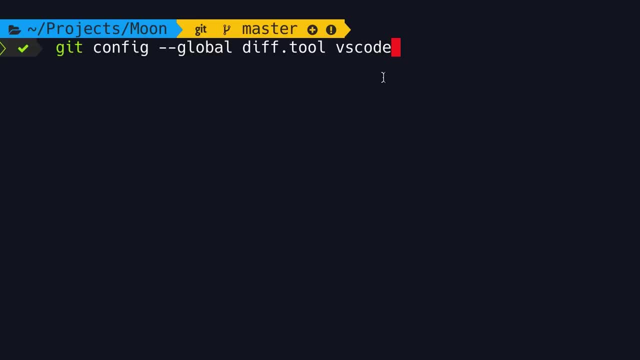 So with this command we're just giving a name- in this case vs code- to our default diff tool. Next we need to tell get how to launch a visual diff tool. So once again, get config, dash, dash, global. here we set diff tool. 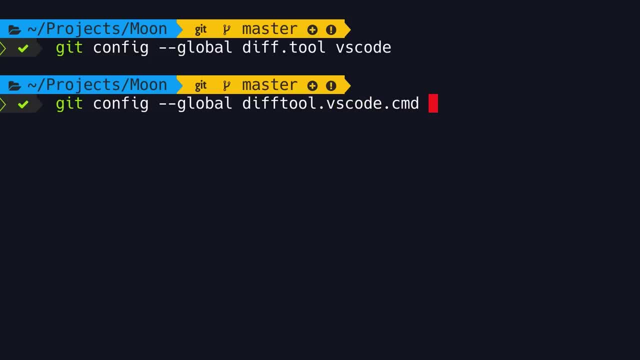 dot vs code. dot- cmd. We set this to double quotes because we're going to have a space Now on my machine I've added code to my path so I can run it from any directories. if this doesn't work on your machine, 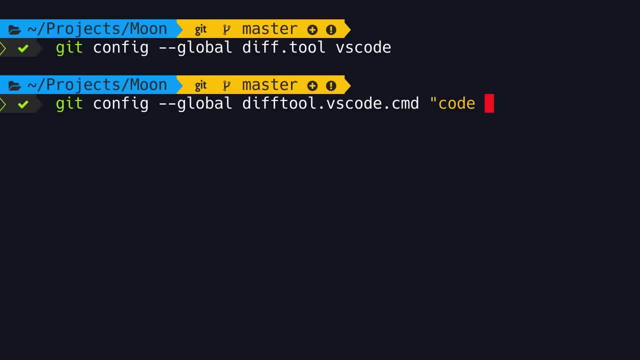 you have to look up the instructions yourself, depending on your operating system. So we're going to launch code with a few arguments. The first one is dash, dash, wait. this tells the terminal window to wait until we're done with vs code, So until we have compared the changes. 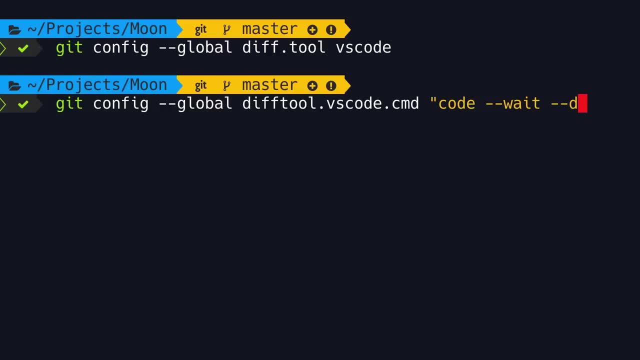 and closed the vs code instance. The second argument is dash dash diff. this tells vs code that we want to use it for diffing or comparing files. then we have two more arguments: dollar sign local in capital and dollar sign remote in capital. 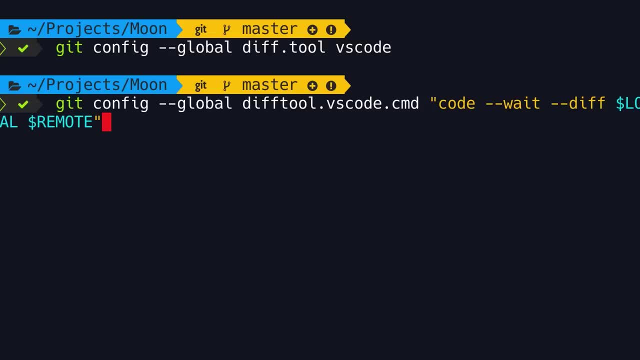 These are placeholders for the old and new copies of a file. Okay, So let's set that now. let's make sure that you've got this step right. So we're going to run get config, dash dash, global dash e, As I told you at the beginning of the course. 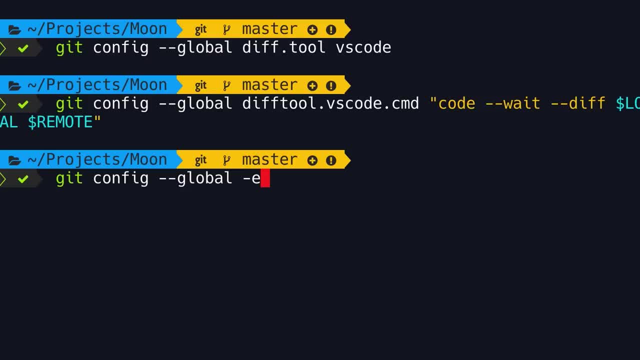 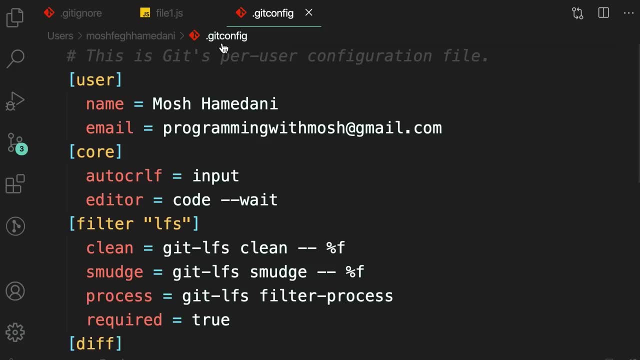 with this command we can edit our global configuration settings in our default editor, which is vs code. So take a look. So all the settings are stored in this file. dot get config, which is stored in this directory. So we have the user section. 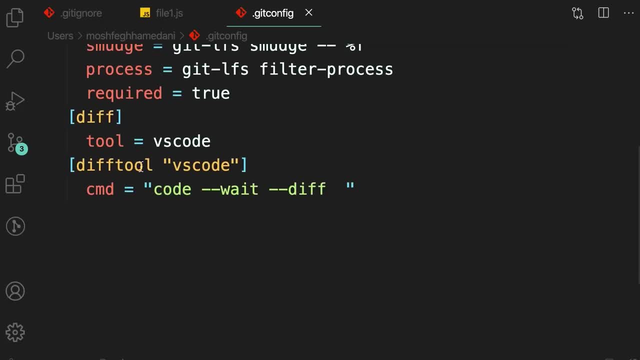 which we set earlier in the course. now here's the diff section that we just set. In this section we have set the tool to vs code. this is just a name. then we have diff tool vs code and here's the command. 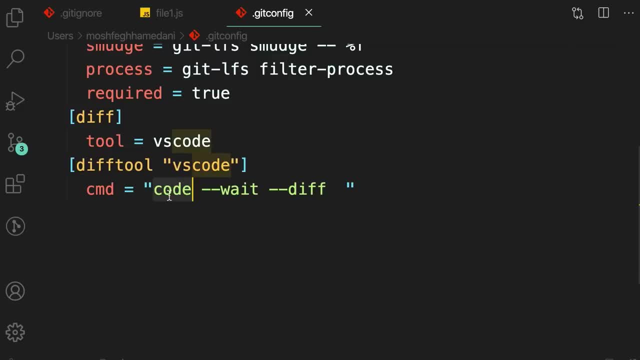 that should be run for comparing files with vs code. So we have code with dash dash wait, then dash dash diff. now those two placeholders that I added. for some reason they're lost, So let's add them real quick. dollar sign local. 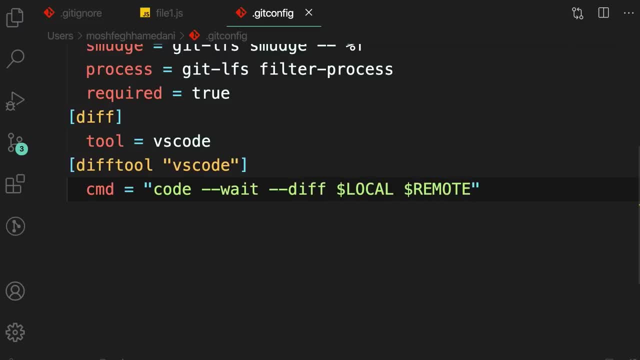 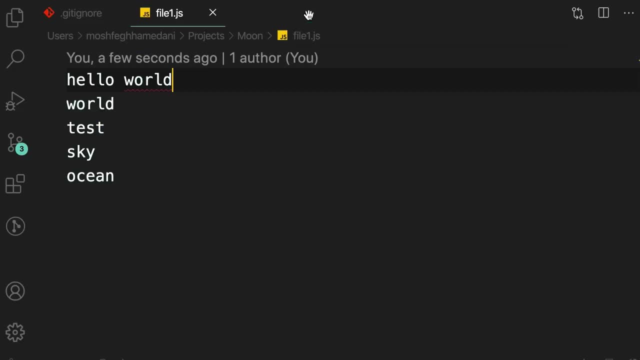 and dollar sign remote. Make sure to get this right, otherwise things are not going to work on your machine. Now we're done. so, as close as we know, we're going to run the back in the terminal. instead of using the diff command, we're going to use 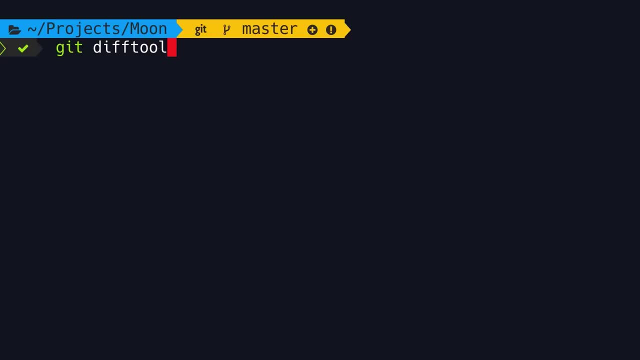 diff tool. this will launch our visual diff tool for comparing files. Now, if you don't supply any arguments, we're going to see our unstate changes. So this will compare what we have in the working directory with what we have in the staging area. 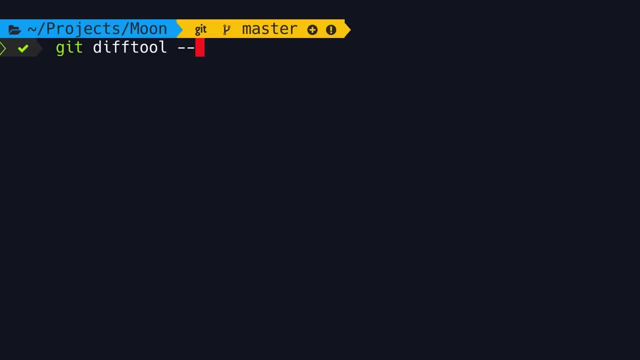 If you want to look at our state changes, we supply dash dash stage exactly the same way we use the diff command. So let's look at the changes we have in our working directory. We have modified only the single file. that is why we have 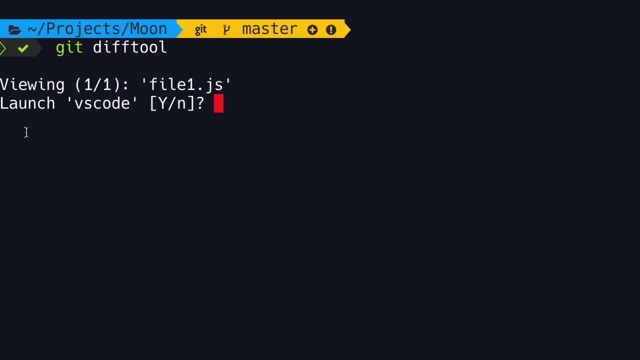 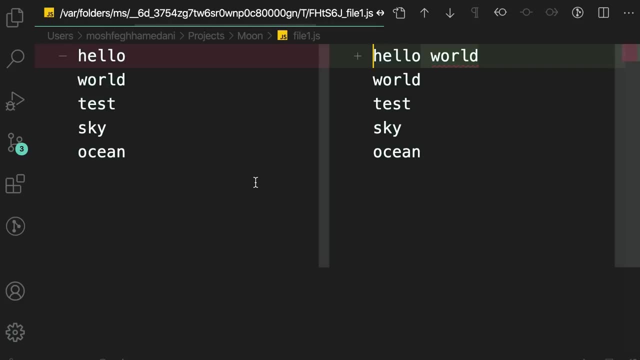 one out of one, and that is file1.js. So git is asking: if you want to launch vs code, which is the name that we assigned to our default diff tool, let's go ahead, take a look. So here's the old copy, which is what we. 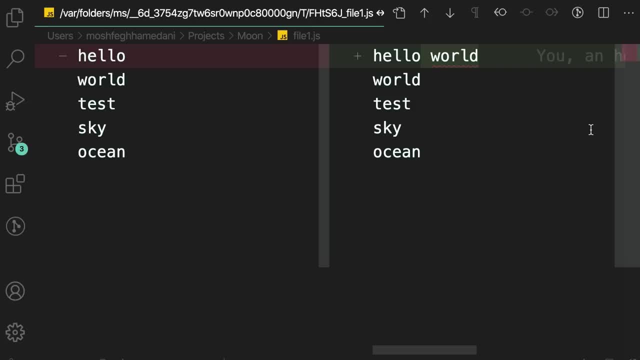 have in the staging area. and here's the new copy, which is what we have in the working directory. As you can see, we can easily tell that this line has been replaced with this line. It's much easier to see the changes. 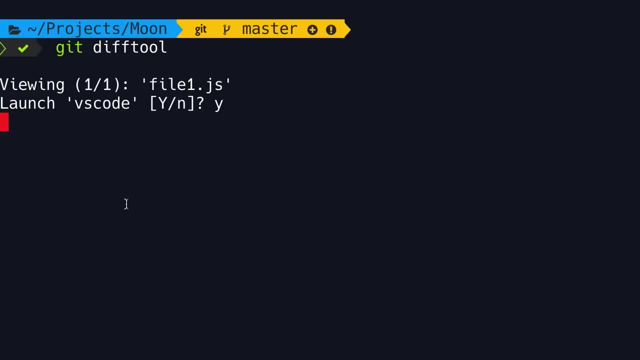 Now the terminal window is with the waiting for us to close the vs code instance. So let's close this window back to the terminal. now let's look at the state changes. So git diff tool: dash, dash staged. Two files have been affected in the staging area. 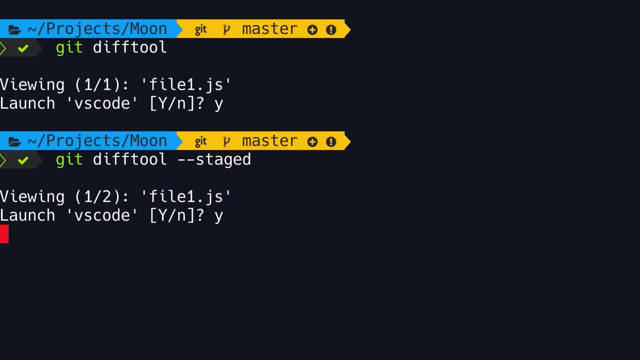 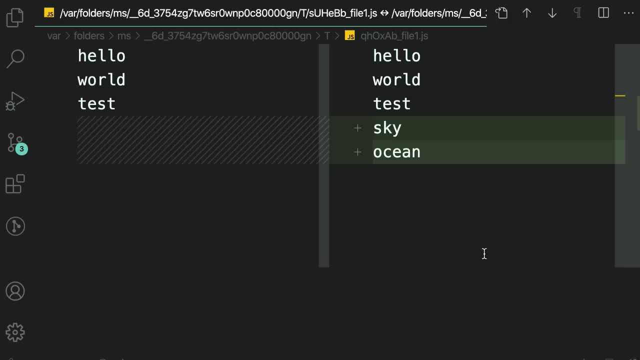 the first one is file1.js. Let's look at the changes. Alright, in this case, the old copy is what we have in the last commit and the new copy is what we have in the staging area. So these are the changes that are going to go in the next commit. 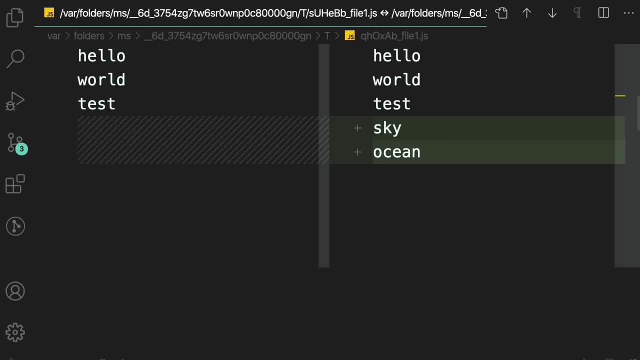 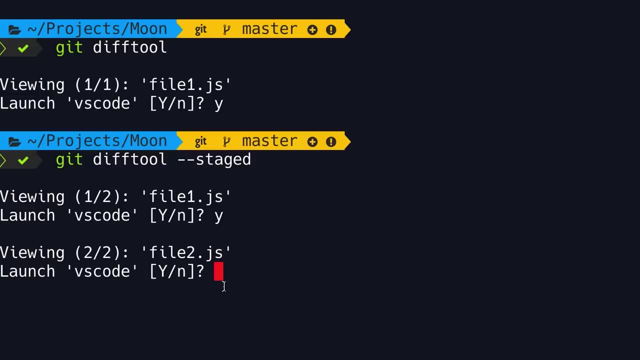 We can easily tell that the we have added two lines here. Now let's close this tab. back in the terminal, git is asking if you want to look at the changes in file2.js. In this case, I'm going to ignore that. 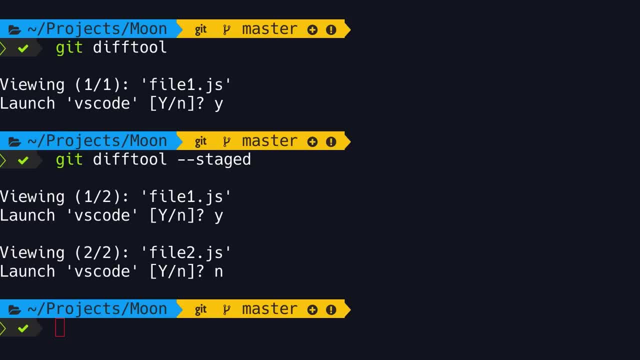 so no, Quite, honestly, we don't use diff tools so much these days. I just covered it because I want my course to be comprehensive. These days, most editors and ids allow us to view the staged and unstaged changes as part of our development. 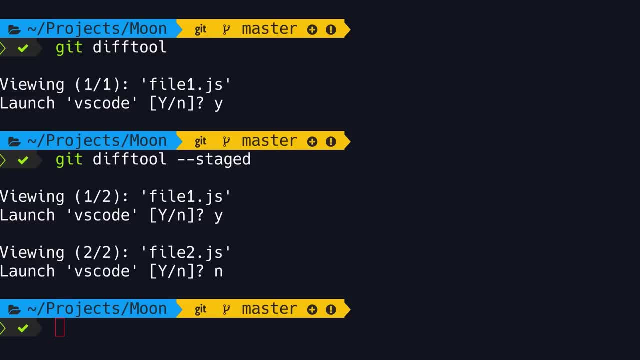 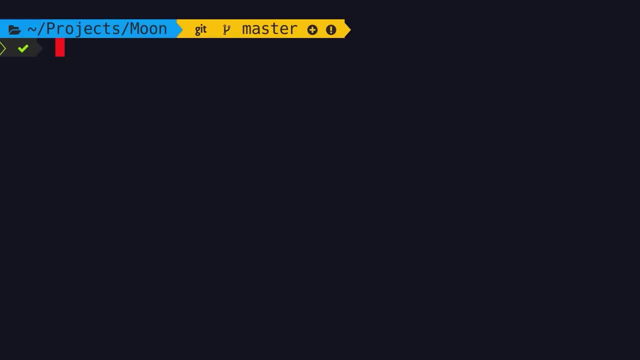 environment. I will show you how to do this later in this section. So we have made a few commits so far, but where are these commits? Let me show you. So we use the log command to look at our history. Take a look. 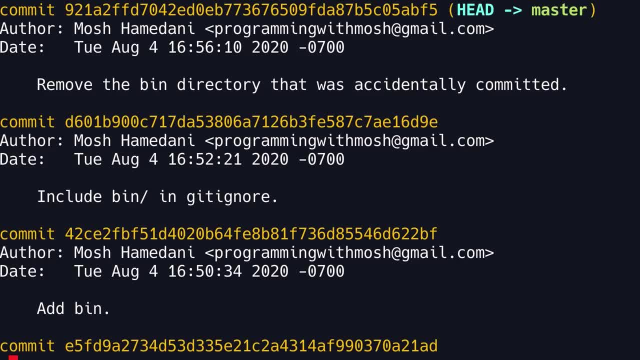 So here are all the commits we have created, sorted from the latest to the earliest. So here is our last commit on top. each commit has a unique identifier. this is a 40 character hexadecimal string that git automatically generates for us. You can think of it like a revision number. 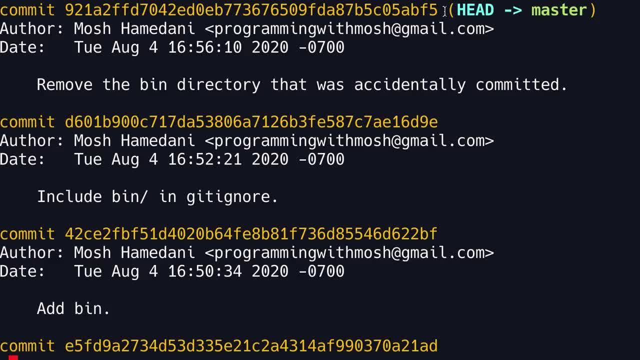 but, unlike a revision number, it doesn't increase. It's just a unique identifier. Okay, Now, next to that, we have head pointing to master. What is this? Well, we're going to talk about this a lot in the future, but 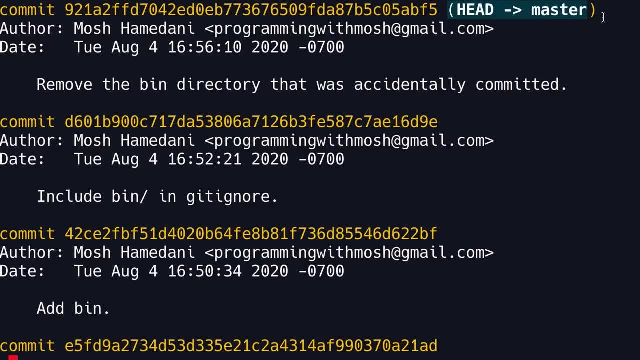 master is the main branch or the main line of work in git. In some other version control systems it's called trunk. In git we can have multiple branches, so we can work on multiple features or multiple bug fixes in parallel and then combine our code. We'll talk. 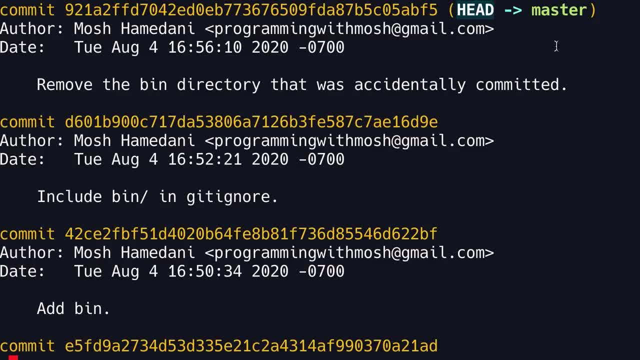 about that later in the course. Now, head is a reference to the current branch, So this is how git knows what branch we're currently working on. Again, we're going to talk about this a lot in the future. Now, for each commit, you can see the author. 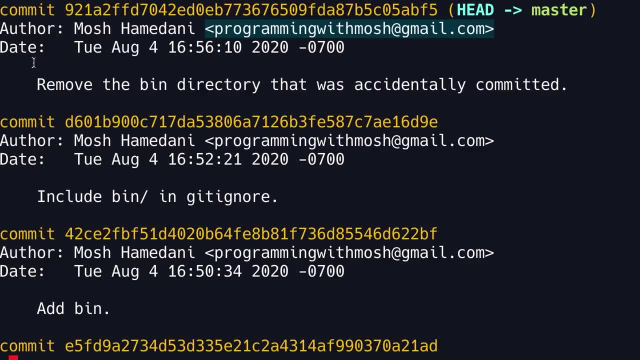 the name of the author, as well as their email, the date and time the commit was created, as well as the one line description. Now, here we have multiple commits that are spread across multiple pages. We can press space to go to the next. 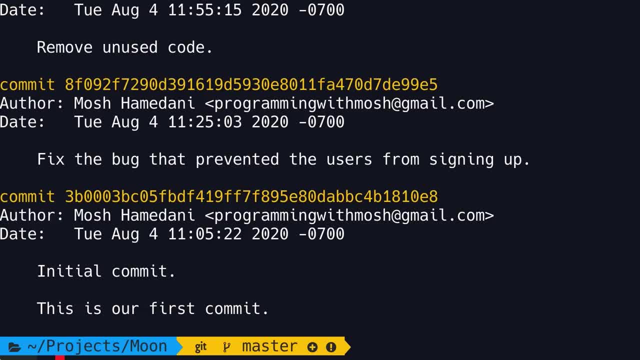 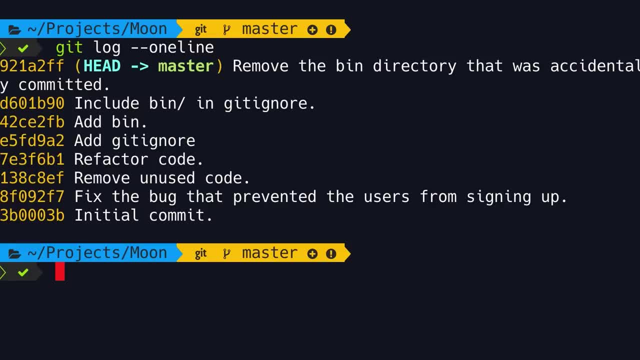 page. and again now to quit, we can press q. Now. the log command has a few interesting options. One of them is one line. This shows us a short summary of the commits. So here we have the unique identifier that is shortened to 7 characters. 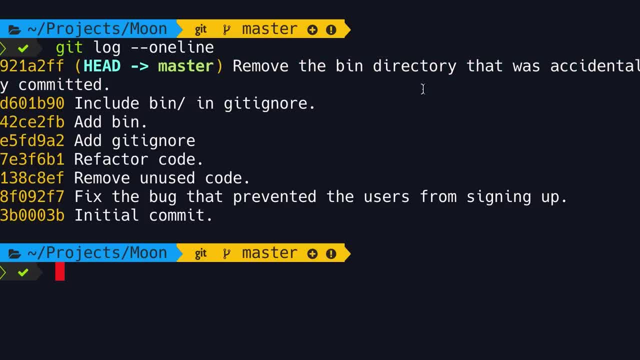 and we only have the one line description, So we don't have the author as well as the date and time of each commit. We have another option for reversing the sort order. Let me show you. So git log one line and then we add: 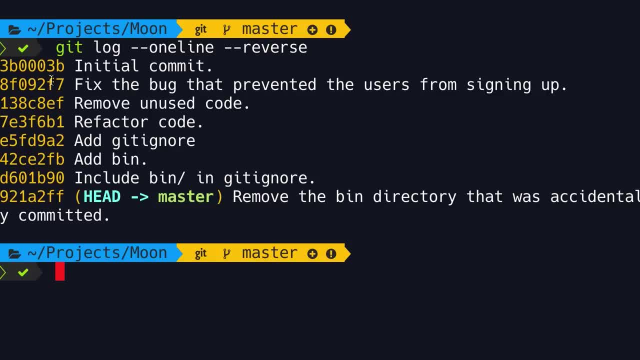 dash, dash, reverse. Now you can see the first commit being on top and here's the last commit. Now the log command is very powerful, so in the future we're going to use this command. we're going to talk a lot about it, in fact. 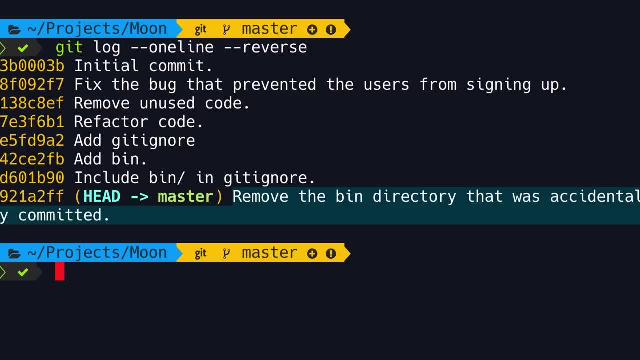 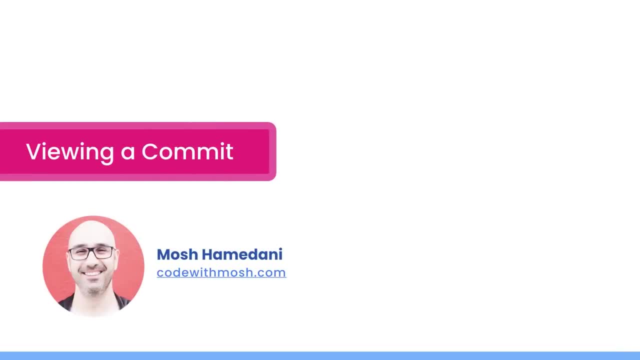 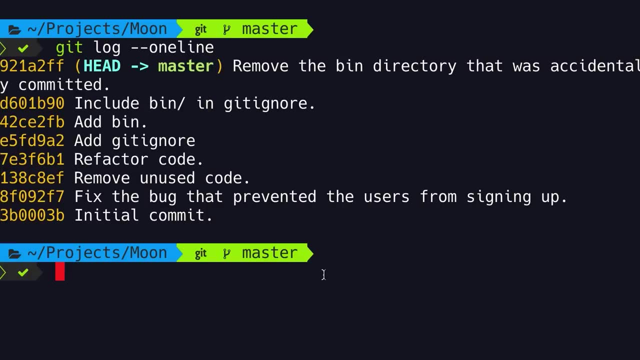 we have a complete section on browsing history. I'm going to show you various ways to get reports from the history. For now, let's just stick to the basics. So viewing the list of commits is great, but what if you want to see what exactly we have changed in a given? 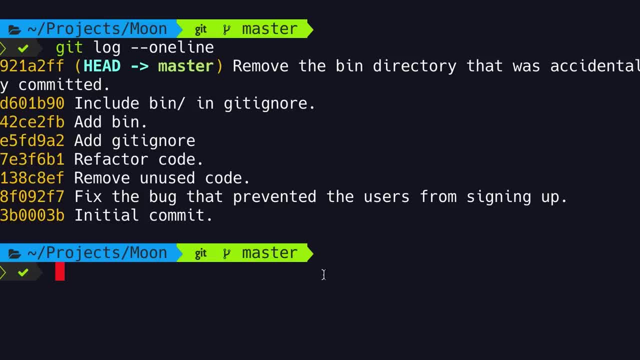 commit. That's when we use the show command, For example. let's say we want to look at the content of this commit. over here We type git show. now here we need to specify the content of the commit we want to inspect. There are two ways to. 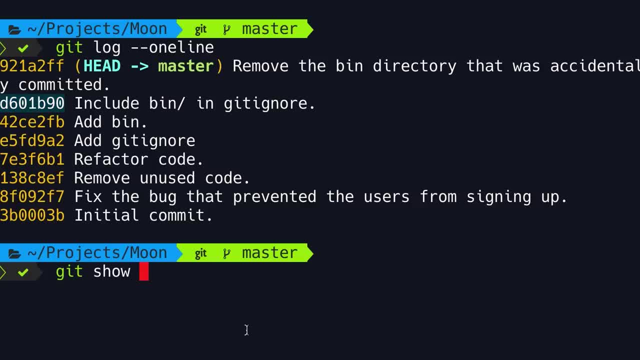 reference a commit, We can reference it using its unique identifier, so we type d601b90.. Now we don't have to type all the seven characters. we can type fewer characters, as long as we don't have another commit whose id starts with these characters. 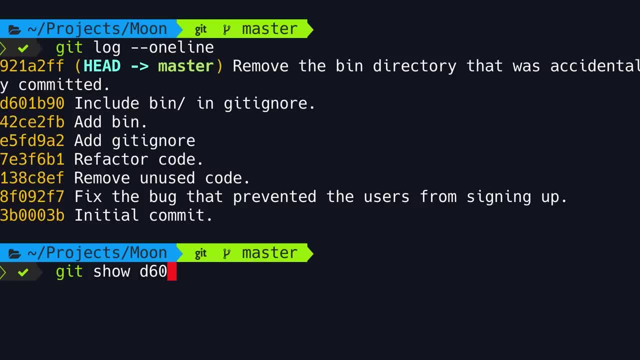 So that's one way to reference a commit. Another way is to use the head pointer. So look, head is currently in front of the last commit. So to view the last commit we can type head, or to look at previous commits. 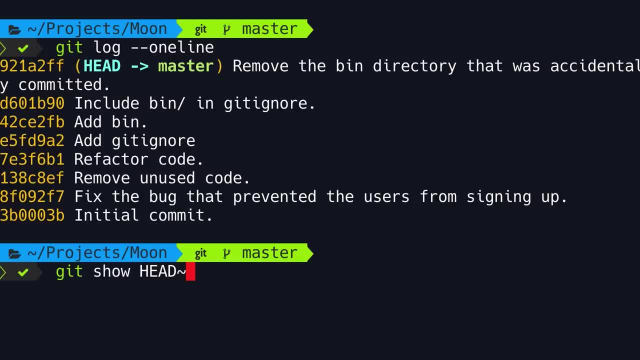 we can type the last commit And then specify how many steps we want to go back. So if we type one, we start from head, which is here, we go one step back, and this references this commit over here. Let's take a look. 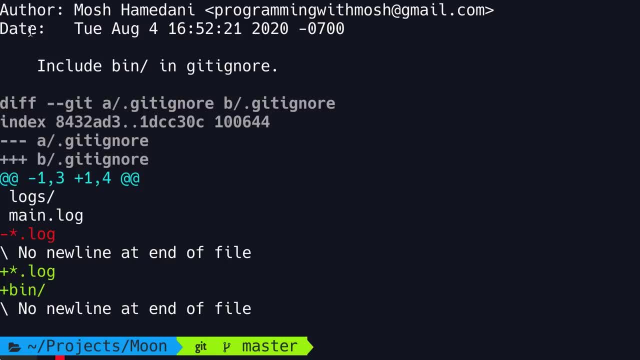 So on the top we can see the author and the date of this commit, as well as its message Below that we have a diff of what is changed. So in this commit we have changed a single file that is git ignore. Over here we can see that. 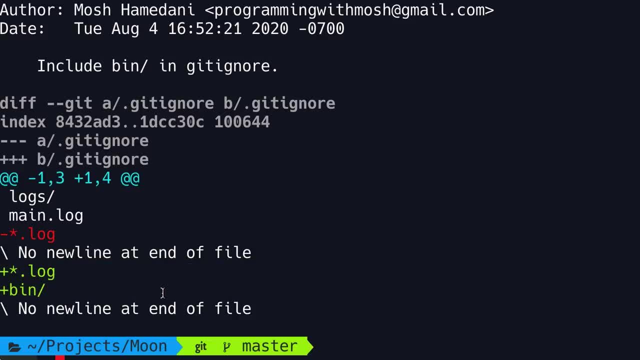 we removed this line and added these two lines, So this is very useful. Now, what if we don't want to see the differences? We want to see the final version, the exact version that is stored in this commit. Well, we bring up. 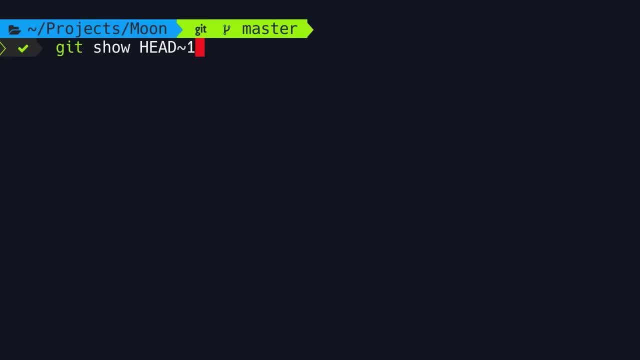 the last command, git show head tilde one. then we type a colon and here we specify the full pass to a file. For example we can say: dot, git ignore. or if this file is in a subdirectory, we type for example: bin slash amp. 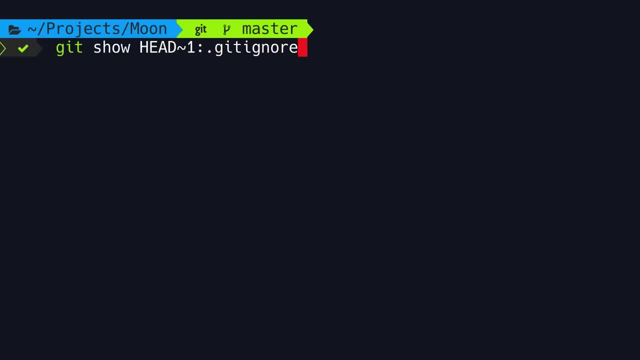 dot bin. Okay, Now let's look at git ignore. So this is the exact version stored in this commit. Now, earlier I told you that each commit contains a complete snapshot of a working directory, not just changes, But when we run the show command. 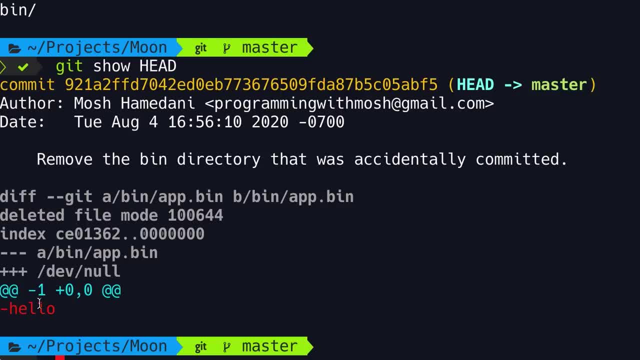 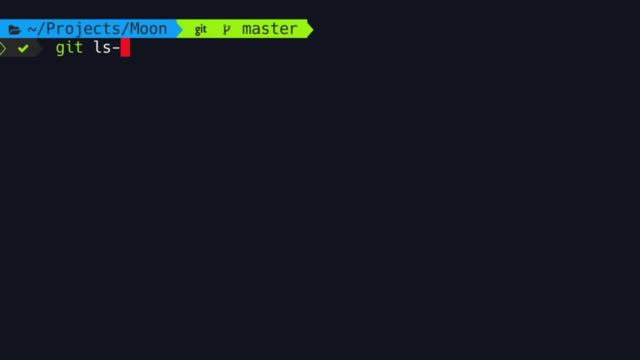 we only see the differences. what is changed? What if you want to see all the files and directories in a commit? Well, for that we're going to use a different command That's called ls tree. Now, why is this called a tree? Well, 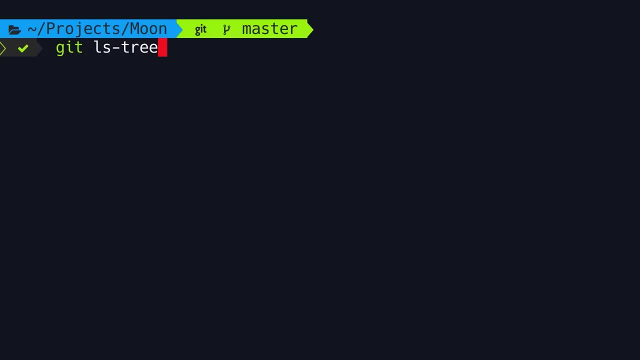 a tree is a data structure for representing hierarchical information. So in a tree we can have nodes and these are nodes can have children. Now a directory on the file system can be represented using a tree, Because each directory can have children. these children can be files. 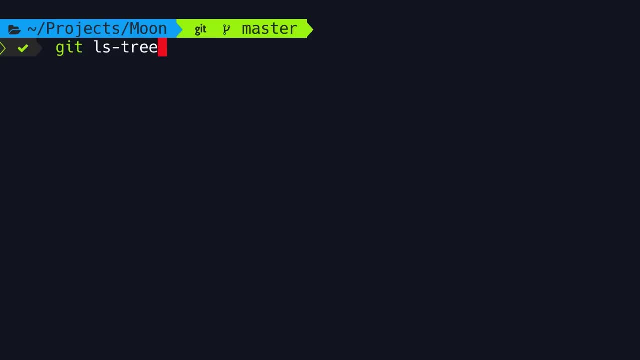 and other subdirectories. If you want to learn more about this concept, you should take my data structures course. So ls tree means list all the files in a tree. Now here we specify the commit we're interested in, head tilde 1,. 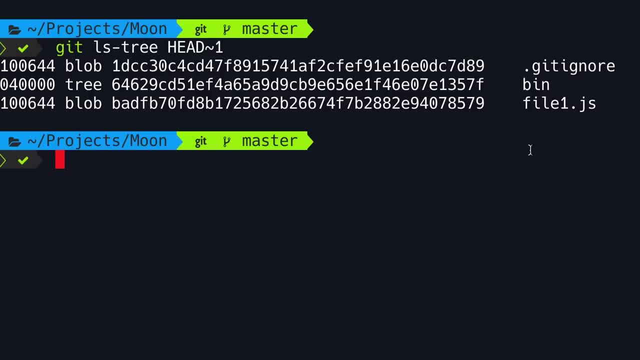 and now look, these are all the files and directories stored in this commit. So we have git ignore. right before that, we have a unique identifier that is generated based on the content of this file. So in git's database we have an object with this id. 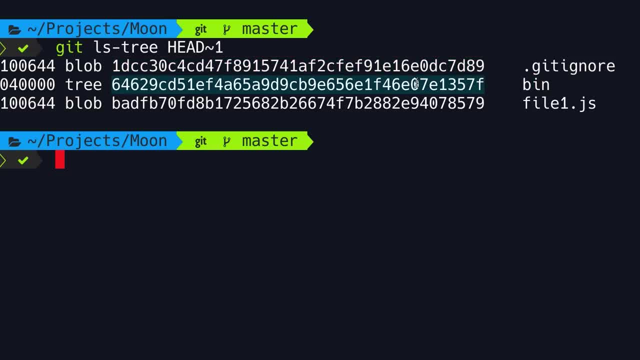 Below that we have bin again. it has a unique identifier that is generated based on the content of this directory. Now look at the type of this object. It's a tree, So files are represented using blobs and directories are represented using trees. 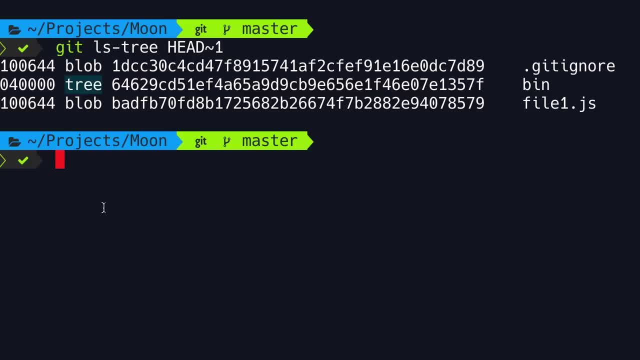 All of these are objects that are stored in git's database. Using the show command, we can easily view an object in git's database. For example, if we type git show, we can easily see the object in git's database And then specify this unique identifier. 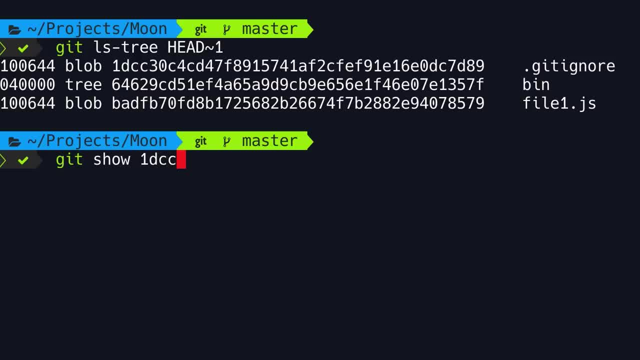 or we can type only the few characters, as long as there is no ambiguity. So here's the content of our git ignore file. As another example, let's look at this object, this tree, the bin directory. So git show. 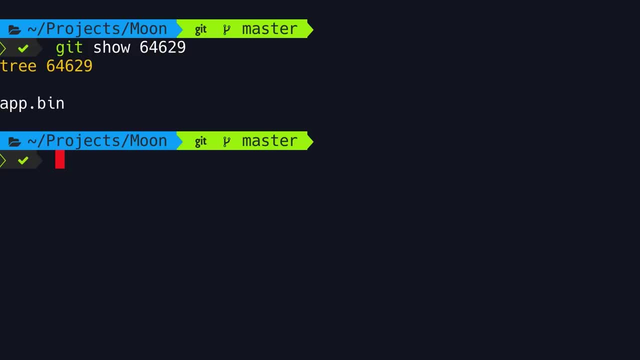 64629.. Here we have a tree. in this tree we have this file appbin. So using the show command we can view an object in git's database. These objects can be commits, blobs which represent files and trees. 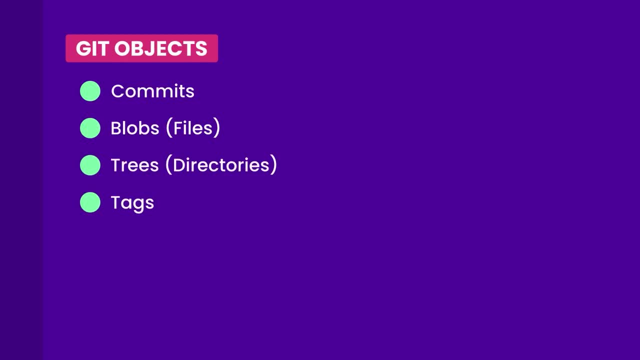 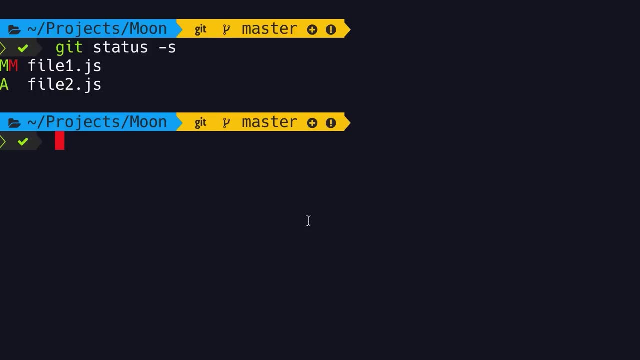 which represent directories as well as tags. We'll talk about tags in the future. So I told you that you should always review the stuff that you have in the staging area before making a commit. So let's say, we review these changes. 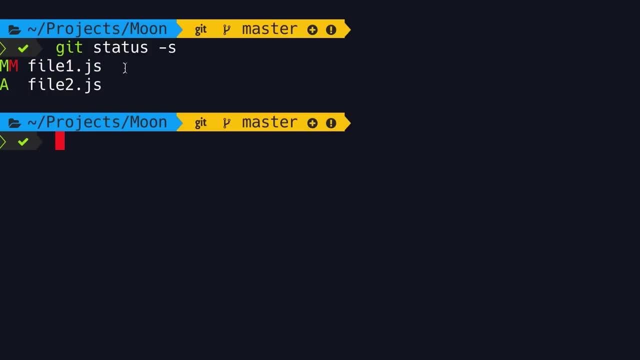 and we realize that the changes in file 1 shouldn't go in the next commit, Perhaps because these changes are logically part of a different task. So we don't want to have a commit that represents changes for different tasks, right? So in this case we want to undo the add. 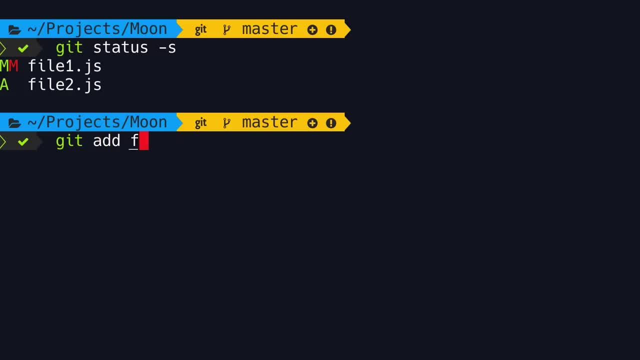 operation, Because earlier we used the add command to add file 1 to the staging area. Now we want to undo this operation. How do we do this? Well, in the past we used the reset command, but a lot of people found this command confusing. 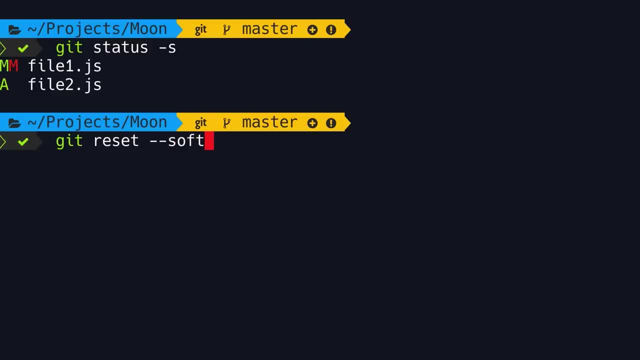 especially with options such as hard or soft. That's why we have a new command called restore. Now make sure you're using the latest version of git, otherwise what I'm going to show you is not going to work on your machine. So here I'm using git version. 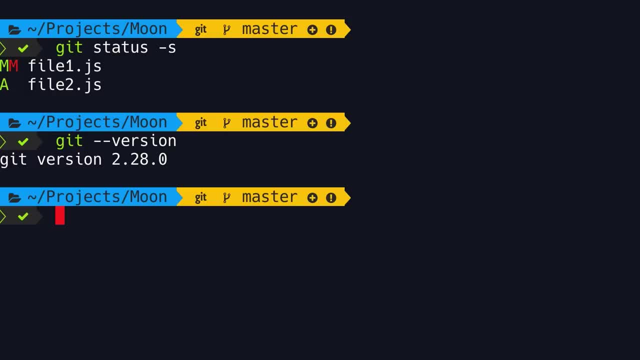 2.28, and with this we can easily restore files in different environments, in working directory or in staging area. So git restore. you want to restore file 1 in the staging area, So we type dash, dash staged, and then we specify: 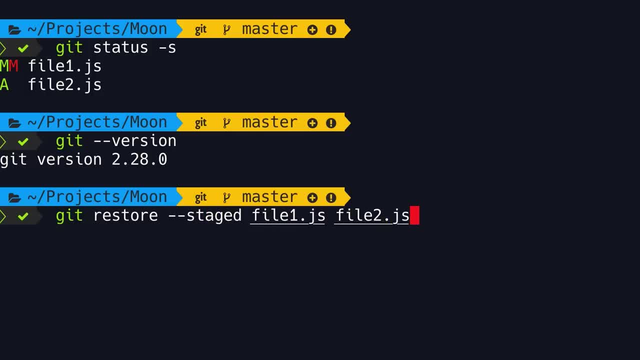 the file name. We can list multiple files here. we can also use patterns, or if you want to restore everything in the staging area, we simply use a period. So here I'm going to restore file 1.js. Now, when we run git status, 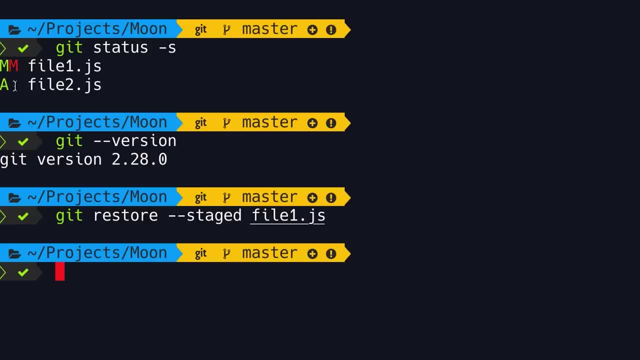 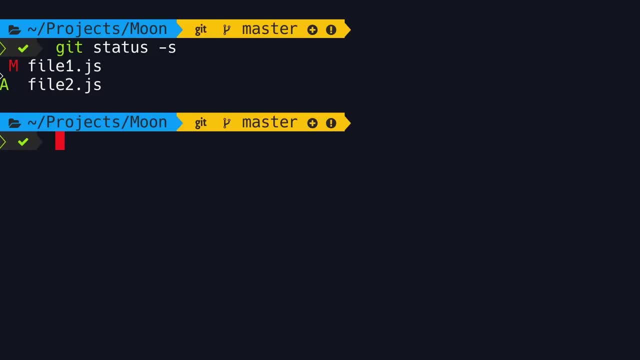 again. you're not going to see a green m here, because all the changes that we had in the staging area are now in the working directory. Take a look. So git status dash s look. we no longer have any changes for file 1 in the staging. 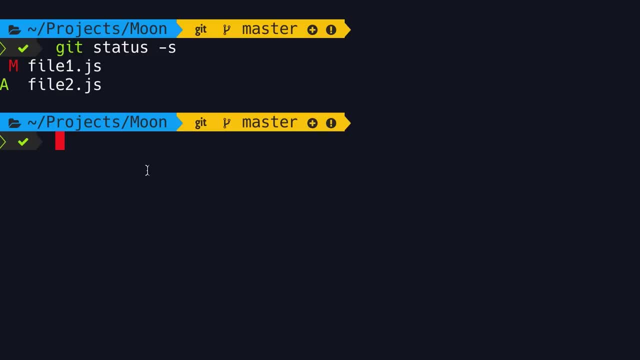 area. All the changes are in the working directory. Now it's essential for you to understand how the restore command works. The restore command essentially takes the copy from the next environment. So in case of the staging environment, what is the next environment, The last commit? 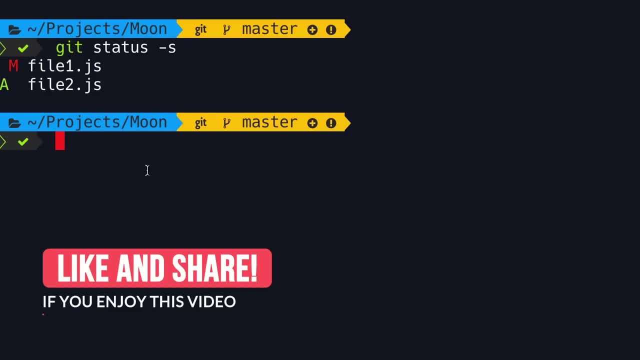 What we have in the repository. So when we restored file 1 in the staging area, git took the last copy of this file from the last snapshot and put it in the staging area. That is what happened. Now look at file 2.. 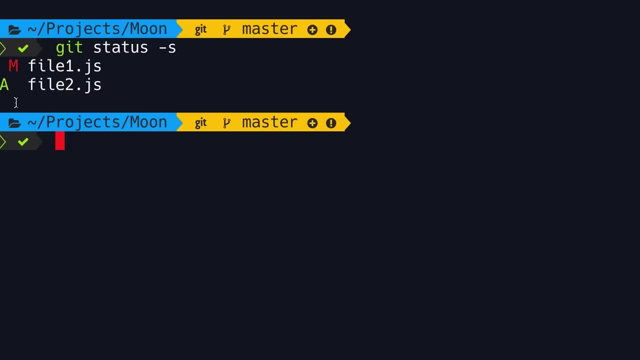 File 2 is a new file because here we have a green a which is short for added. So we have this file. we have this new file in the staging area, but this file doesn't exist in the last commit. So what do you think will happen when I? 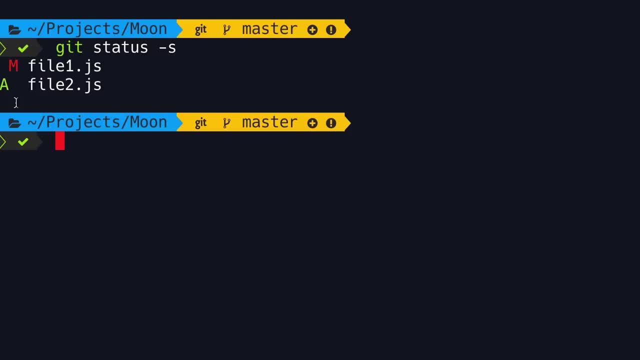 restore this file. Well, because we don't have a copy of this file in our repository or in our last commit, git is going to remove this file from the staging area and take it back to its previous state, which is a new on track file. Let me show you So. 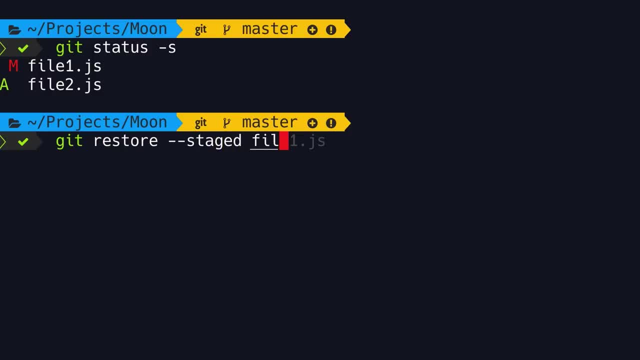 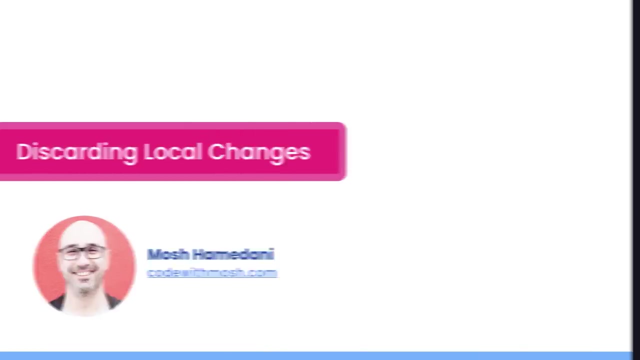 git restore dash, dash staged file2.js. Now let's run git status again. so file2 is a new on track file because we have two question marks. So there are times that we have some code in our working directory that we want to throw away. 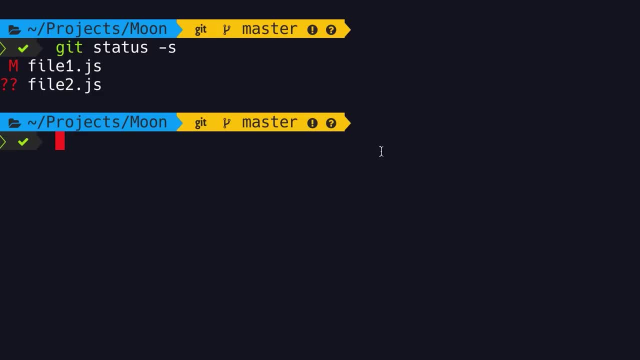 Let's say we made some changes but we didn't like those changes, so we want to scratch everything and start over. We can discard the local changes using the restore command. So here we have some local changes in file1.js. To undo these changes we type: git restore. 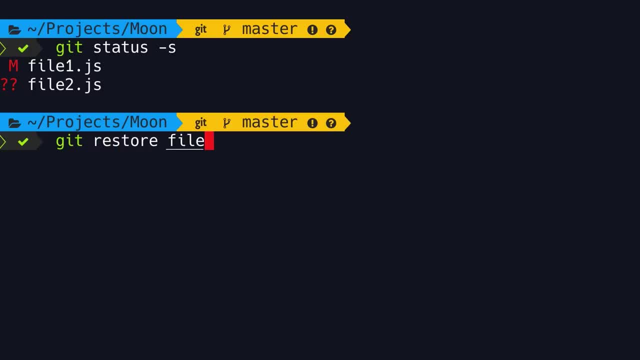 file1.js. When we execute this command, git is going to take the version of this file in the next environment. So let's run this command, Which is our staging environment. it's going to take that version and copy it into our working directory. We can also: 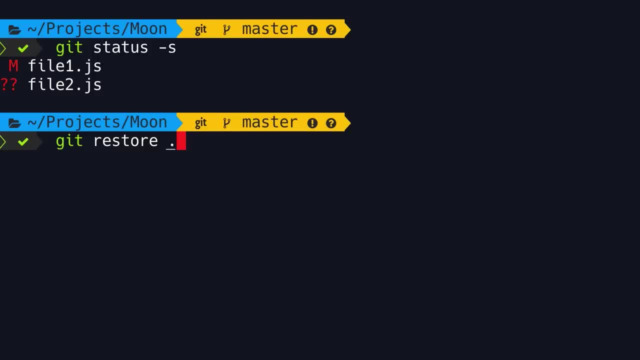 use a period here, and this will undo all the local changes. Now let me show you something. So the command is executed. now let's run another short status. but file2 is still here. Why is that? Well, this is a new. on. 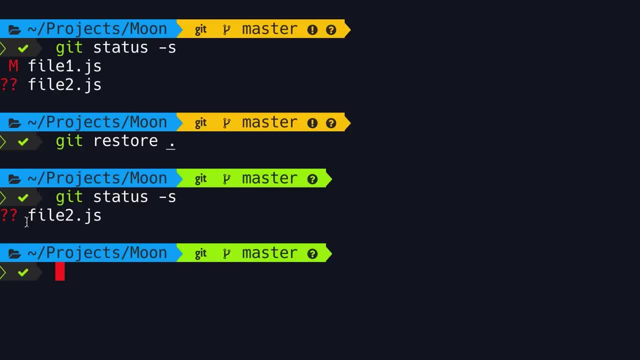 track file. so git hasn't been tracking this. So when we tell git to restore this file, git doesn't know where to get a previous version of this file. It doesn't exist in our staging environment Or in our repository. So 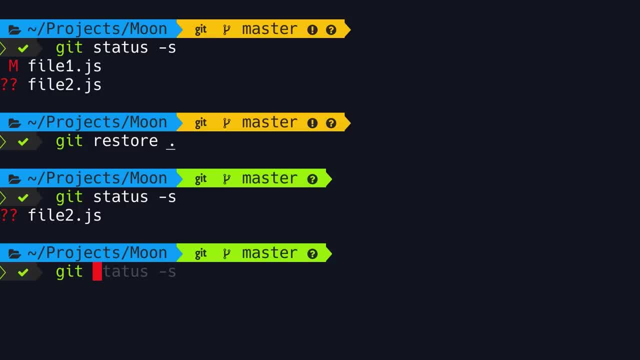 to remove all these new on track files we have to type git clean. Now take a look. By default we get this fatal error saying: require force defaults to true, and neither of these switches were given. So basically, git is telling us that hey. 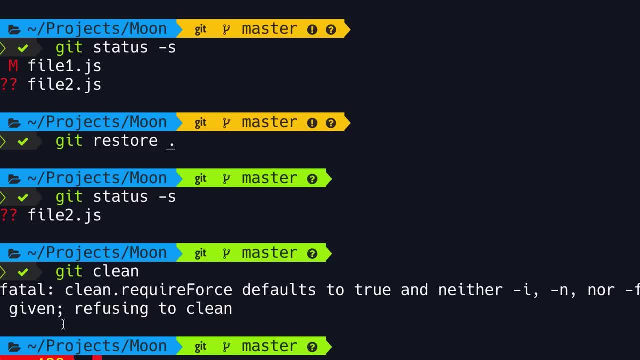 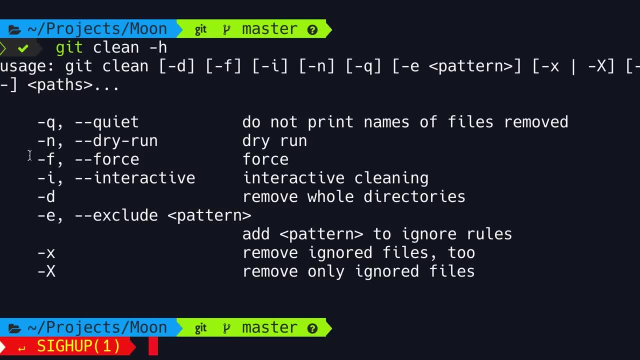 this is a dangerous operation. if you accidentally remove these on track files, there is no way you can recover them, So let's run git clean, dash h. for a quick help Here we have this option, dash f, which forces git to remove these on track files. 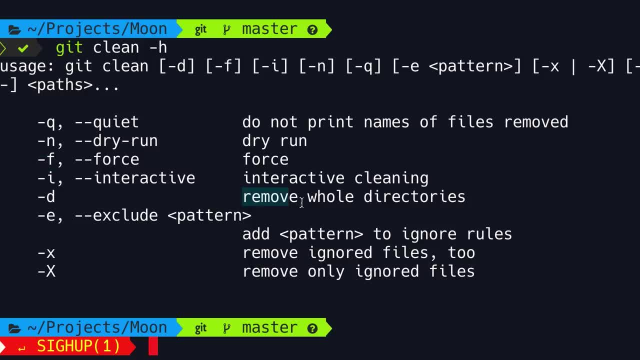 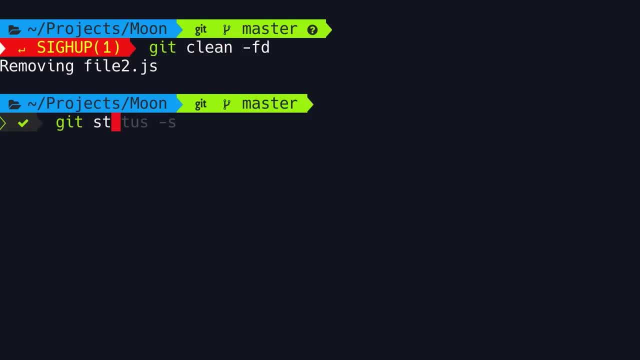 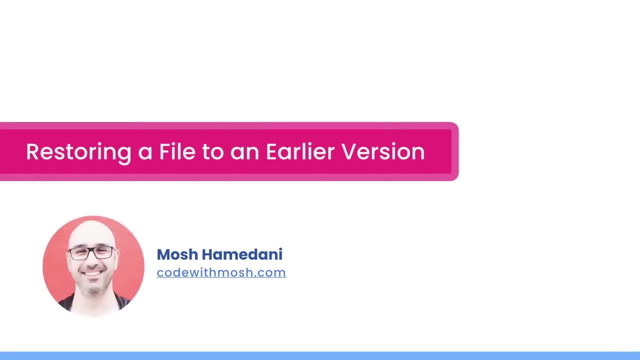 You also have dash d for removing whole directories. So quite often we type: git clean dash fd. Now let's run short status again: file2 is gone. So this is how we undo local changes. So now you know that. 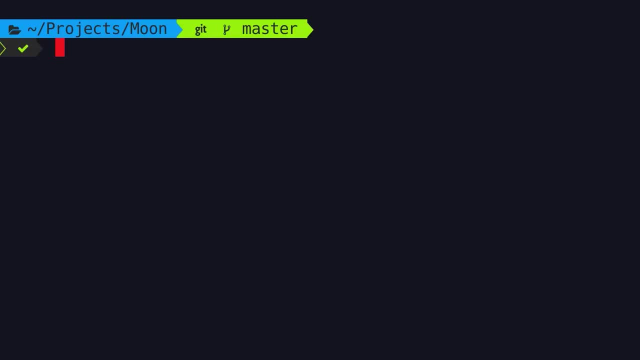 once git tracks a file, it stores every version of that file in its database, And that means if you screw things up, we can always restore a file or a directory to a previous version. So in this demo I'm going to delete a file. 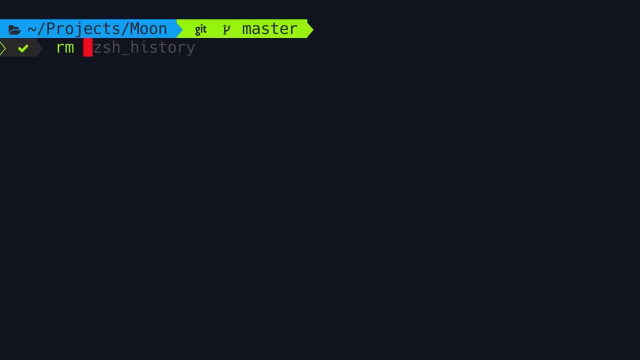 and then show you how to restore it. It's very easy. So we're going to delete file1.js now. I told you that if we use the rm command in Linux or Unix based systems, this will only remove the file from the working directory. 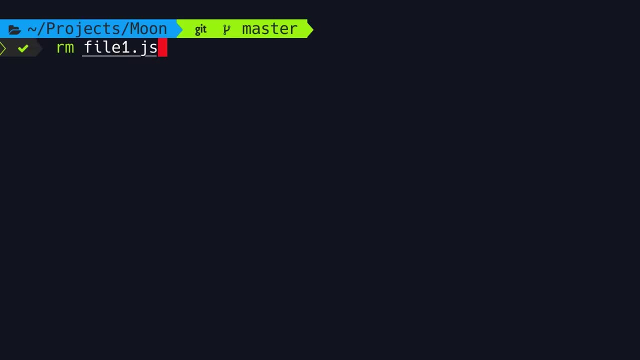 So then we'll have to stage the change or the deletion. A better way is to use the git rm command. This will remove the file from both the working directory as well as the staging area. Okay, So now let's get a short status. 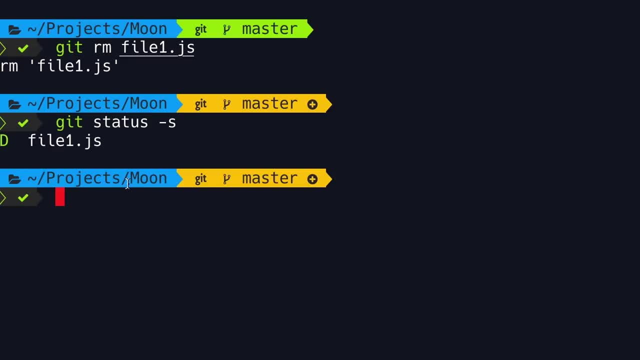 So in the staging area we have a deleted file. Now let's make a commit: delete file1.js. Alright, now let's say: shoot, we shouldn't have deleted this file. So what can we do here? Well, we have a few options. 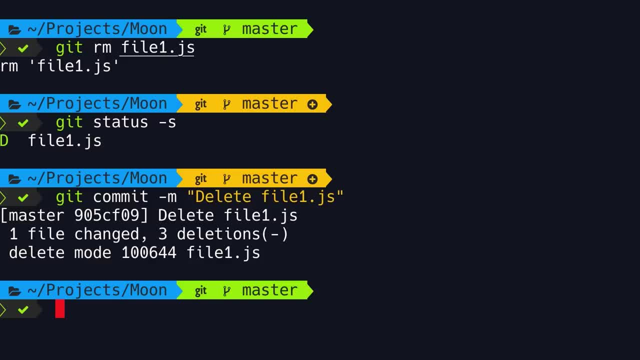 We can undo or revert the last commit. we're going to talk about that later in the course, but in this lesson I want to talk about restoring a file to a previous version, not undoing a commit. So let's look at our history. 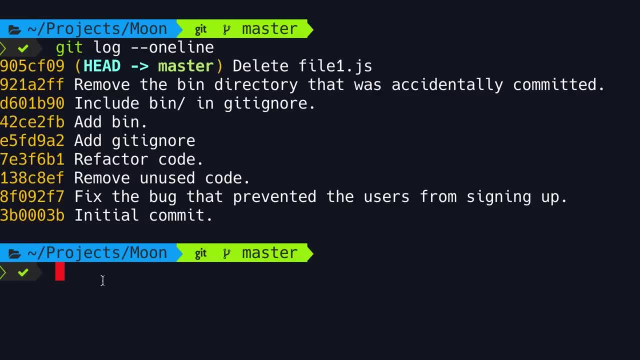 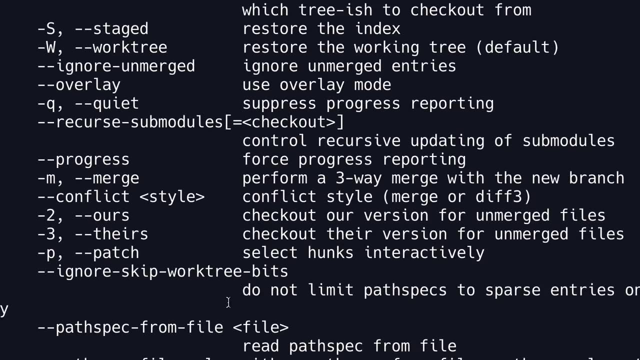 So here's our history. we want to restore file1 to the commit before the last commit, That is, this commit over here. So we type git restore. Now let's have a quick look at the documentation. The restore command takes three types.